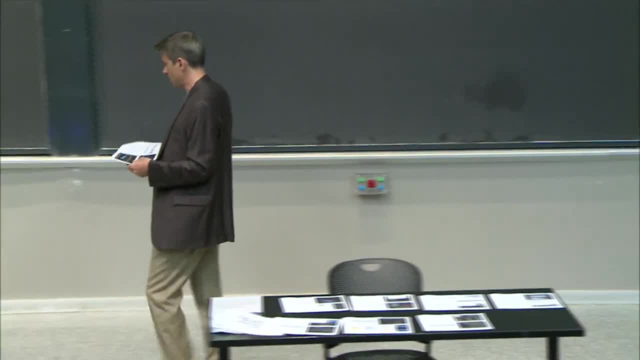 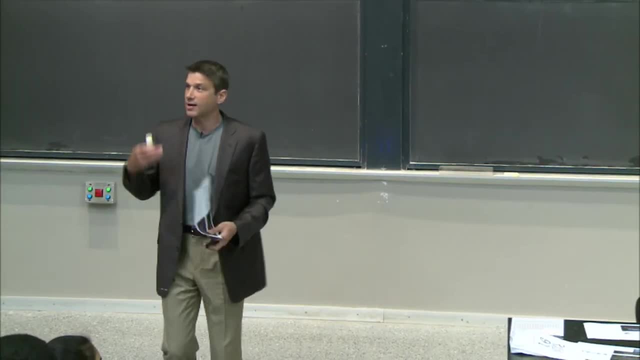 of thing. you might be asked on a quiz. I'm just saying So. that's good to know If I asked you this question because we counted on Friday, we learned how to count and we learned about the mole and Avogadro's number and how that gets us into and out of the atomic 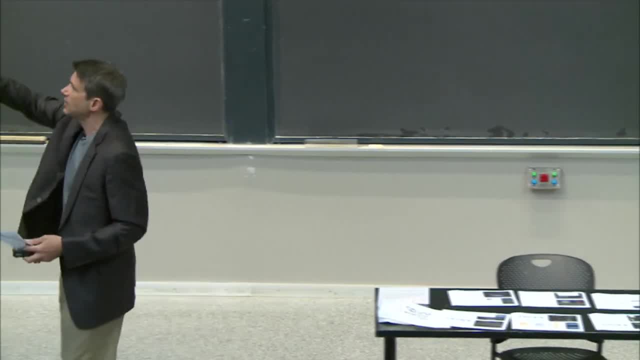 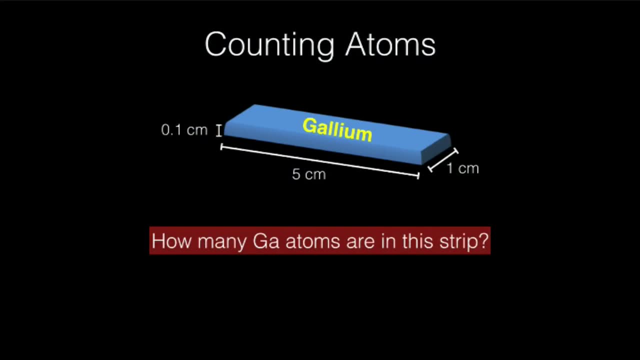 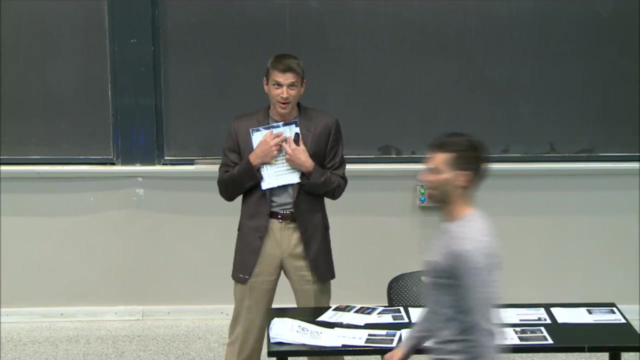 world, right? So if I say how many gallium atoms are in this strip of gallium, well, we can do that now, right? Because, well, how do you start? This is where you start And you're all taking it with you everywhere now. Remember, on Friday, we talked about how you 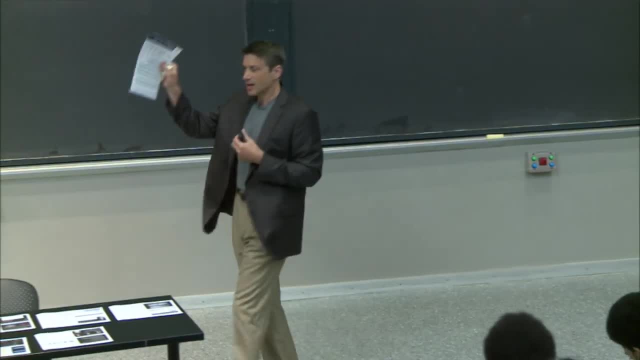 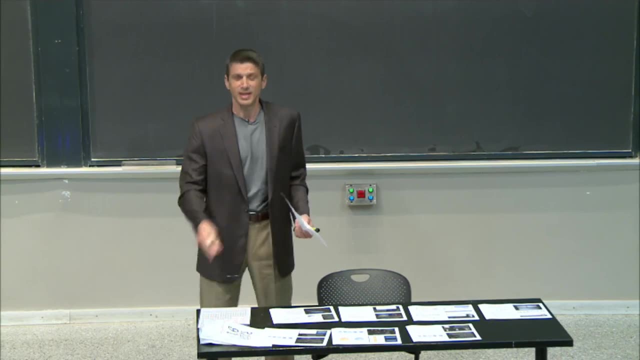 got to bring it with you everywhere And tweet about it and send me pictures and all that. I need the density, right, I need the density Density in the periodic table. Let's start with the density. So if I have the density of gallium, 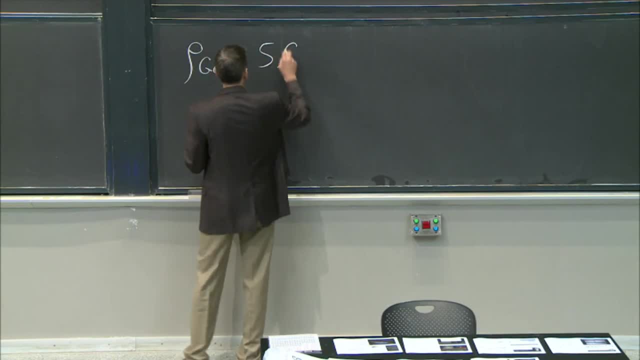 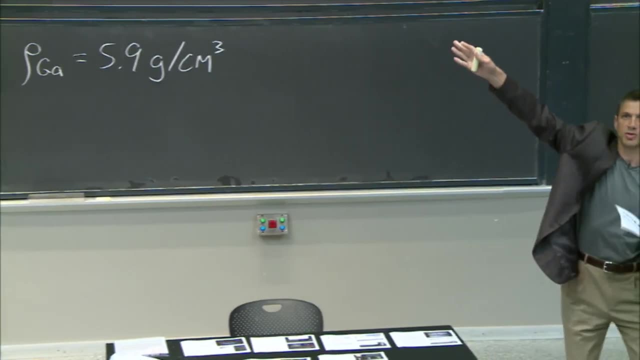 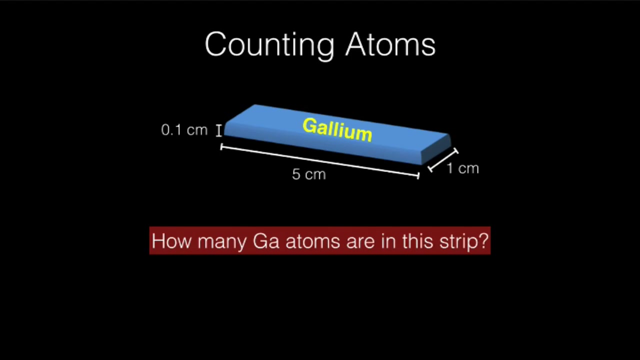 And I look that up as 5.9 grams per centimeter cubed. Okay, that's good. Well, you know, from the strip I can measure it with the super most accurate ruler in the world that you have now in your hands, from the goodie bag. And you see, those are the measurements And 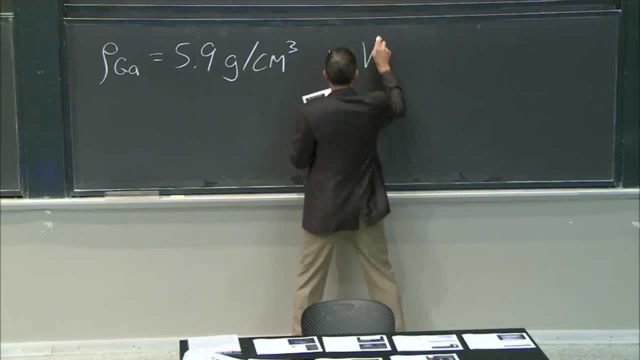 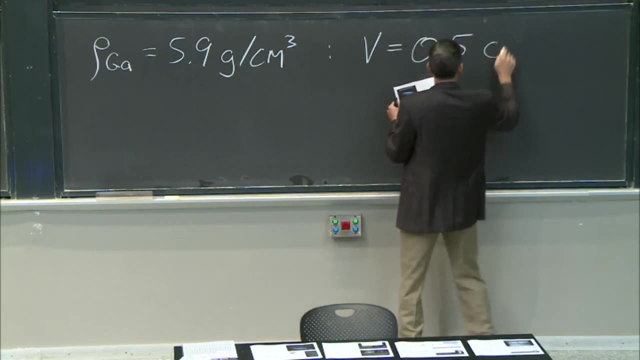 so if you measure it, you have a volume. Okay, it's those three numbers multiplied. I won't write it out. It's 2.5 centimeters cubed. And so now, with the density and the volume, I get that that. 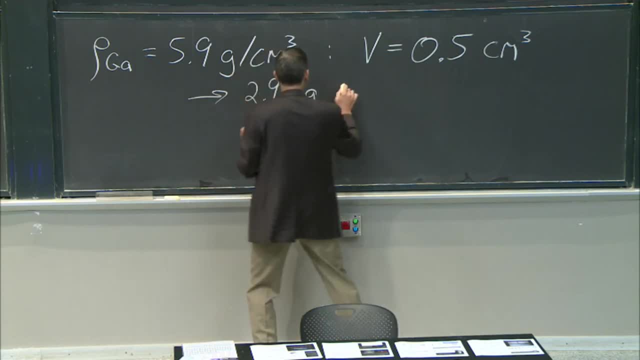 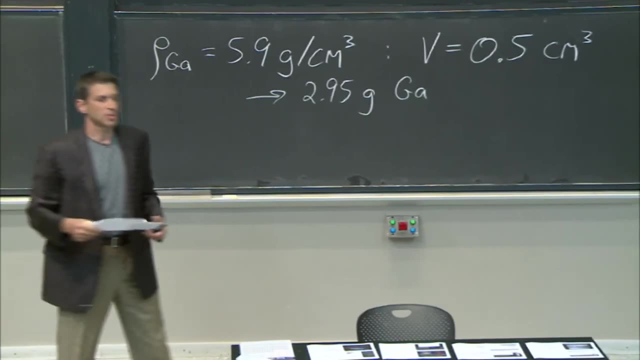 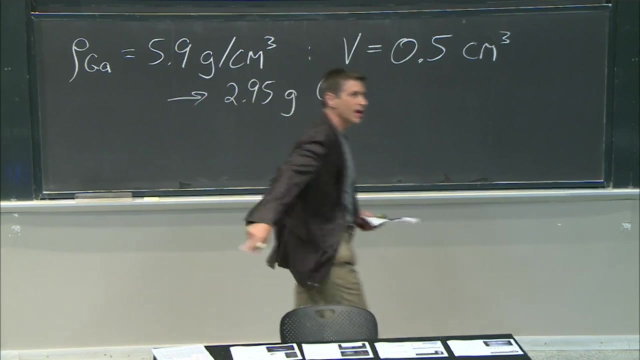 strip has 2.95 grams. Okay, now that sounds pretty good, It's promising, But I want the number of atoms. right, I want the number of atoms. And that's where again you go to here, Because in there is the grams per mole and also the atomic mass units, which, as we 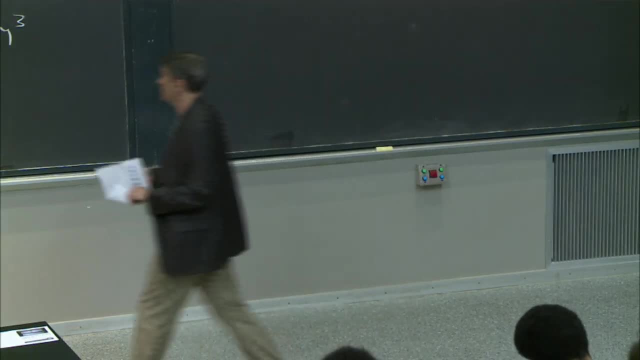 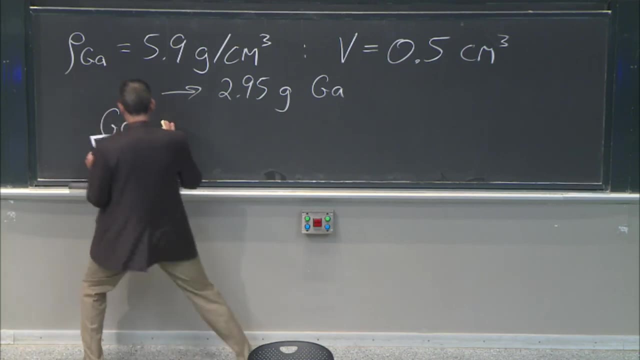 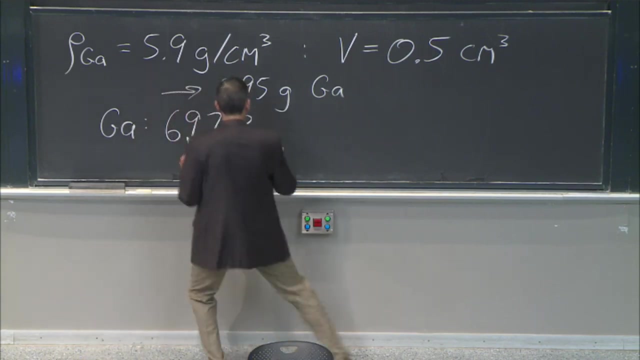 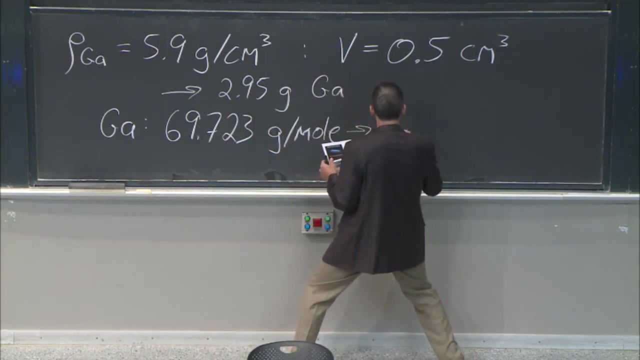 talked about Friday are the same thing, right, And so if I look that up, I have that. for gallium we have 69.723 grams per mole, right, And so that means that in 2.95 grams I have. 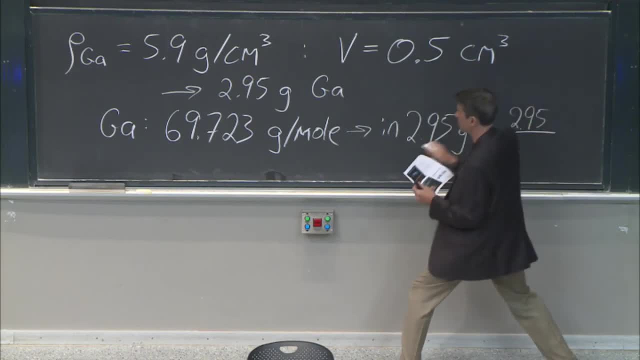 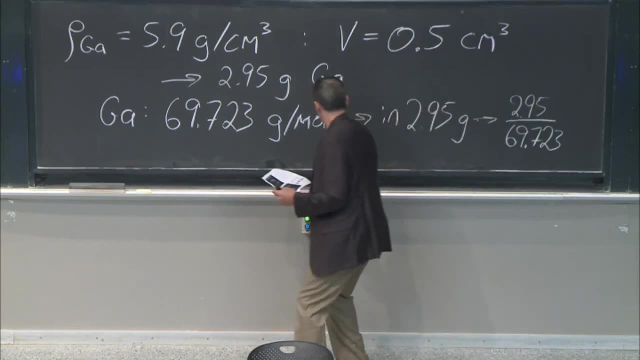 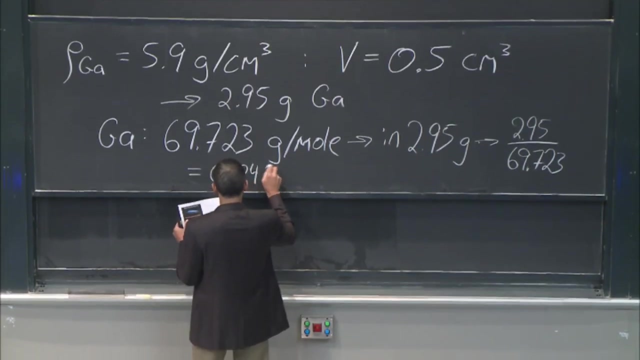 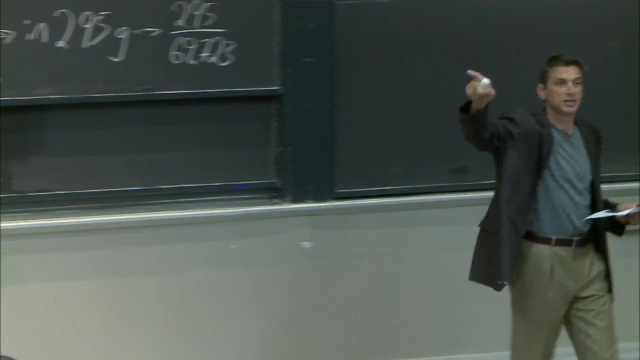 2.95 divided by that number, 69.723.. Let's raise this up a little- which equals 0.0423 moles. I still have not answered the question, because the question says how many atoms? right, But that's where N, sub a, or the mole, or this. 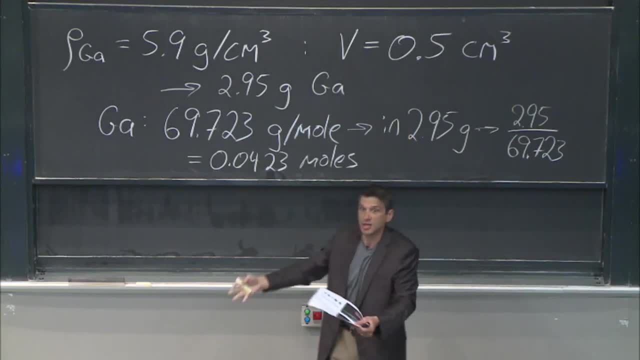 Okay, Okay. So this, this dozen, right, But it's not a dozen, it's a much bigger number. But this number, Avogadro's number, comes in. And so in that strip of gallium, no, in that strip. 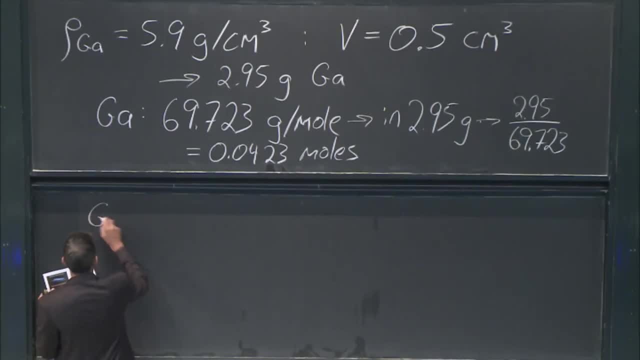 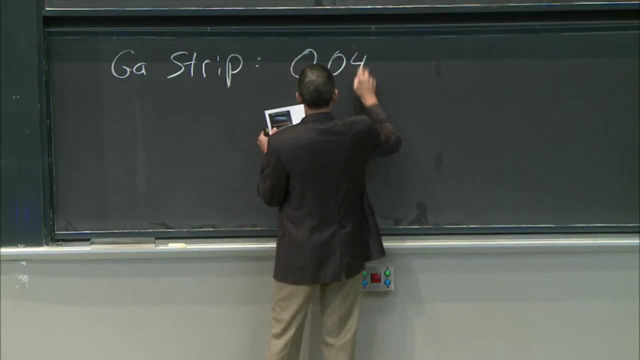 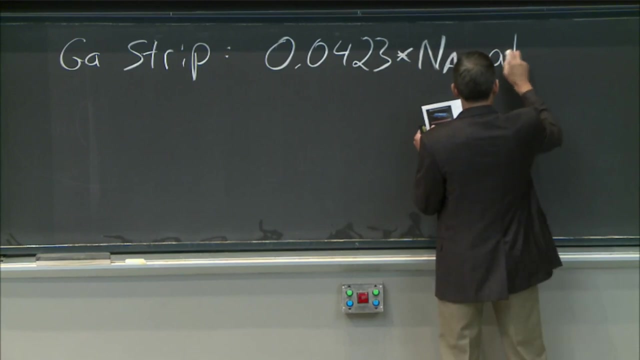 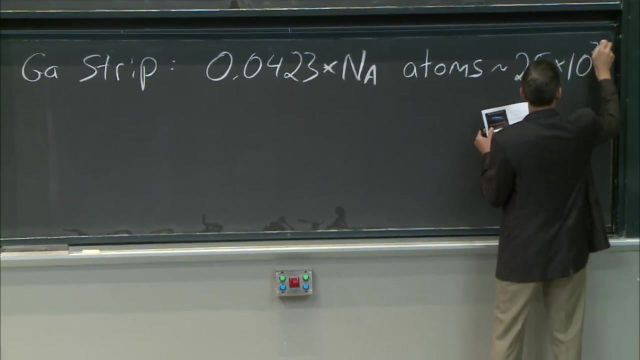 of gallium you've got. you know, in the GA strip you've got 0.0423 times N A atoms. Okay, Okay, Okay, That's something like you know, 2.5 times 10 to the 22nd atoms. That's a lot of atoms. 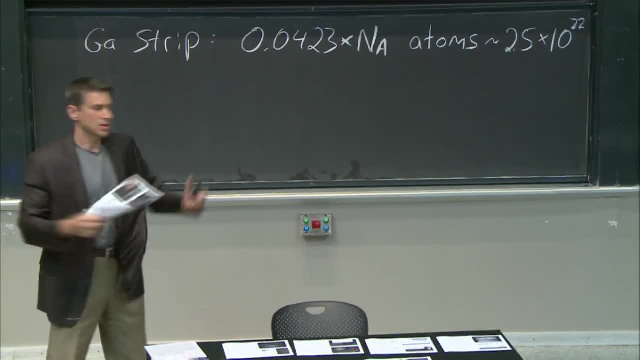 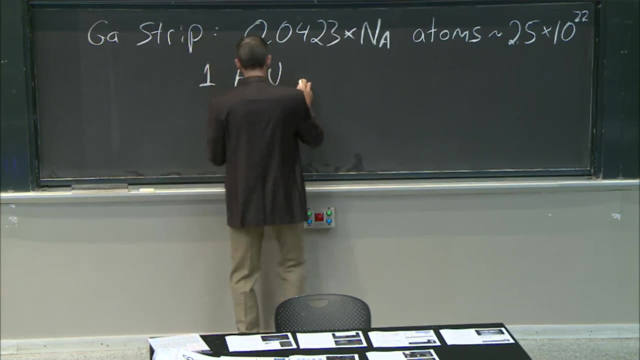 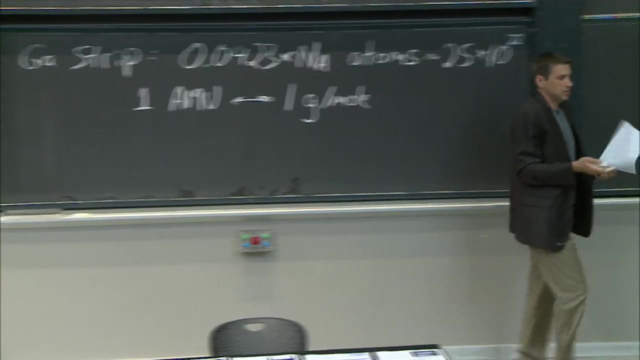 in that strip, but I was able to, but the. the secret is the the right. Remember, one atomic mass unit gets you back and forth between one gram per mole. And, by the way, the atomic mass unit is is nothing, It's just a mass unit. 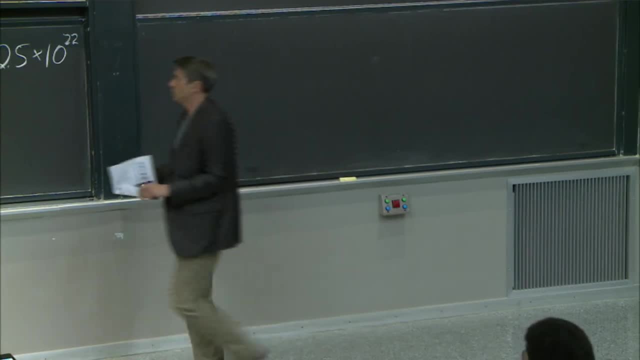 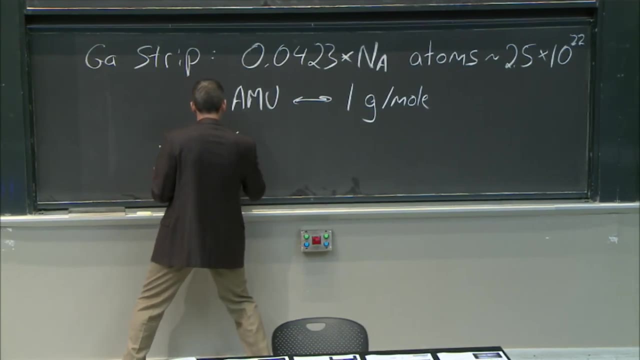 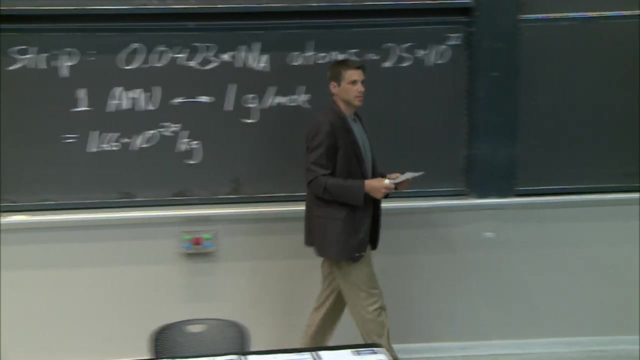 Okay, Okay, I mean 1 amu happens to be, by the way. oh, roughly 1.66 times 10 to the minus 27th kilograms. Oh, that works, because now you can multiply this by a whole mole and it's a gram. 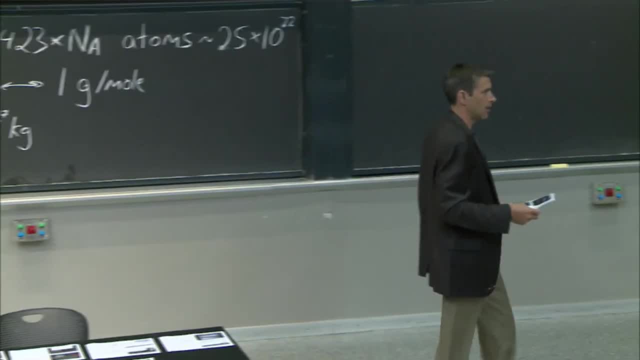 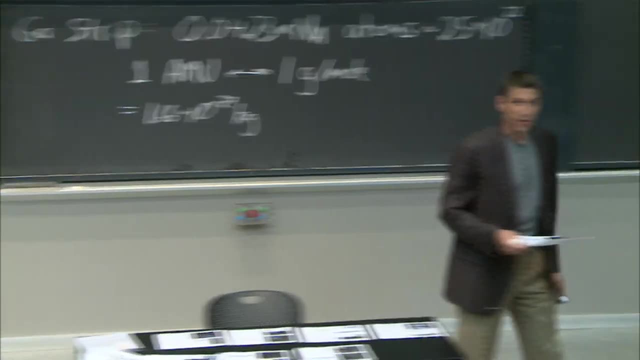 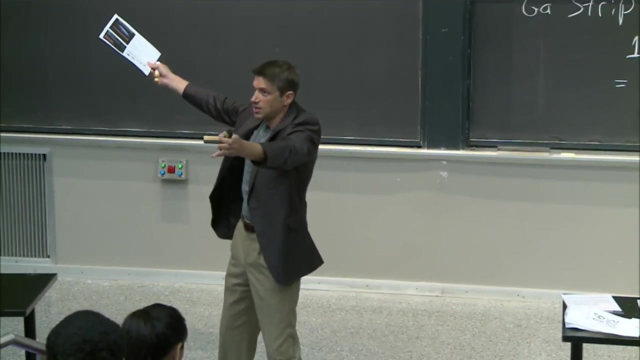 Back and forth. Okay, good Counting, Starting with counting, We're going to end with counting, But in between we're going to discover something beautiful. Because last week, okay, the thesis of this whole class, remember, is electronic structure holds the key to everything. 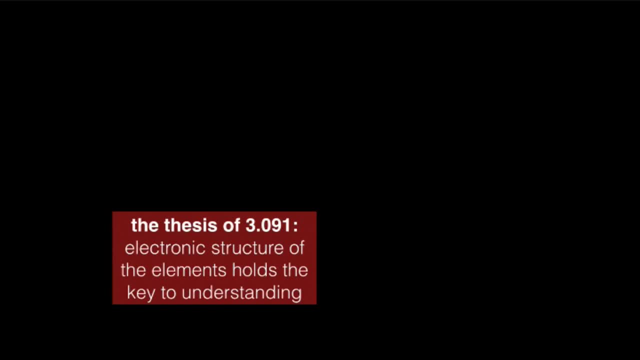 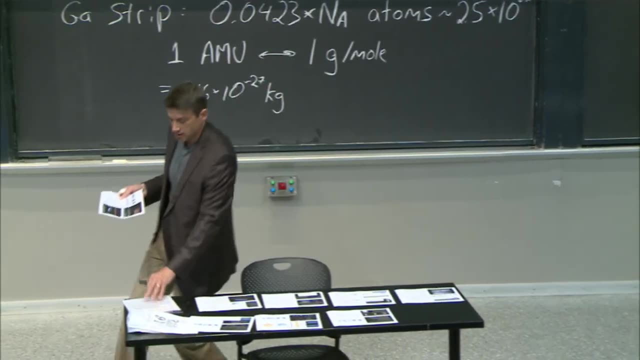 Everything in your life can be understood if you understood the electronic structure of the elements, Week 1, last week. well, we talked about this, We built it on Friday, We talked about elements, We did a few reactions, We talked about balancing. 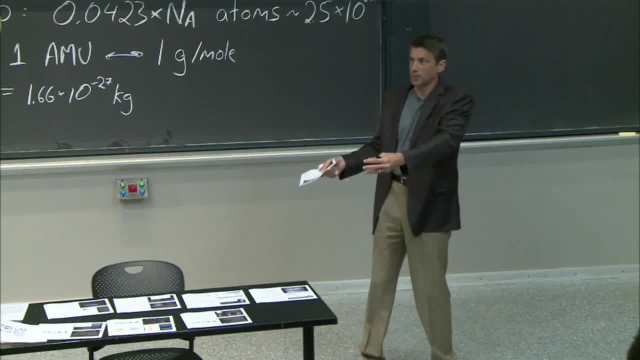 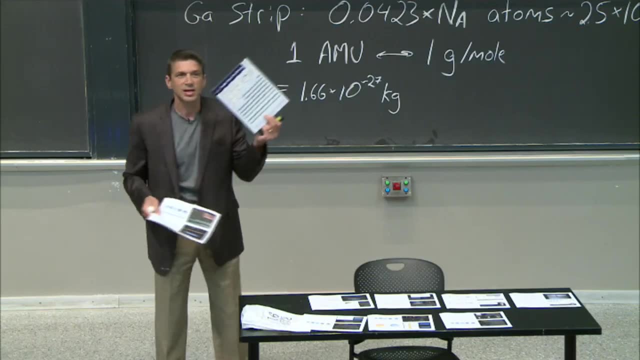 We made sure we have enough nitrogen. We had enough nitrogen to grow plants for 100 million more years. Limited reagents: This week we're going to answer the question: Why are these things different? We're switching gears Right. We know that there are these indivisible atoms now. 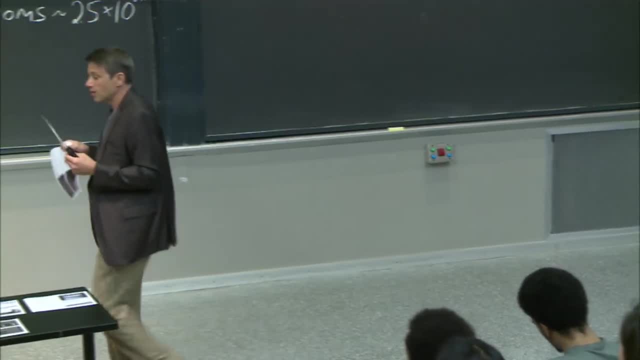 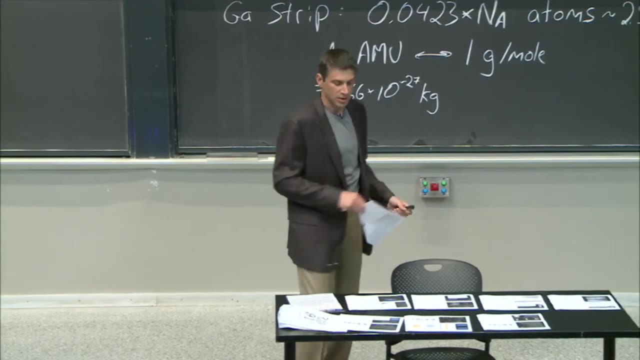 We built a whole table of them, Right Mendeleev, But now we want to know why they're different from one another. What causes that difference? And that starts with the discovery of the electron. And really this is such So. 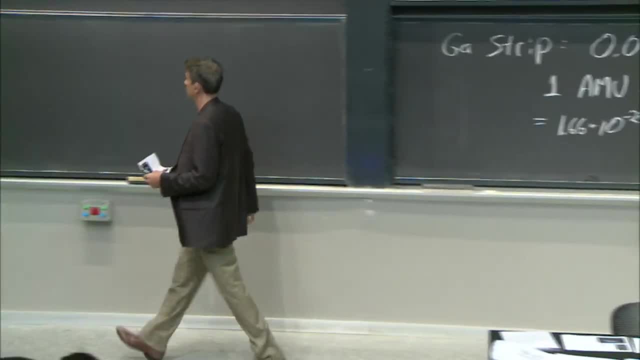 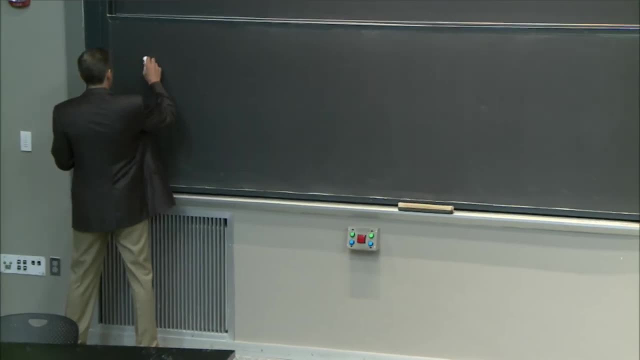 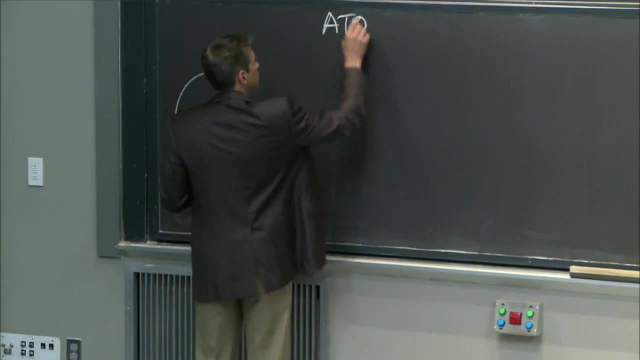 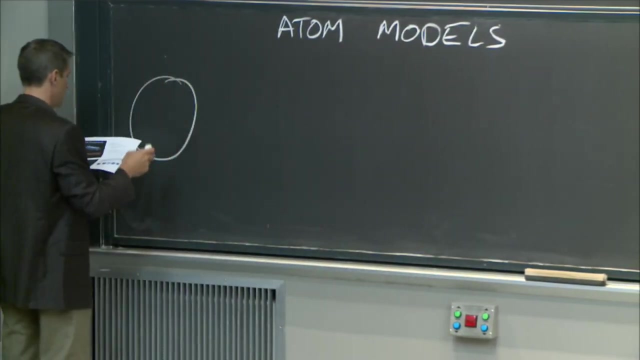 We started. let's write this here. We'll have this board. This is such a great story. This is a detective story that starts with an atom looking. So these are like atom models. OK, so back in, oh, let's say 18.. 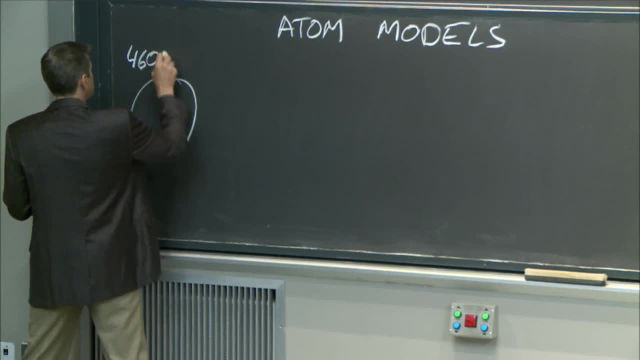 OK, 460.. If it's Democritus, it's 460.. And then, remember, we sort of went all the way to Dalton who, in 1803, he said, yep, Democritus, we're going with that. 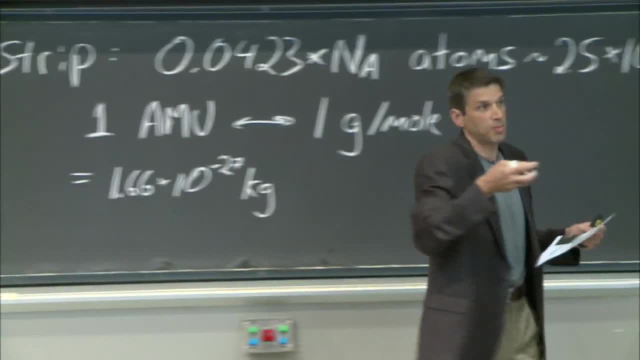 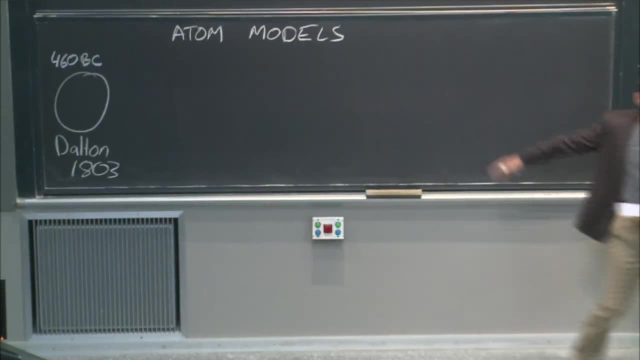 We're going with that. And oh, there are these indivisible things called atoms. So that was 1803.. But we need to understand them in order to explain this. We need to understand. So this is a detective story. It's a detective. 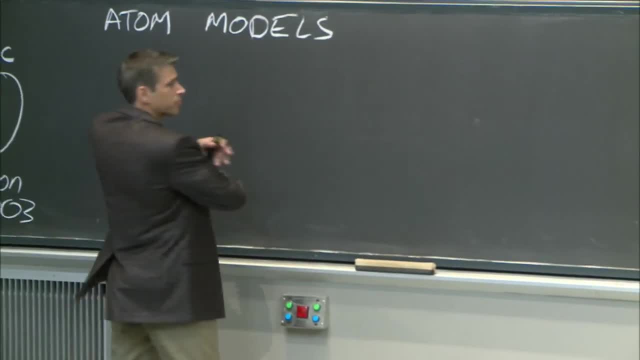 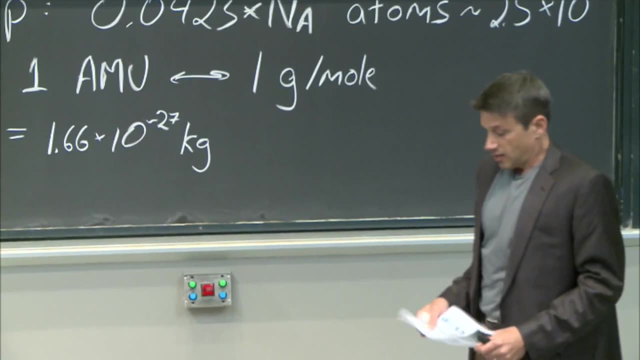 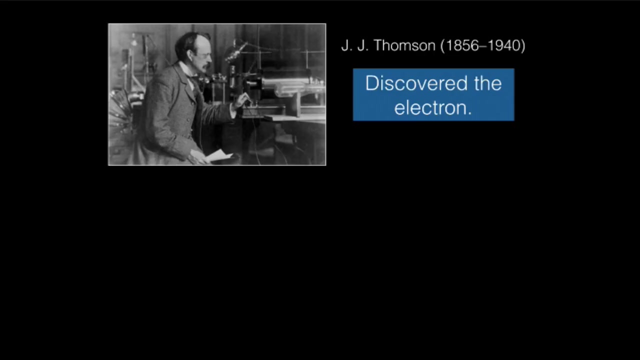 It's one of the greatest ones ever, ever, ever played out in science. It led to nothing less than the understanding of all of nature. OK, now, how did it start? Well, it started with JJ Thompson. Now JJ Thompson, by the way. he won the Nobel Prize for this discovery. 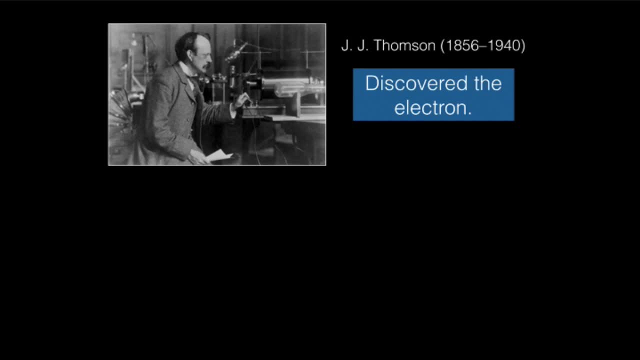 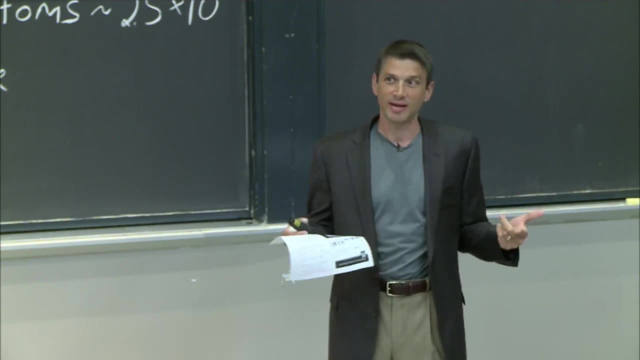 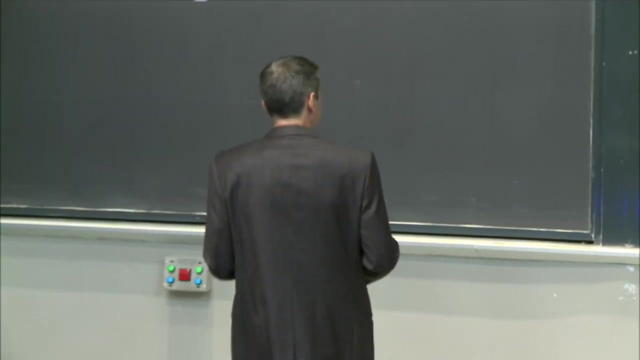 He's credited with discovering the electron. Also, seven of his students won the Nobel Prize. That's cool, And I remind my graduate students of that all the time, without trying to put any pressure on them. How did he do it? Well, you see, he had these things. 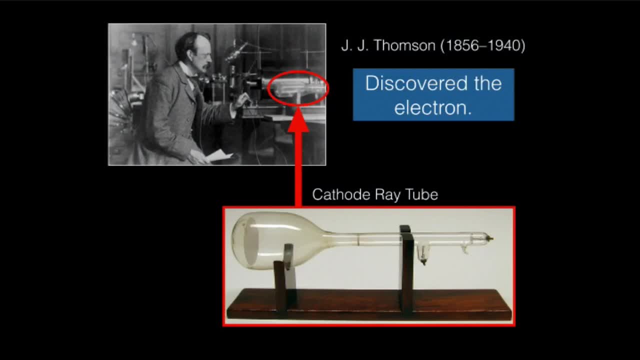 There's his lab. There's Thompson, There's his lab, And these things were around. They're called cathode ray tubes. Cathode ray tubes. What do they do? All right, What do they do? Well, your grandparents would know something about them. 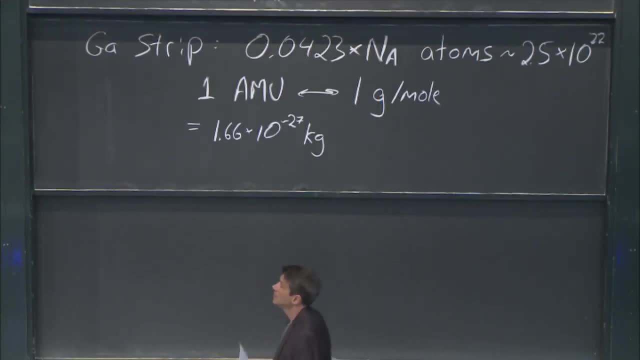 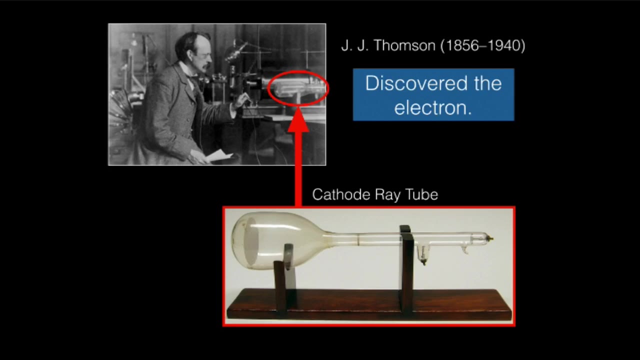 I'll talk about that in a few minutes, But Thompson. Thompson was interested in seeing what he saw on this thing here, And that's the photographic plate. So what we're going to do is I'm just going to draw the cathode ray tube. 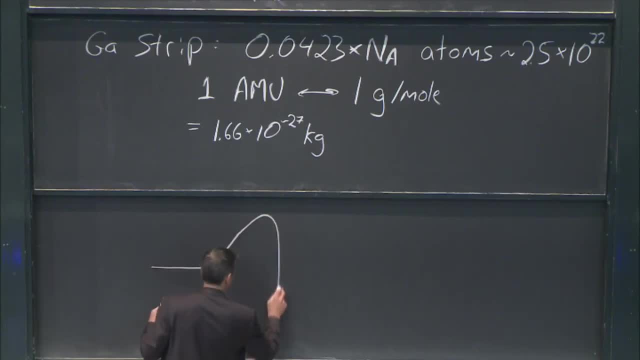 I'm going to draw it as best I can here. So there's a cathode ray tube And over here we've got a cathode, And over here we've got an anode, So this would be a cathode. 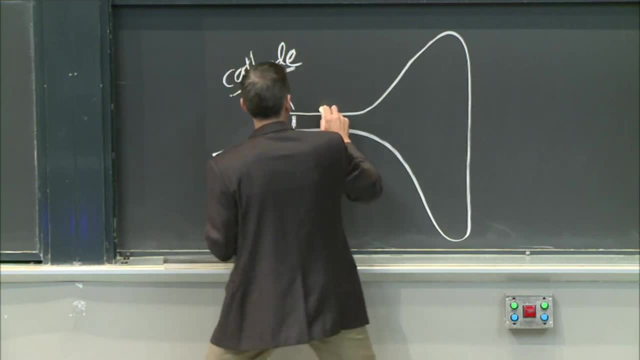 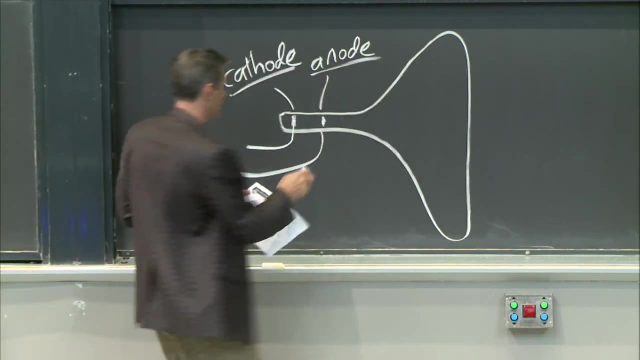 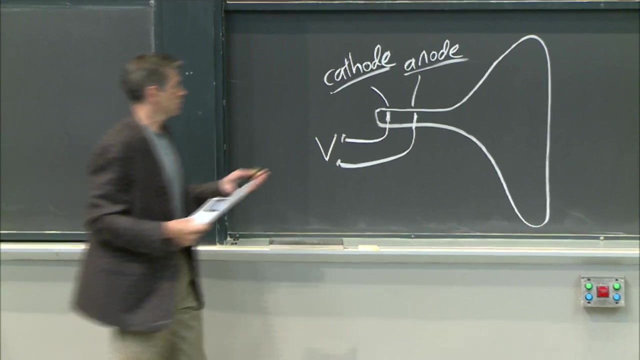 And this here is an anode. OK, Good, Now that means that if I hook those, those are two pieces of metal, Two pieces of metal. And if I hook them up to a voltage supply Right, Well then I can get charge on them. 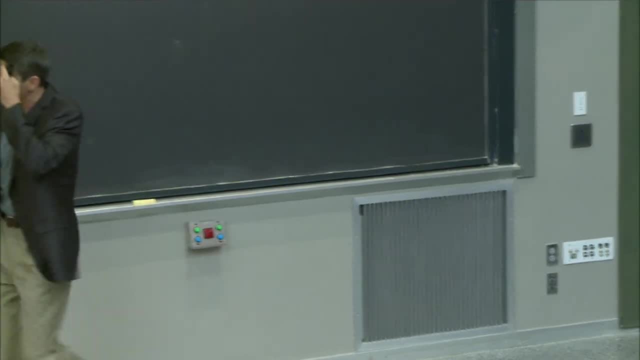 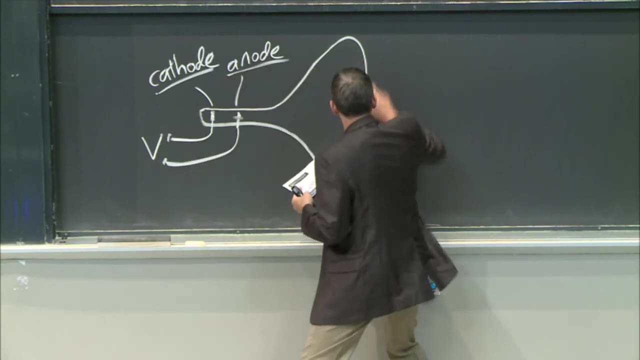 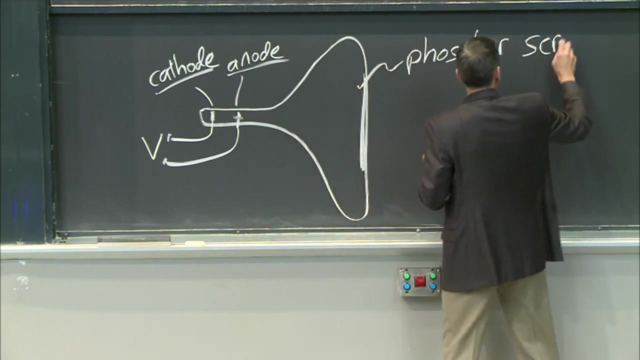 We know that already. But what they didn't understand is what happened next. You see, because if you crank the voltage up really high And you put a phosphor screen here- So this was a phosphor screen- And if you crank the voltage up high enough- and this is what Thompson did- 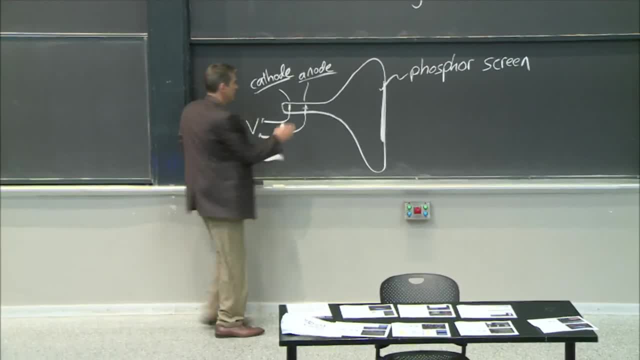 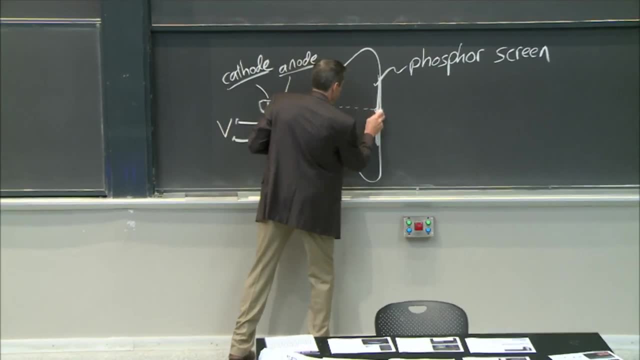 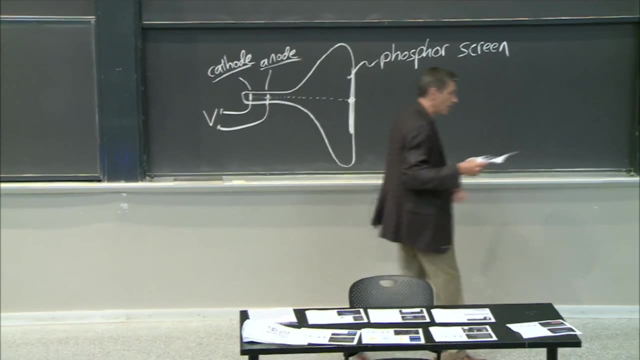 You pump the gas out of it, Right, So you get it, So there's not too much stuff in there. Then what happens is something shot across and lit up the screen, Something What They really didn't know. And when you don't know, you experiment and you apply the scientific method. 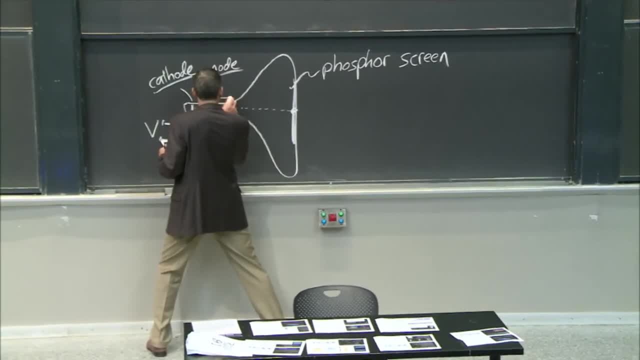 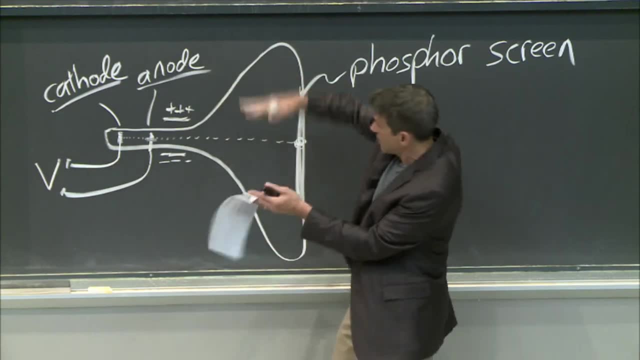 And one of the things that Thompson did is he said: well, what if I put some charge plates here like this and this? So I have a, I have a set. So I just said this is going to have charge. that flies off. We know that because we kind of know what happens. 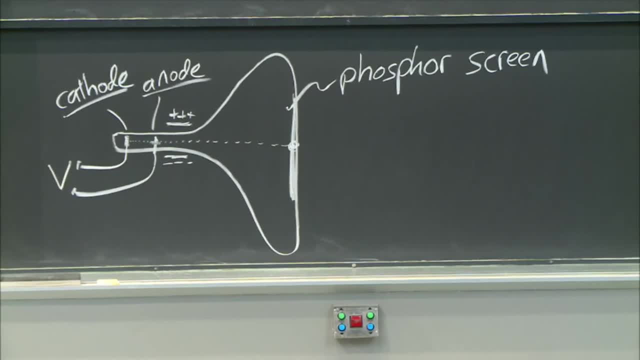 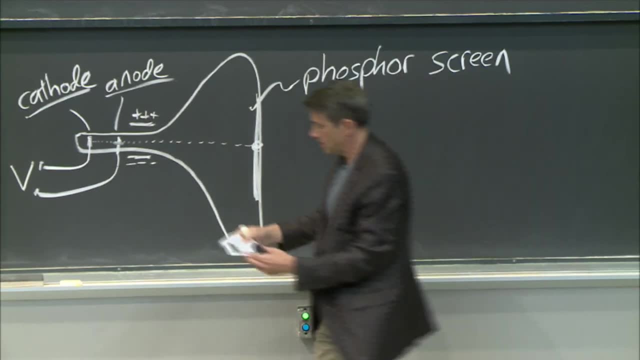 But he didn't know what was happening. He's just cranking the voltage up and all of a sudden the screen lights up. So he's like, well, let me put some charge, Play It's here and see what happens. And what happened there is. it went like this: 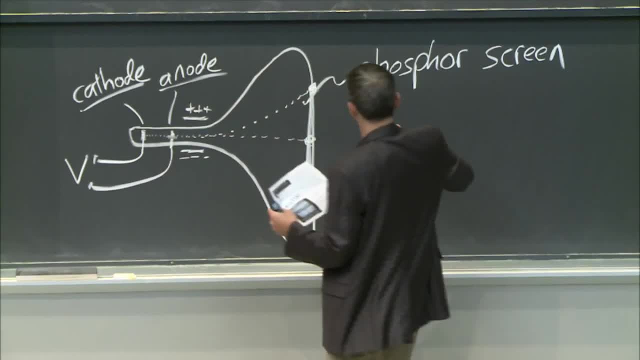 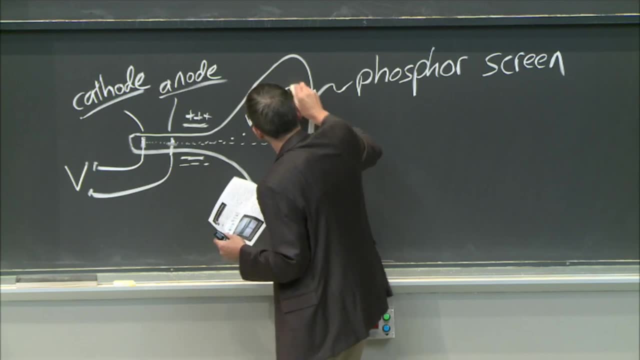 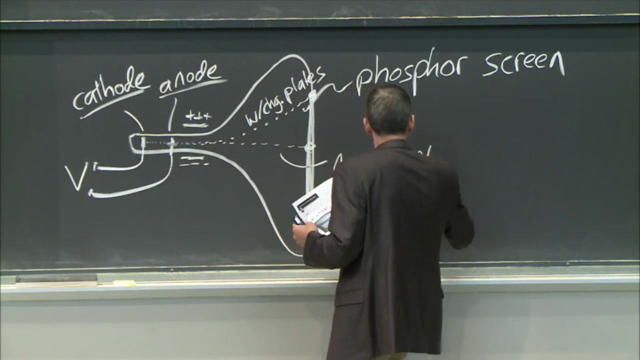 Right, And it made. it struck the phosphor screen there and it glowed there. So that's with charge, with charge plates, Right? No charge plates, just to be perfectly clear. Right, And he could play with this night, and people do play with this. 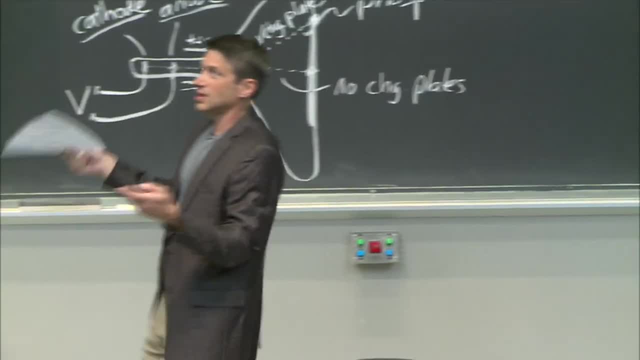 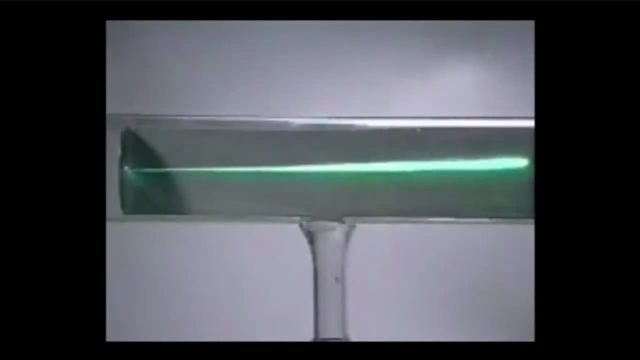 To my great surprise, if you go on to the Internet and you Google this, you find people make these and play with them, And that's a magnet. This is what it looks like. Right, There's that. We know what this was. 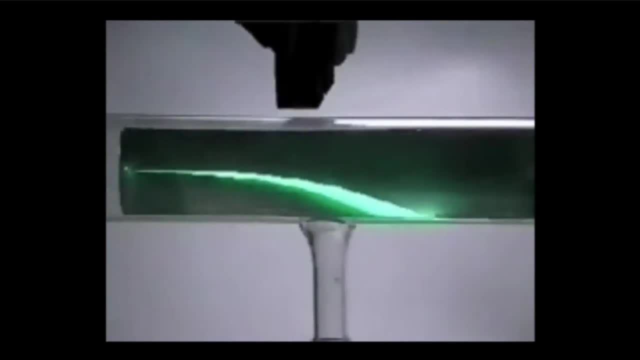 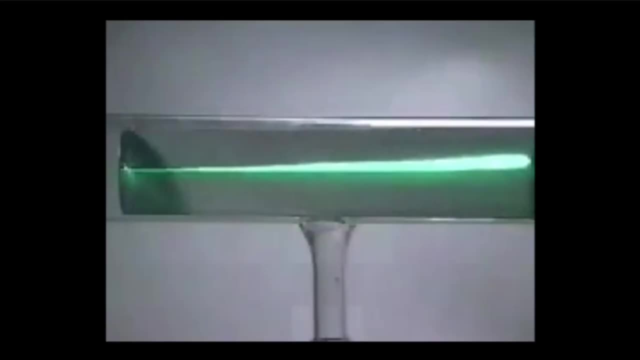 Right, So so that's a magnet And this, this person, is just turning over, whether you know which part of the magnet, where the magnetic field is oriented, And you can see you can really mess with this. What could it be? It's responding to an external field. 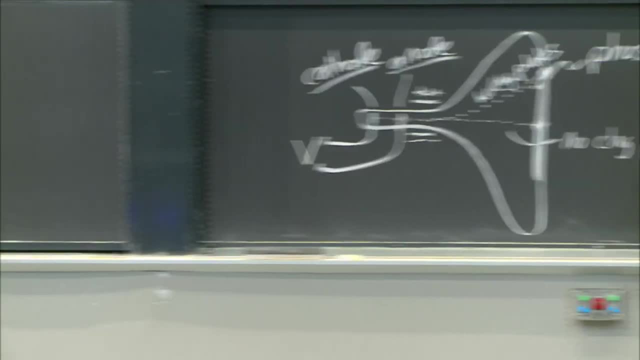 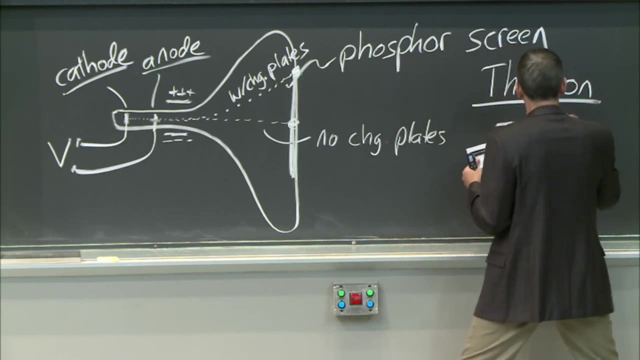 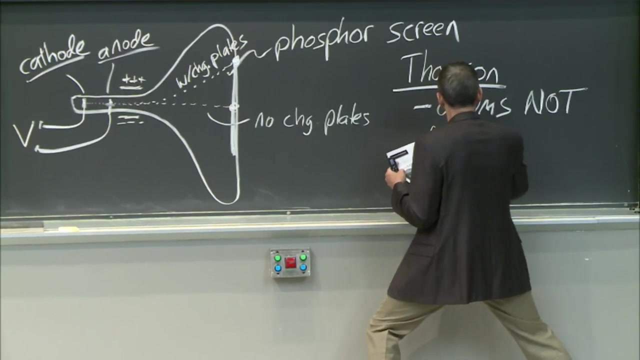 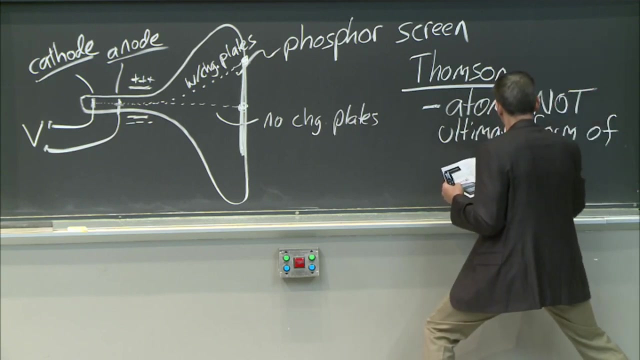 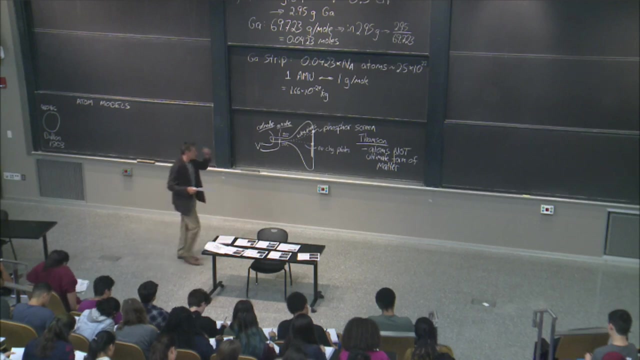 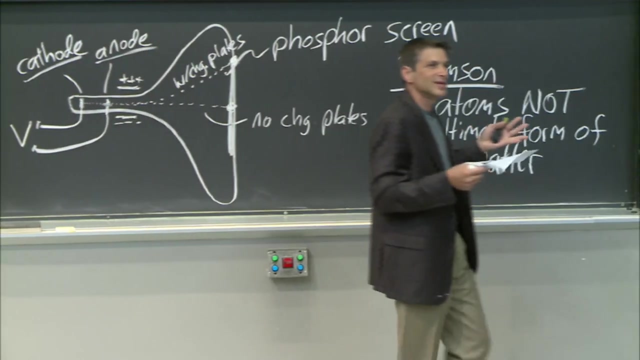 It's responding to an external field. So we know right away. this tells us that atoms are not the ultimate form of matter. That was a big deal, because you know the atoms here were neutral, they didn't respond. So this must be something else that's flying off and responding. that I can see visually on this photographic plate. 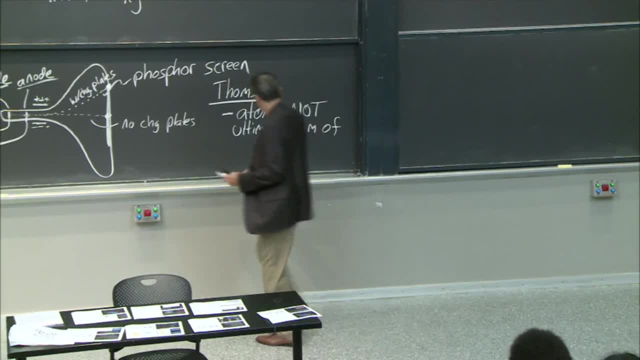 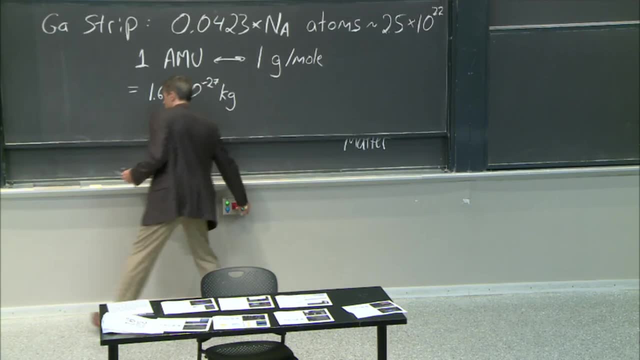 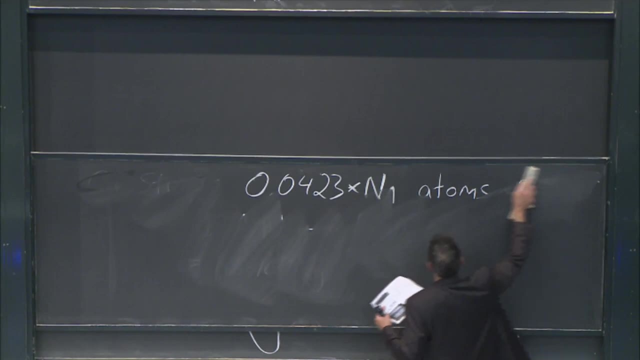 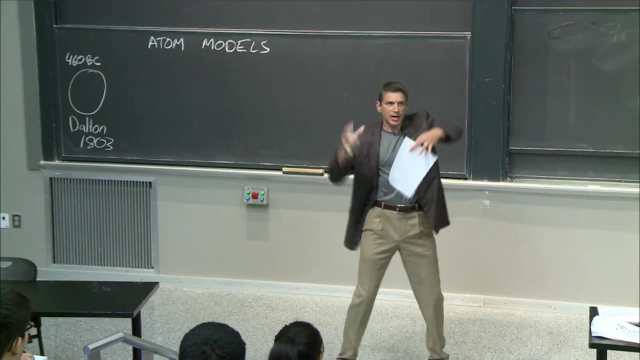 It must be something else. Well, he was also. Thompson was going down here. I'm going to use this, So it's right next to it. He was not able to measure the mass of these things, but he was able, using a combination of magnetic and electric fields and a little bit of Maxwell, some E&M. 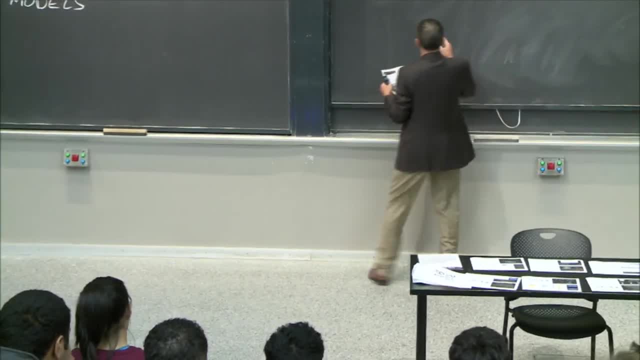 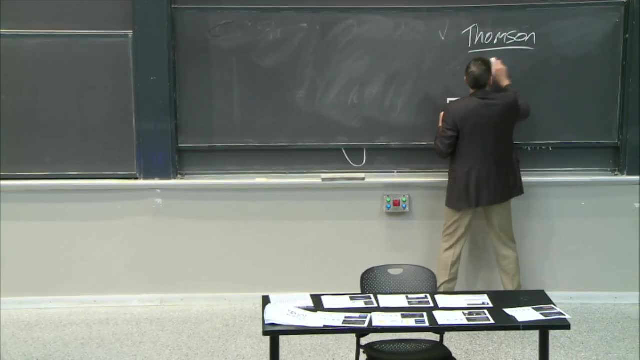 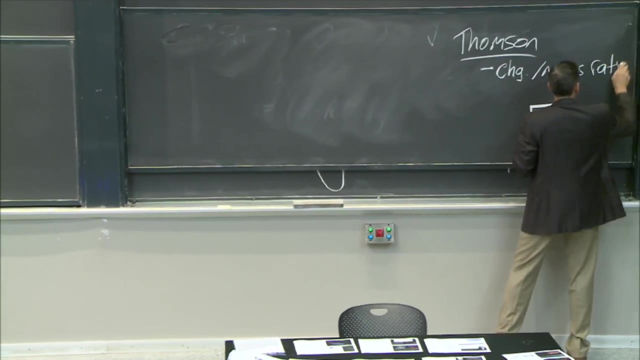 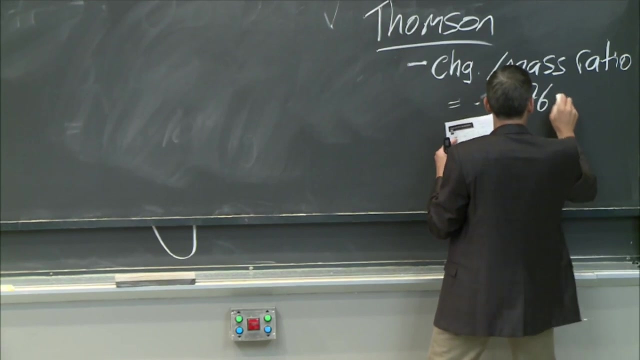 He was able to deduce the charge to mass ratio, So this falls over here. I'll put it here from from Thompson. So he was able to get the charge. It's a mass ratio and he was able to measure that at minus one point seven, six times ten to the eleventh coulombs per kilogram. 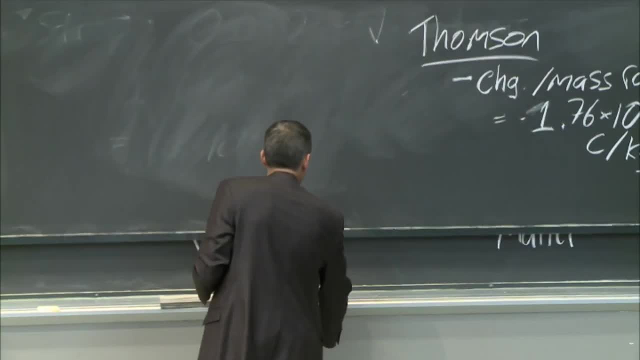 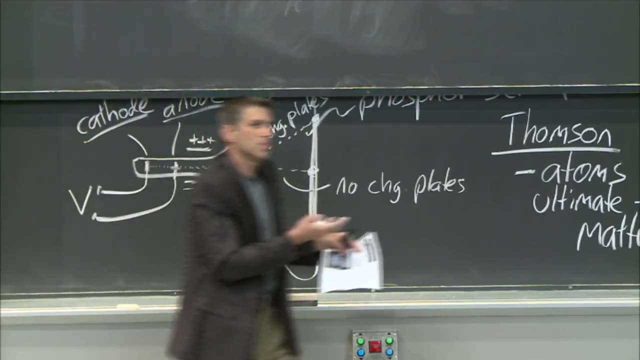 Now he knew it was negatively charged because of this right, He put the plates on and it wanted to avoid the negative plate. So we knew they knew. they knew their E&M at the time. They knew that The negative charges would repel, so he knew that it was negative charge. 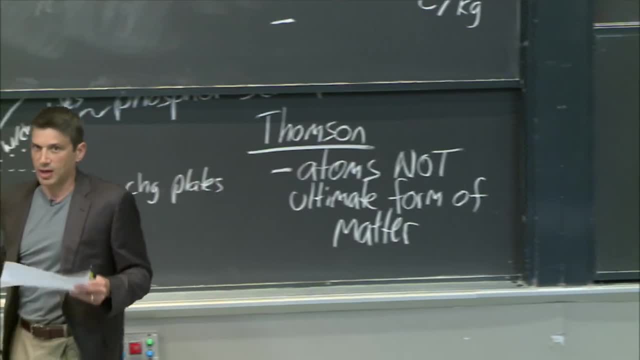 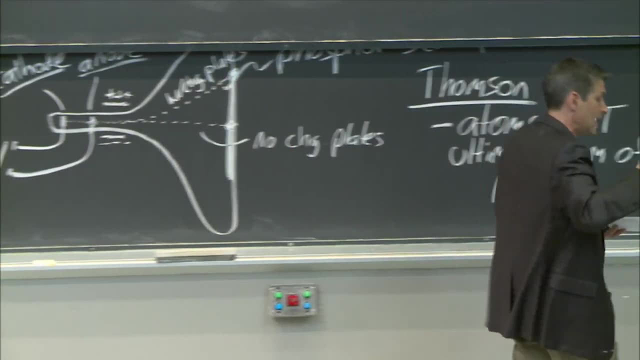 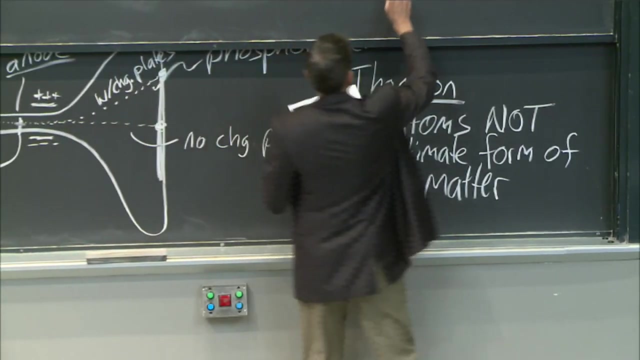 Now the last thing. oh, is this one important for chemistry? He would swap in different materials, different metals, for the cathode and for the cathode especially, And the results were the same. The results were the same, whole, whole, independent in dependent. 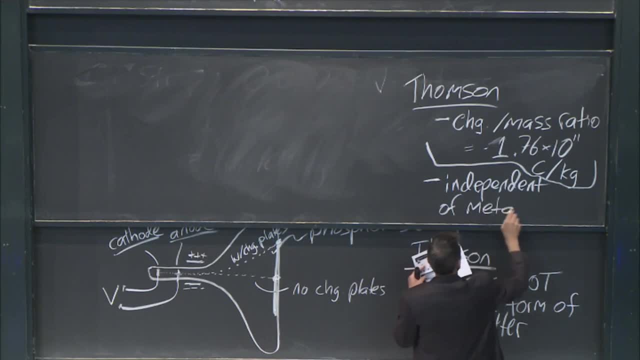 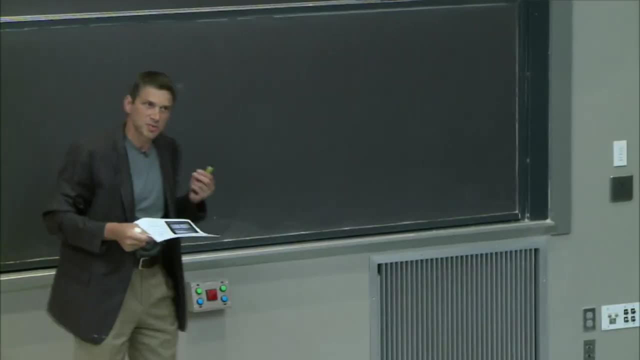 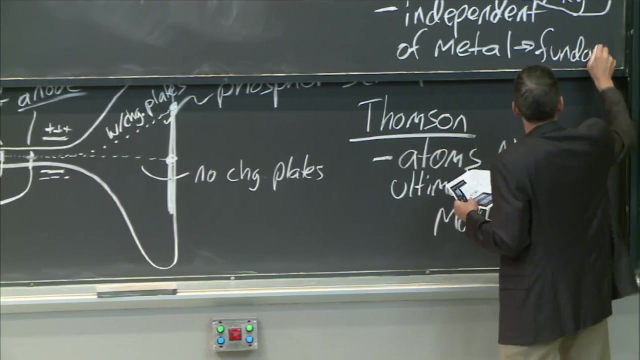 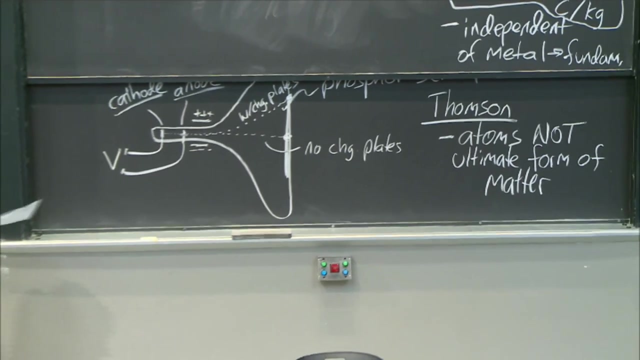 Of metal, independent of the metal. that meant this thing that he was observing for the first time was fundamental. There's something fundamental about it: Fundamental, fundamental, fundamental. oh, this was a really big deal. This was a really big deal. 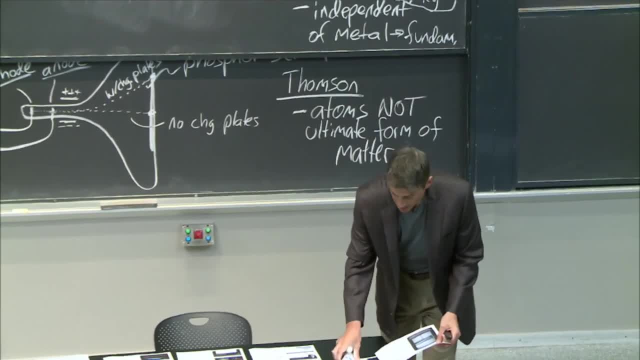 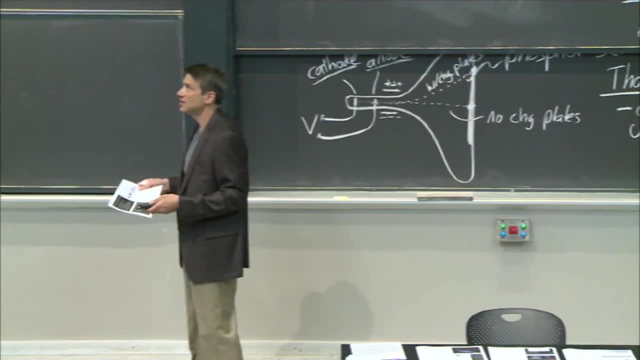 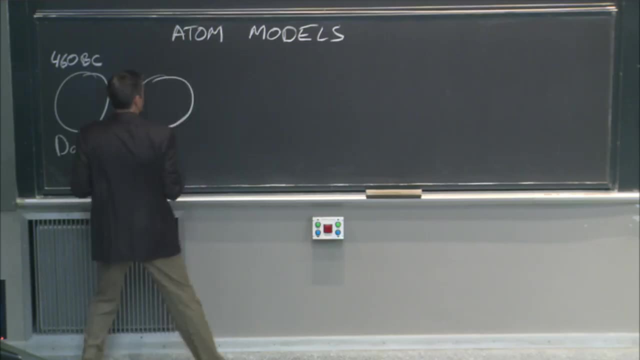 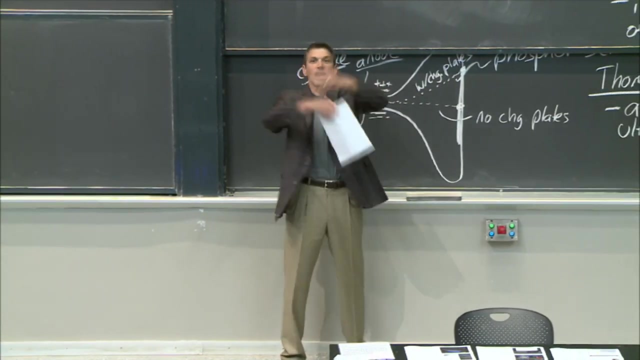 And it, and it, It. It really opened up the idea that the atom had something else in it. Now, Thompson, see, Thompson knew right, he knew that the atom was neutral, like I said. So you got these charge things coming off of these atoms which are neutral. 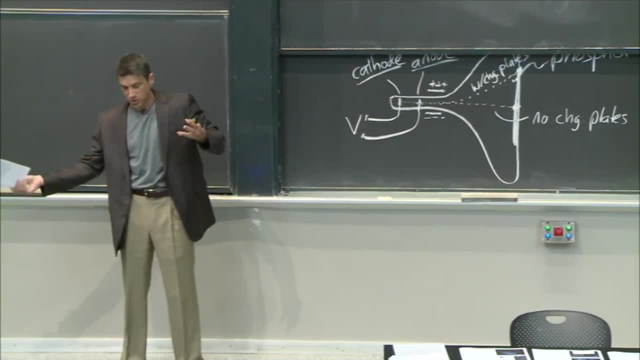 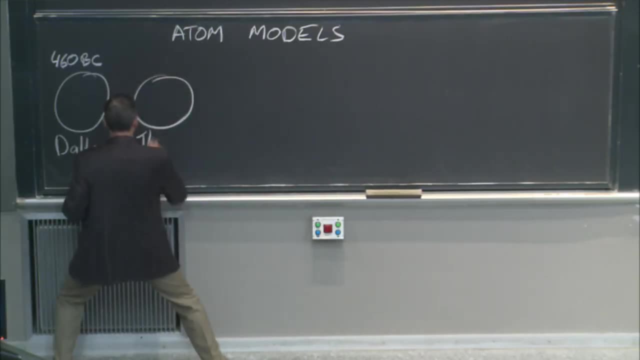 That means that it must consist of these charged particles, But if it's neutral, it's got to have the other charge of particle in it as well, And so the detective story goes on. So this would be Thompson around 18, oh, things really picked up 1807.. 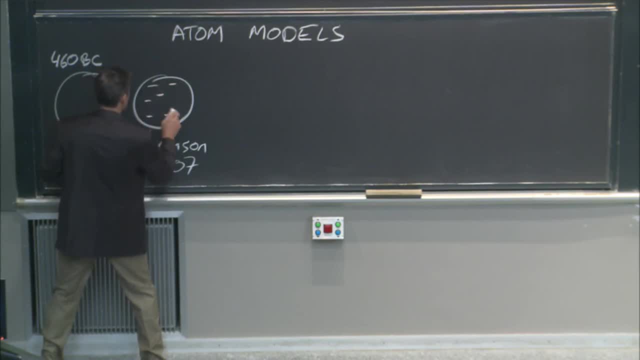 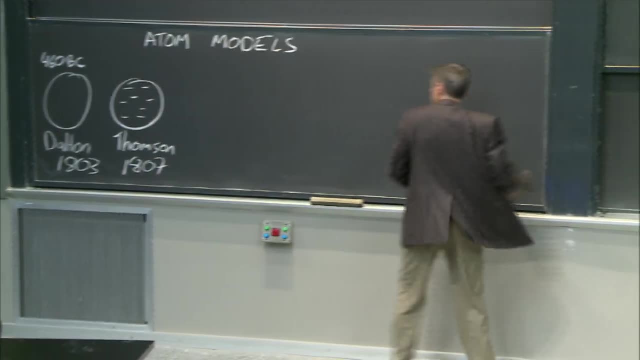 And he said: well, OK, these electrons must be inside of the atom. That's how I'm liberating them: Crank up the voltage, and and they must be in there. But so must positive charges. so must positive charges. OK, and that was Thompson's model. 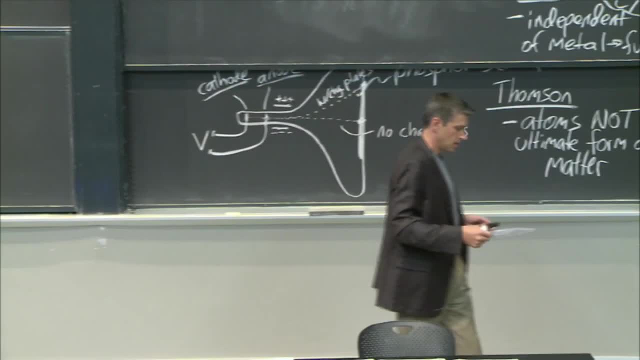 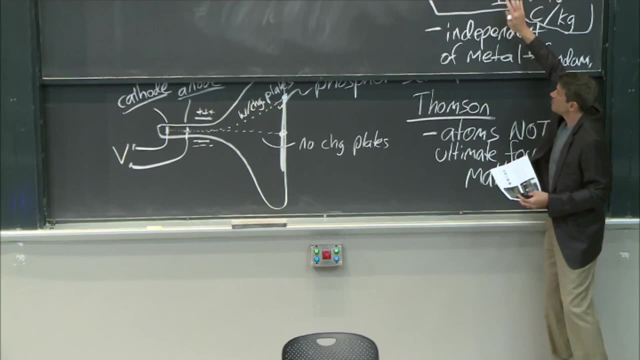 So at that time, And you could, you could, you could really have this picture of stuff inside the atom. Now, like I said, he still he couldn't measure. They didn't have a scale good enough to measure the mass of the electron. 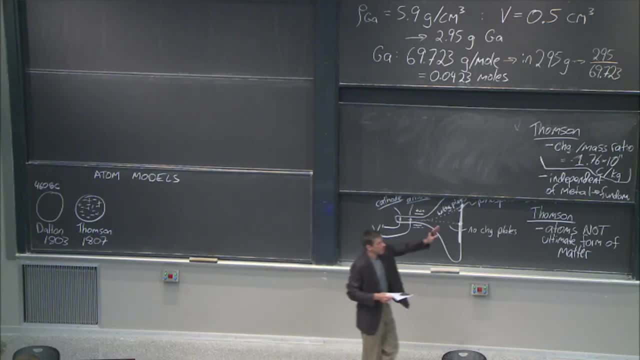 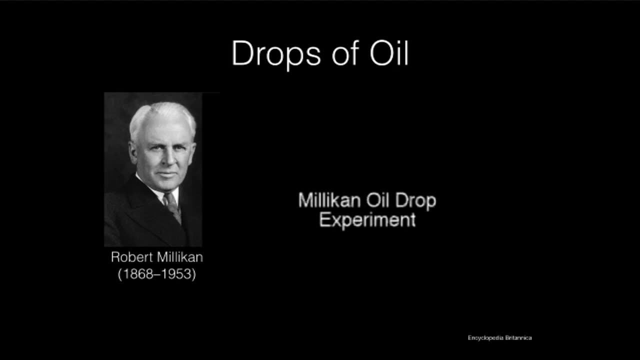 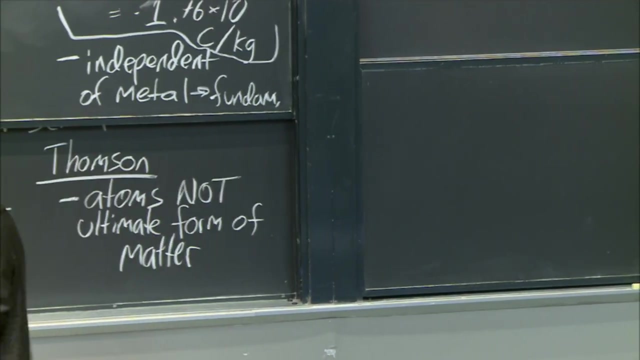 He couldn't get it out Right, But it was. it was Millikan and his very famous experiments called the oil drop experiments that gave us the actual charge. And then, from this ratio, We can get the mass of this, this mystery thing that was coming out of atoms. 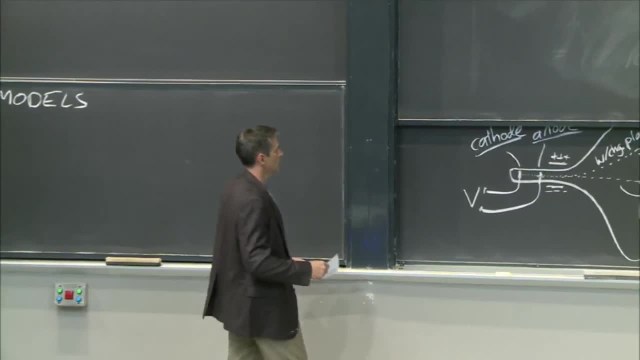 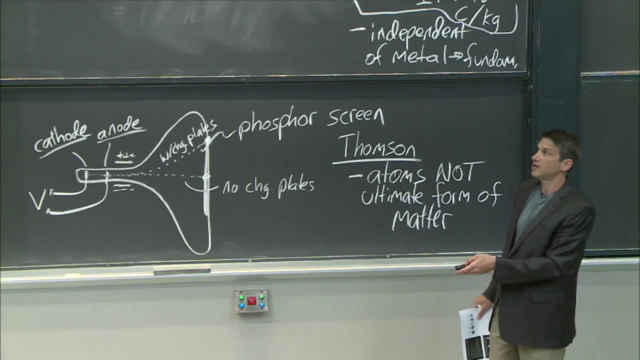 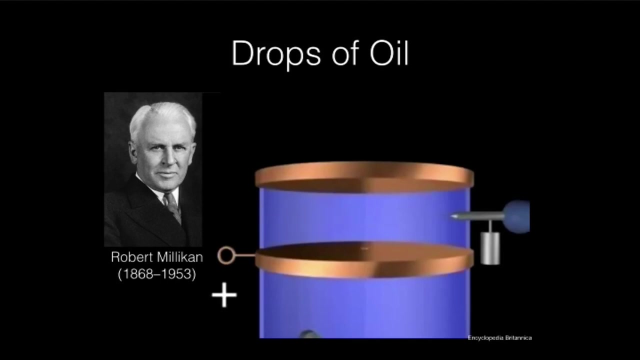 OK, And instead of drawing, trying to draw the Millikan experiment, I found a wonderful short, like one ish minute video which I'll play because it shows how the Millikan experiment worked. It's really cool. Oh, working at the University of Chicago succeeded in measuring the charge on the electron. 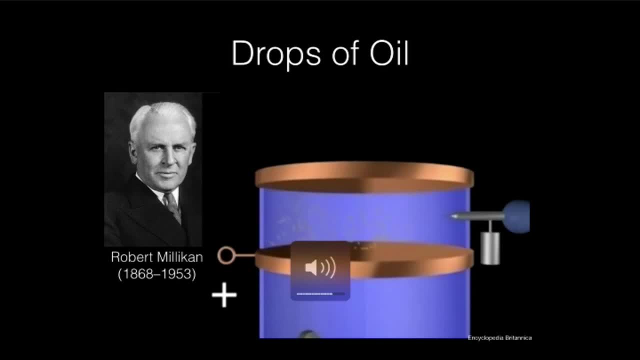 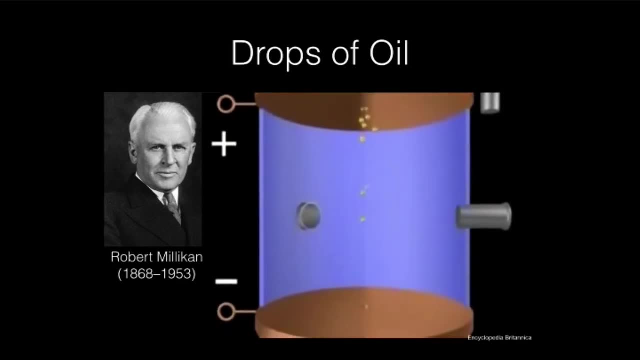 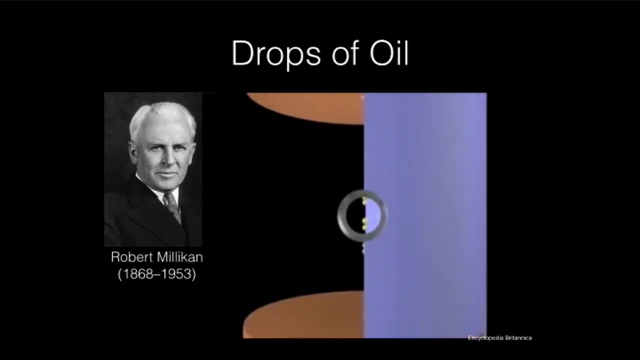 That's not happening. He allowed a fine spray of oil to settle through A hole into a chamber where he could observe their fall. The top and bottom of the chamber consisted of electrically charged plates. He introduced a source of X-rays which can cause creation charges when they strike manner, charges produced by the X-rays attached to an oil droplet, producing one or more charges on the droplet. 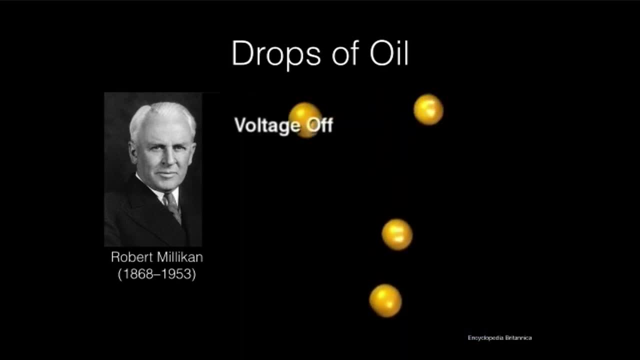 When there is no voltage applied, the fall of the droplets is determined by the mass and viscosity of the air through which they fall. When a voltage is applied, the droplets that have a negative charge will fall more slowly, stop falling or even rise, depending on the number of charges on them, by adjusting the applied voltage and 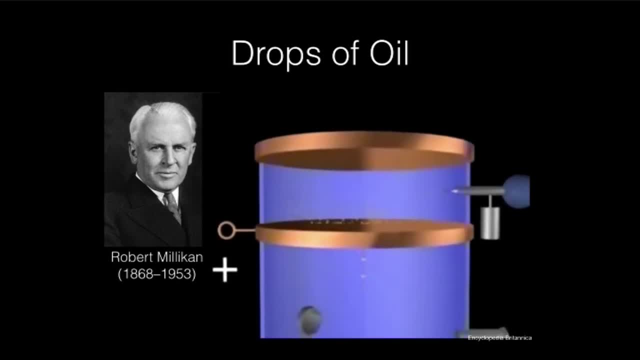 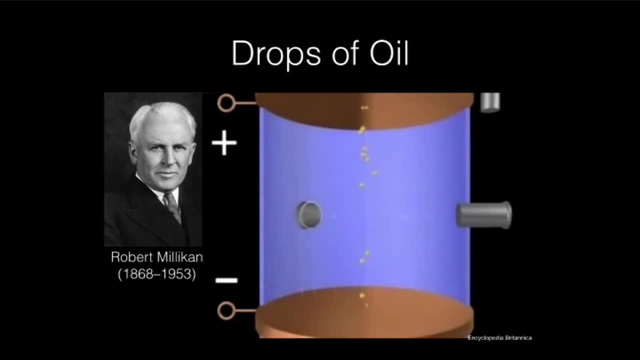 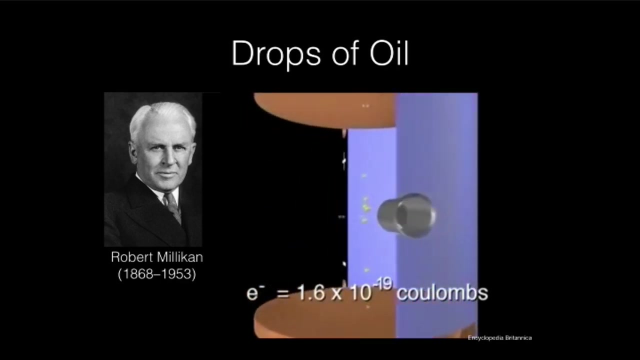 observing the droplets both with voltage off and voltage on, milligan was able to determine that the charges on the droplets were all multiples of a smallest value, 1.6 times 10 to the minus 19 coulombs. he took this to be the charge on a single electron. all right, so now you can see. 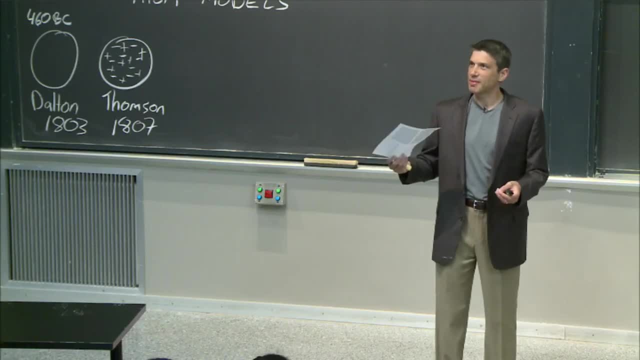 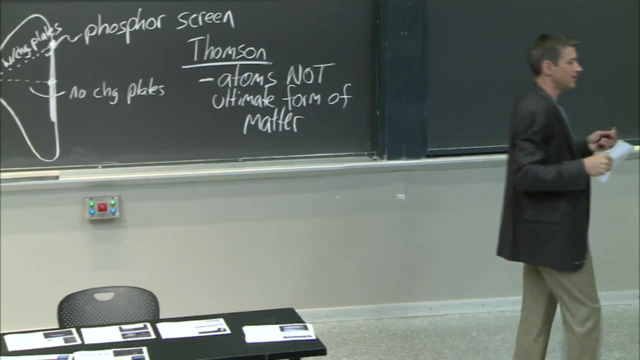 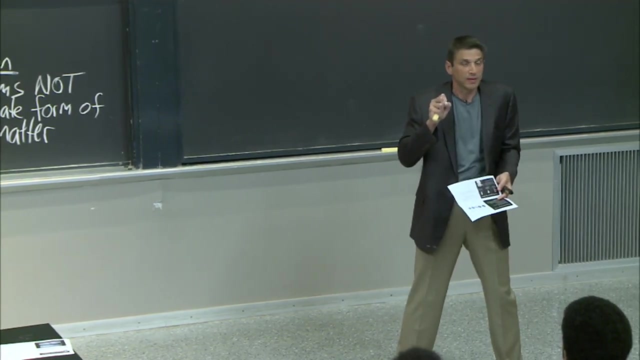 that that would have been. i hope that was. uh, could you hear that in the back? sort of: okay, all right, oh, i got that, i got this. it's good. i, i, uh, i. you know that would have been hard for me to draw the animation, but what a brilliant experiment, right? so spray some oil in a container. okay, try to get. 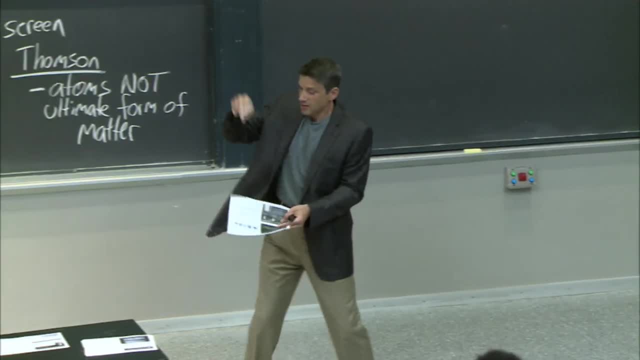 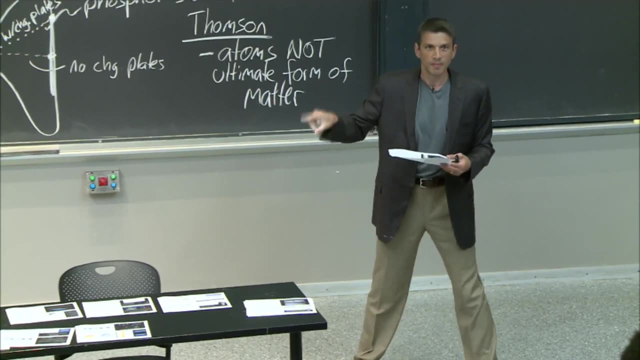 the drops small, you don't know how small they're going to be- and then, as they fall, okay, have a, have an electric field in there inside there, and then, as they fall, zip them, zap them to charge them. You also don't know how much charge you're putting on them, right? 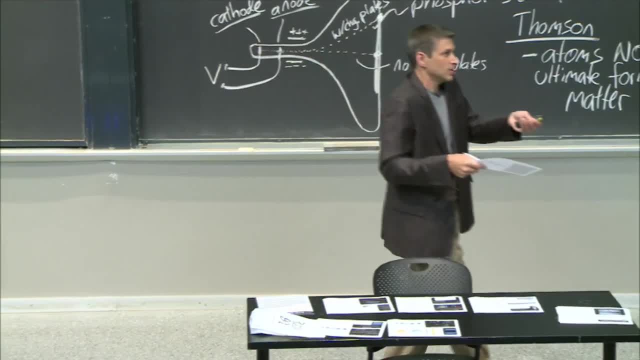 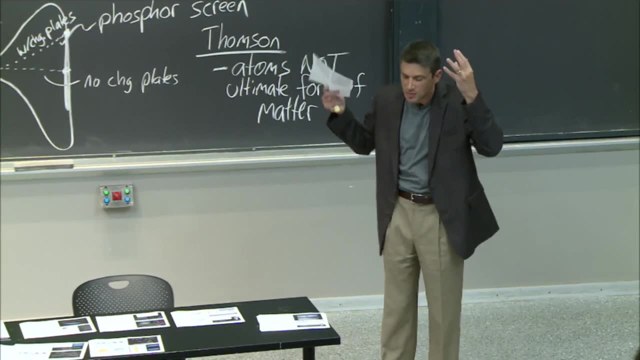 But you're charging them and if they're charged and they're in a field and they're these tiny little, microscopic droplets of oil, they're going to maybe slow down or suspend or maybe even go the other way. And what he observed by doing this over and over again, that there was some multiple that. 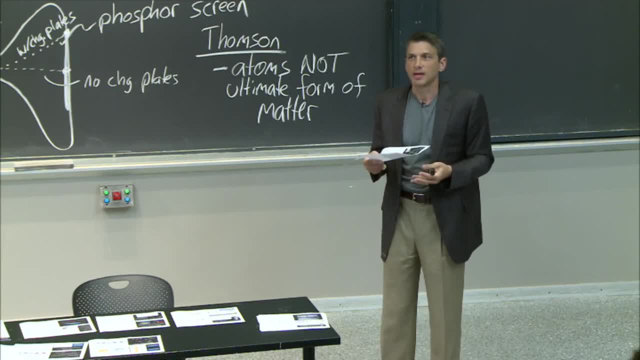 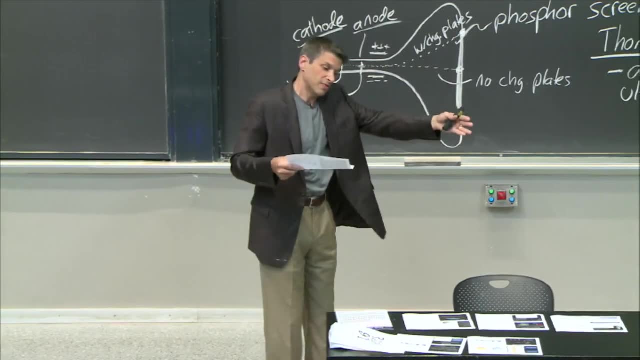 you never got below right And you couldn't say necessarily for 100% certainty that it was the fundamental charge of the electron. It might have been a multiple of that, but it was pretty clear You could never get below that. So that was the charge discovery in this detective story. 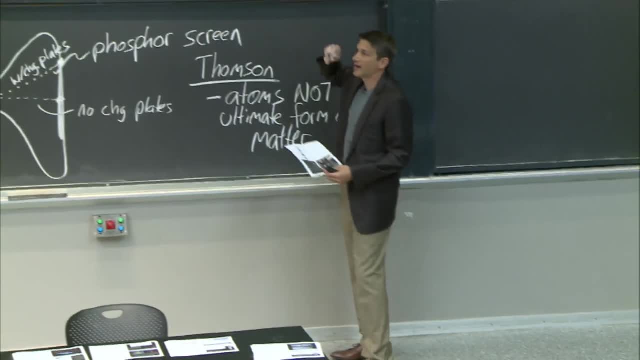 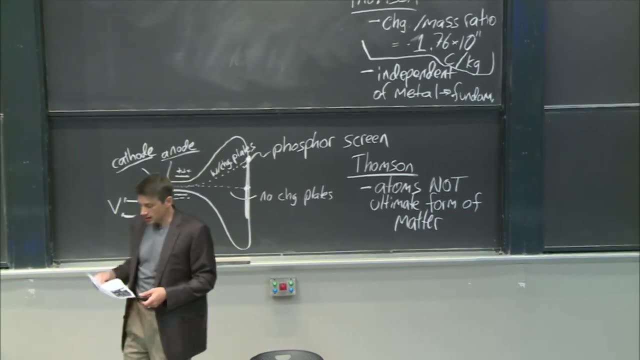 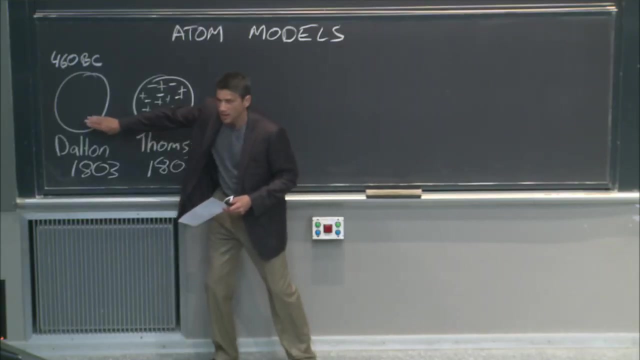 And it allowed us to understand that the electron had a mass and it had a charge, and that we knew both of them at the time. So at the time, then, we already had a much deeper understanding. if you think about it just four years later. 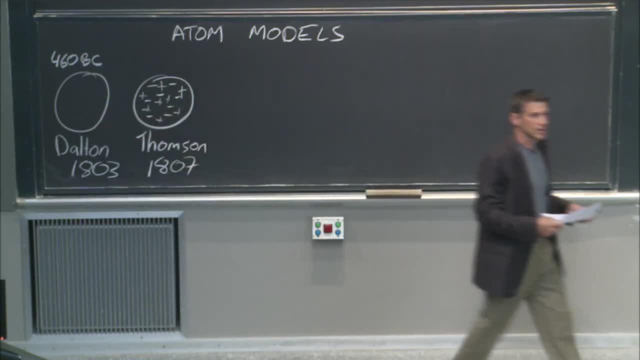 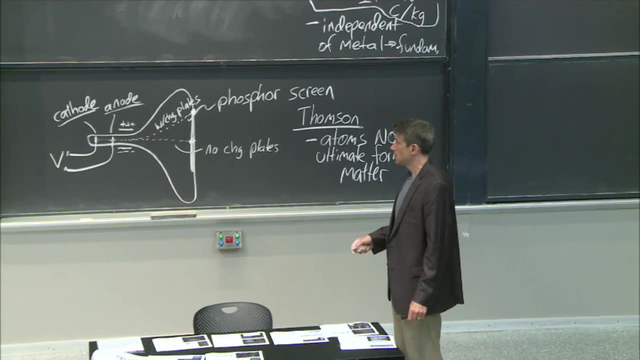 In the time of Dalton because of these two experiments. Yeah, So you said that Tomson was 56 to 1856 to 1940, so wouldn't that be 1907? 1856 to huh? You said that Tomson was alive. 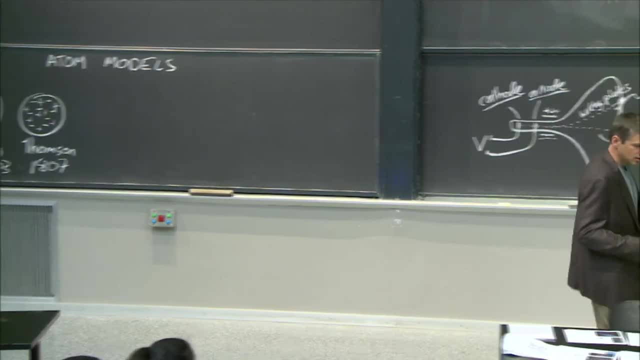 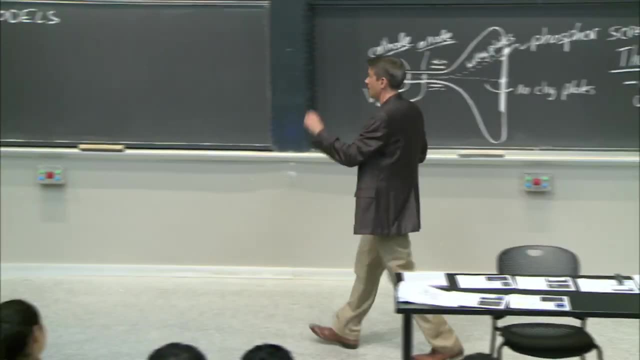 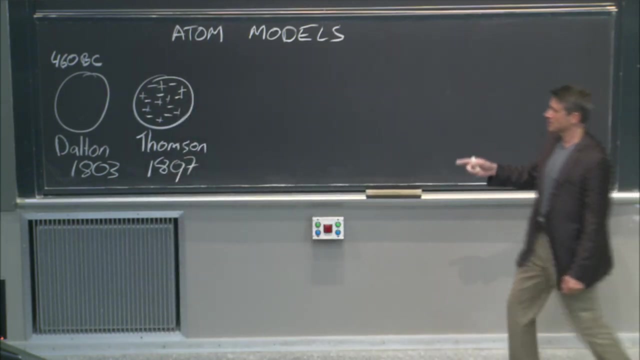 Alive 1856.. I read: I think I read my. he was ahead of his time. thank you very much. I think I read this wrong and that's because I don't have my glasses on. Okay, So now that I look at that, it wasn't that small of a distance. 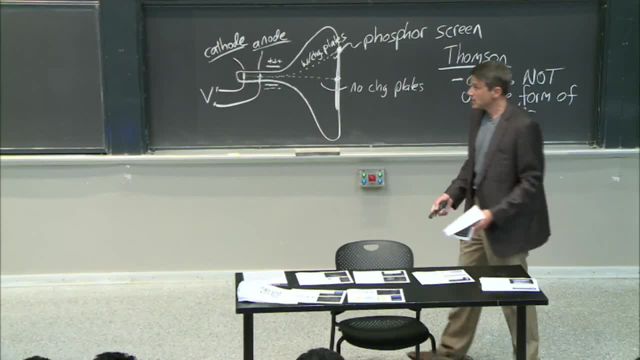 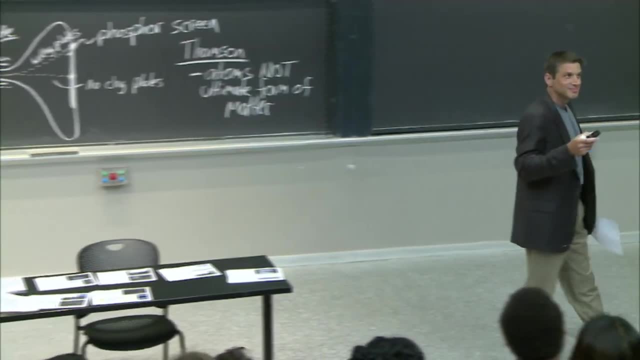 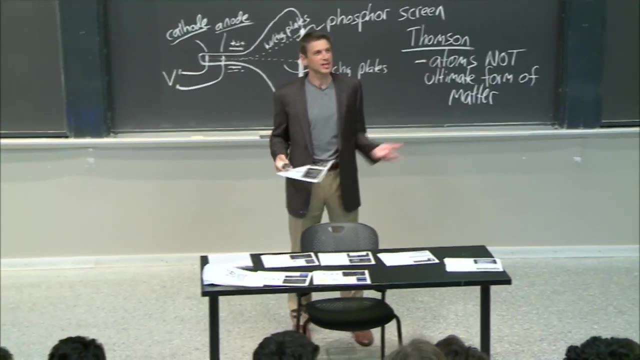 Thank you very much. You make mistakes, You make mistakes and you. that is how you learn. You won't make progress. progress has almost nothing to do with success. I mean this. I'm using my own mistake here as an example. 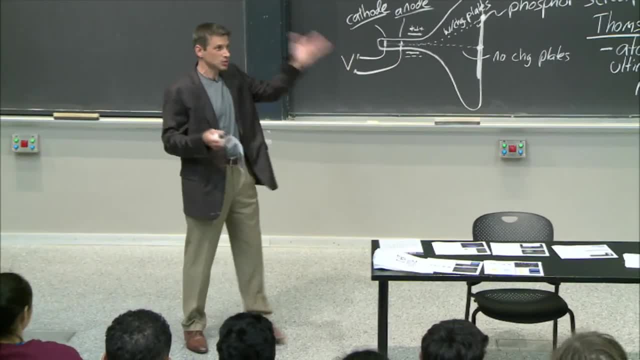 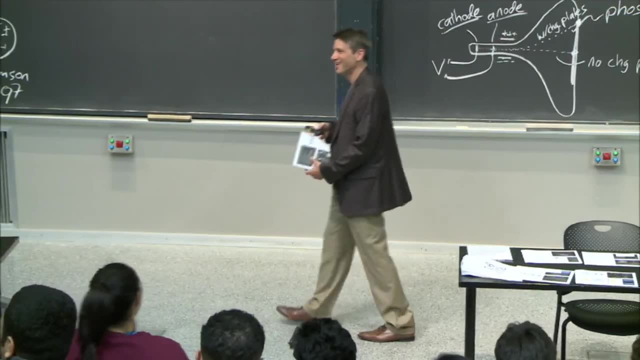 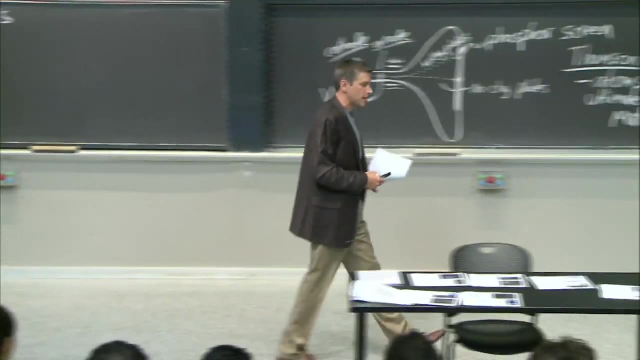 I, I don't know. Progress has almost nothing to do with success. Progress has only to do with what you choose to do with failure. Did somebody just say, whoa, Thank you, Thank you, that hit me here. Alright, Okay, let's do a why this matters. let's do a why this matters. 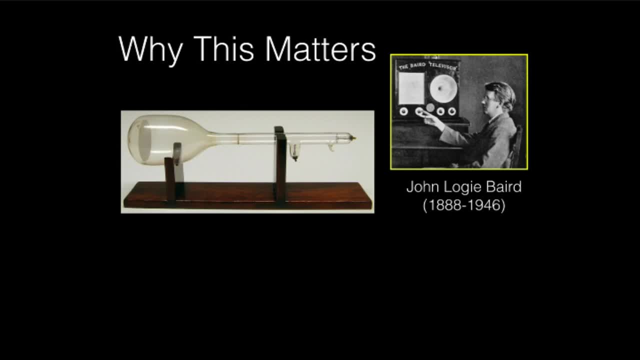 Why does this matter? Well, because see, these guys were trying to figure out what was inside of an atom. Yeah, Yeah, Yeah, Yeah, Yeah, Yeah said. well, wait a second, you just gave me a paintbrush. 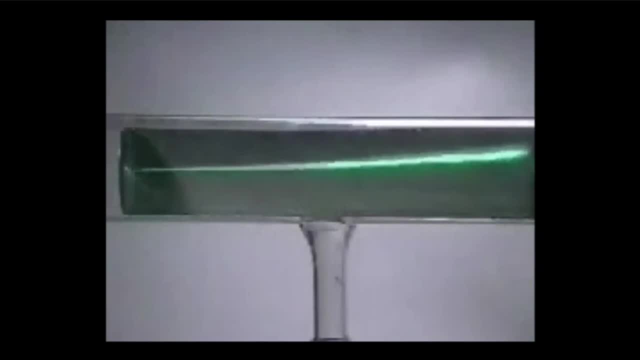 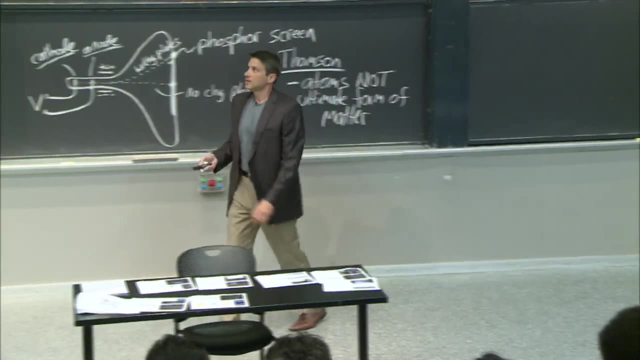 You gave me a paintbrush. Look at this, That's a paintbrush, Painting with a magnet. It really is, And the screen would light up over here. And so he said: well, I can paint pictures. And this really is the first television screen. 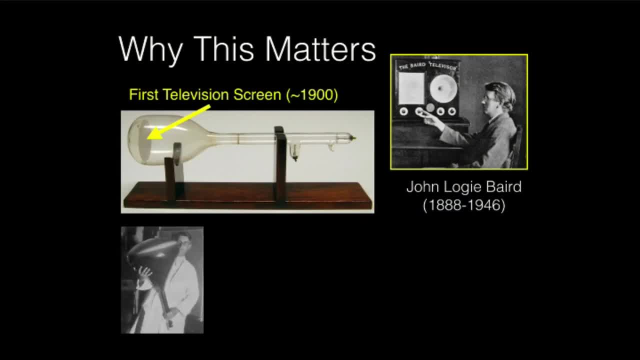 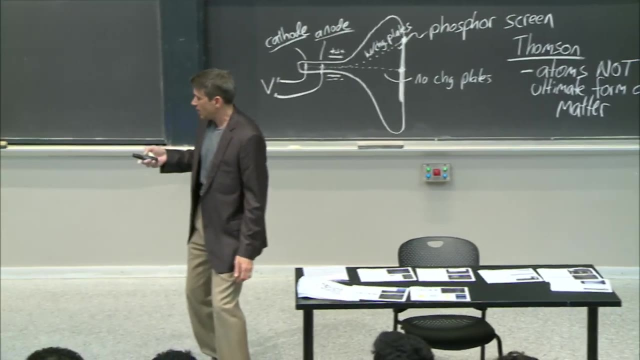 This was the first TV screen And all they needed to do. they're okay, right, There it is. That's a cast-out rim tube. Maybe that's one of Thomson's students who won a Nobel Prize, But now you put this down and you put these sort of things around it. 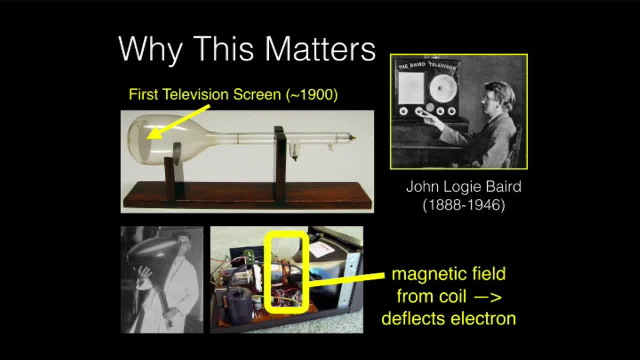 What are those things? Magnetic fields, That's all it is. It's just magnetic fields. It's Thomson's experiments, right? But now they're using it to zip the beam around faster than your eyes can keep up with, so that it looks like a picture. 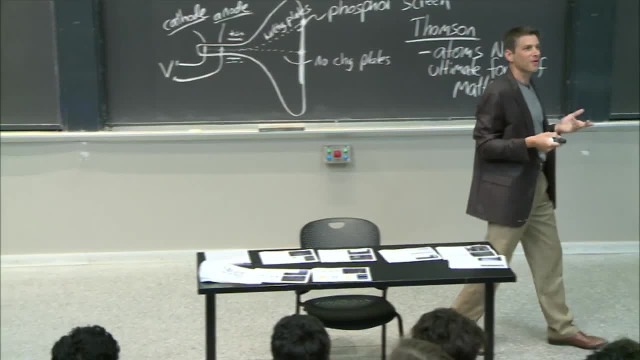 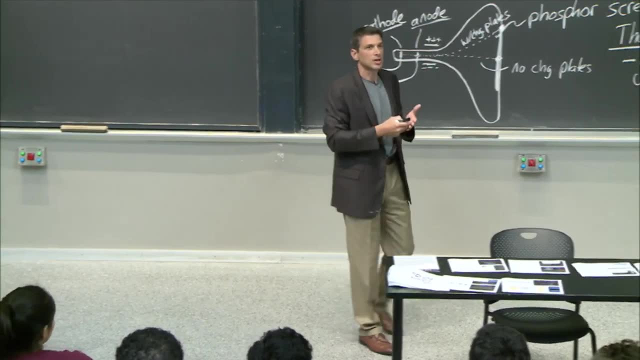 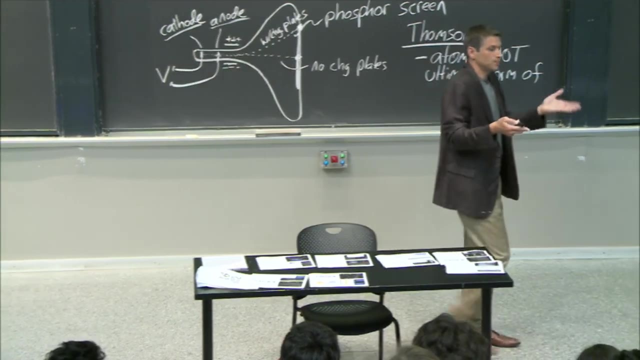 Now, electron painting had never been done before, Because we didn't know that we had these electrons. But as soon as we knew, boy did that launch a completely new era of screens. Right, The era of screens. We don't use cathode ray tubes. 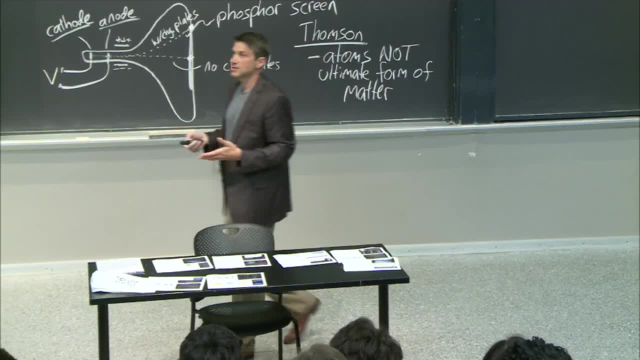 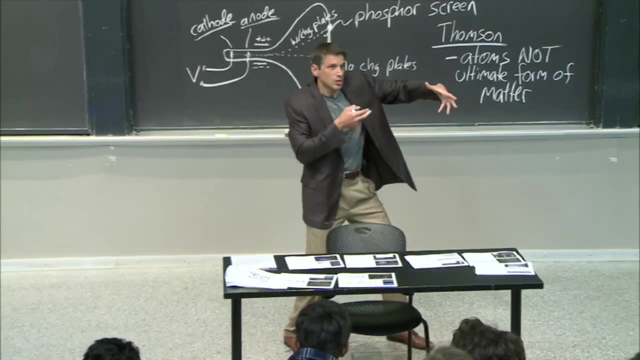 They'll just say: ask your grandparents, They'll tell you about the cathode ray tube TVs which they all had. But you know, we don't use cathode ray tubes to paint with electrons today in that way, But we still paint. 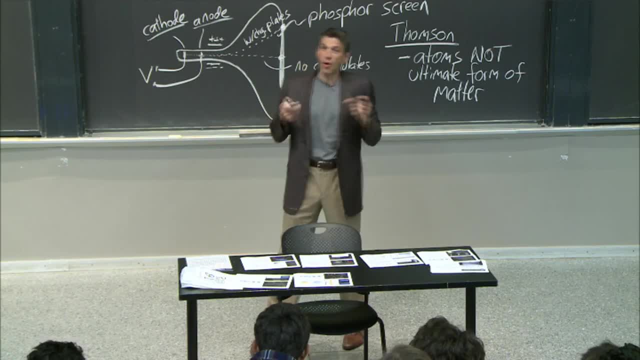 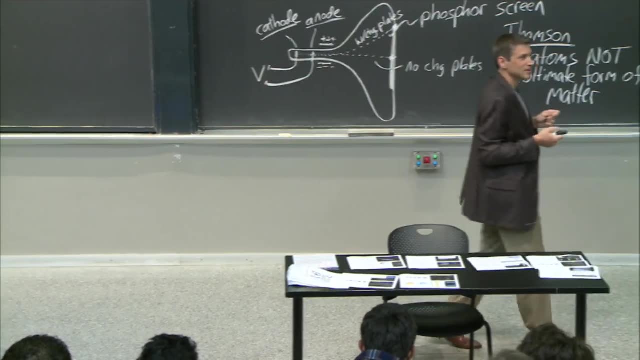 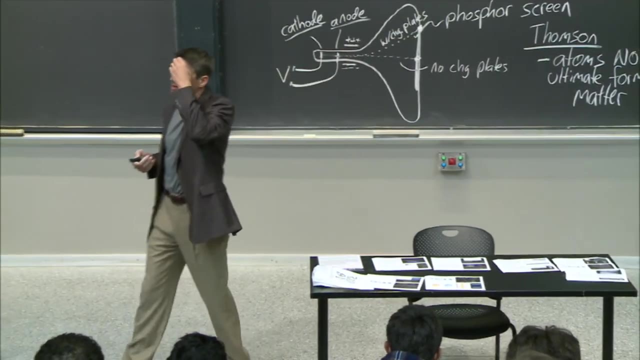 We still paint with electrons today, Right, Your OLED screen is still simply an electron-based painting tool, Right? Right, Okay, We're just pumping the electrons into the phosphor in a different way, Right, And we'll be talking about that as we go through the rest of this week. 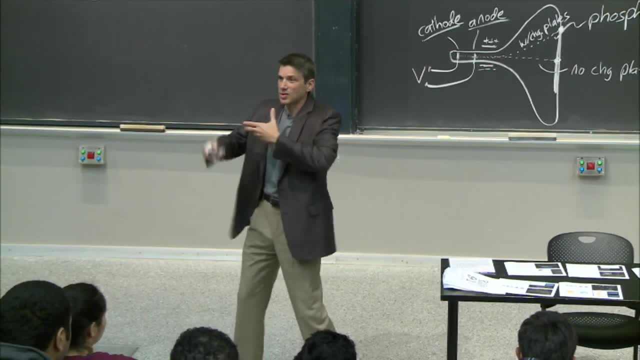 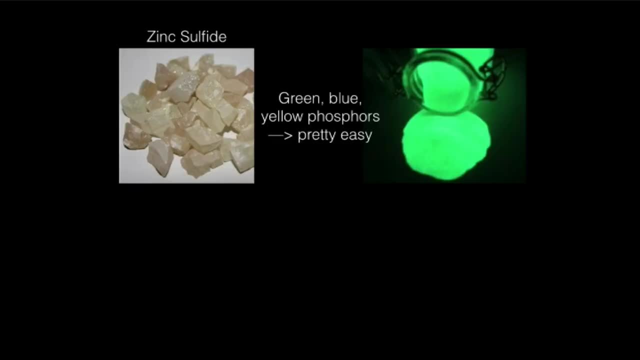 And we understand how electrons interact with light coming in and out of an atom. Okay, So that's why this matters. And, by the way, a side note here Is that When TVs first came along it, you know, green was pretty easy. 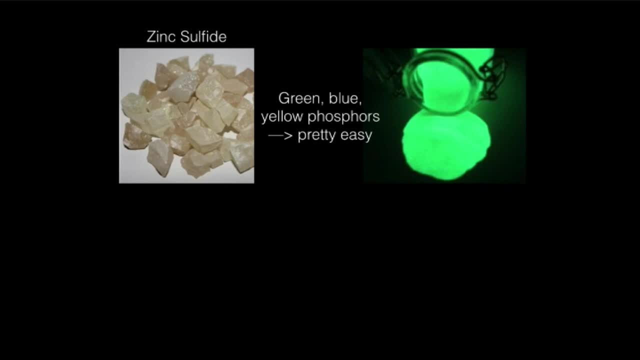 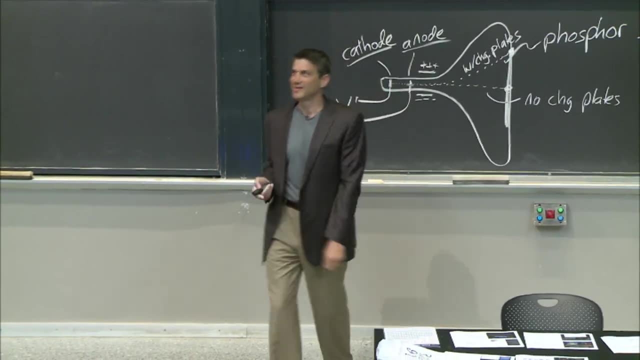 There were a lot of chemistries that were used for this screen. Right, You put a different chemistry here and it lights up differently when electrons hit it. Why Wait until Wednesday? Green was easy, Yellow was easy, Red was hard. 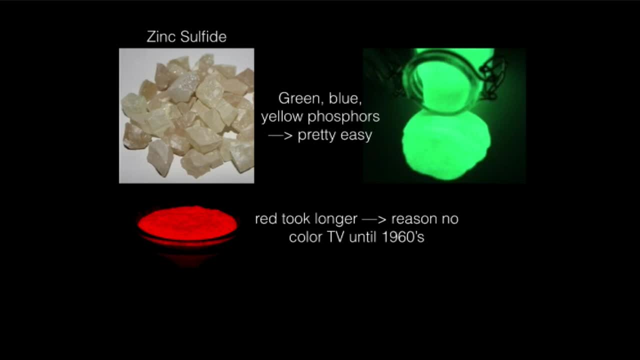 Red was hard, They couldn't get a good red And, of course, and that's why there were no, that's essentially the reason there were no color TVs Until the 60's Right, And the answer, of course, was here: 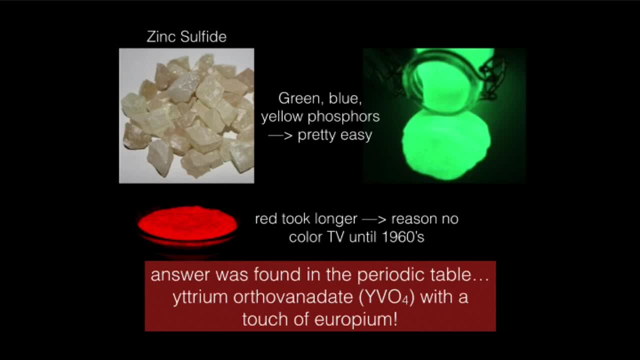 The answer was that there was a phosphor that worked, but it was yttrium orthovanadate, With a little bit of europium added to it- Just a little bit of europium. Why did that work? Again, we need to understand how electrons interact with matter, which is where we're going. 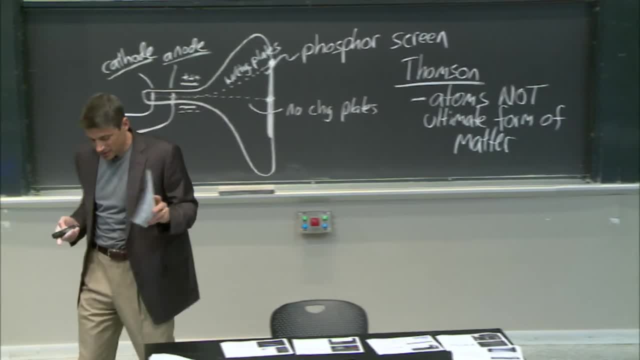 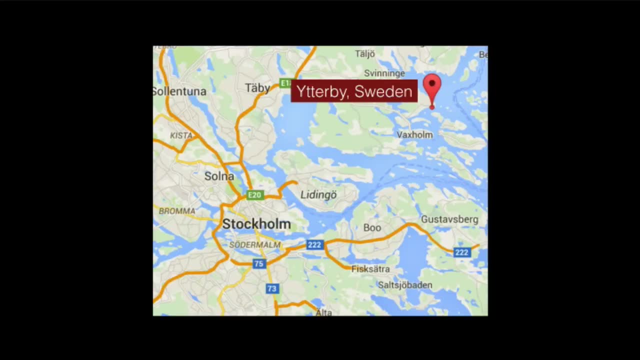 And speaking of yttrium, Speaking of yttrium, This is also a side story, but it's kind of a good one. This is also a side story, but it's kind of worth noting. You know, elements are named often. well, elements can be named after many things. Alright, In this case it was named after Ytterby Sweden. Ytterby Sweden is a pretty cool place. They have this one cave. You gotta go to it. It's really cool Because four elements of the periodic table were all discovered from Ytterby Sweden in this one cave. 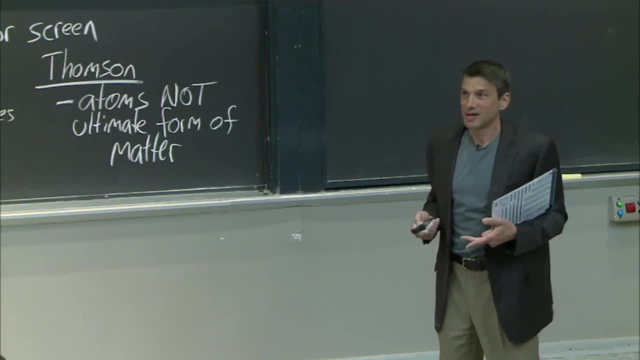 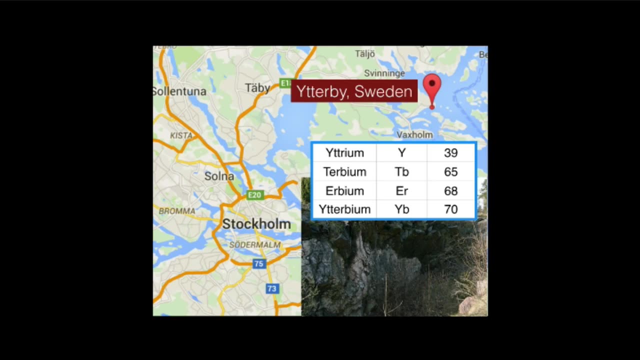 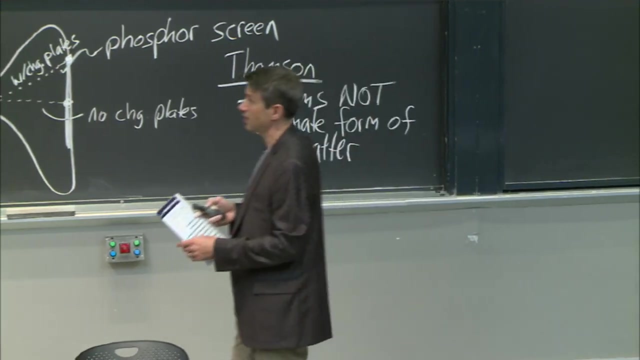 Four And I keep thinking: where is that cave in Cambridge? They can't, they cannot discover any more elements because there's no other way to mess with the name Ytterby. That's pretty cool. That's pretty cool. That's a cool cave. 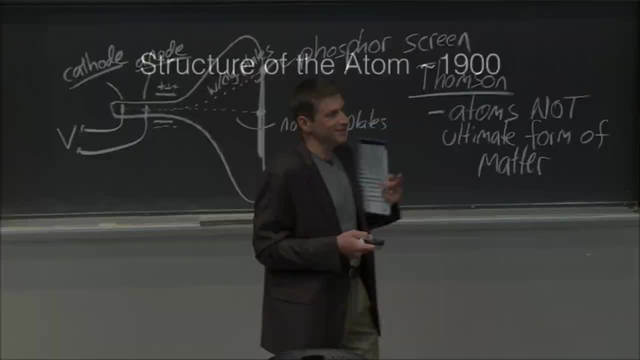 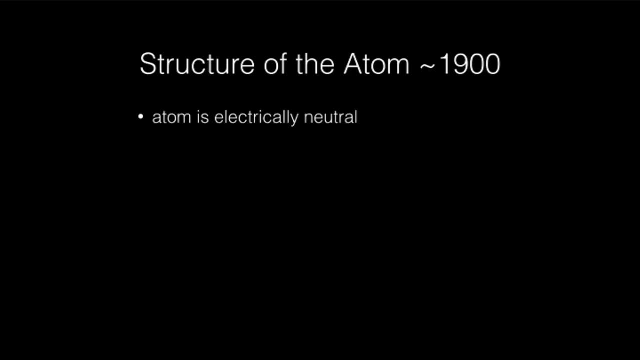 That's worth visiting. Alright, So the structure of the atom in the 1900,. thank you for the date correction- 1900.. The structure of the atom was as follows: Alright, The atom is electrically neutral, But there are these negative charges. 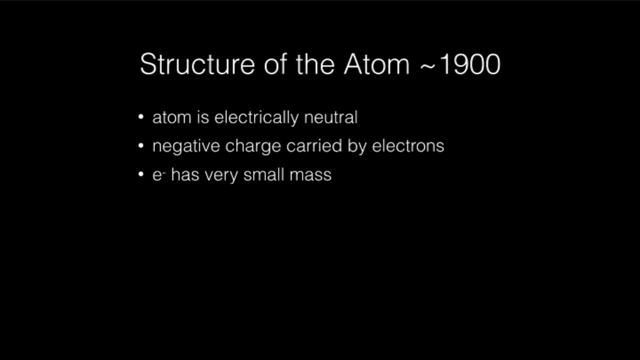 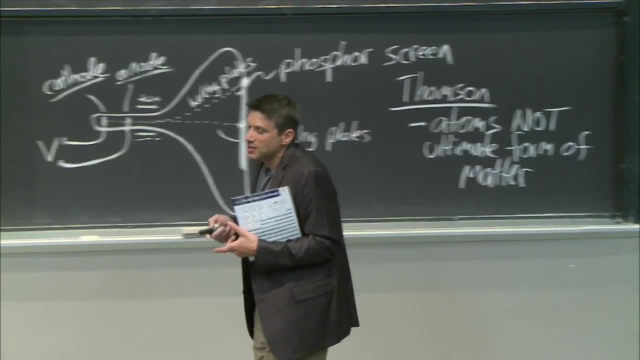 These negative charges called electrons. The electron has a very small mass. We know that from the oil drop experiments, Right, Which means that the bulk of the atom is positive, because the bulk of the mass of the atom, right, You know, the atom weighs one thing. 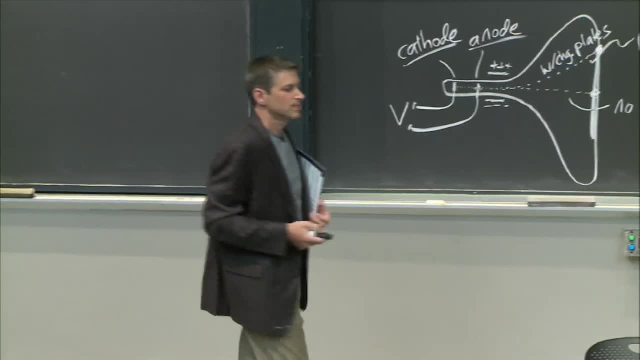 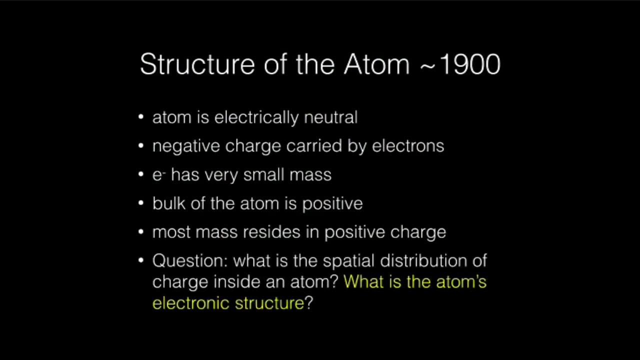 The electron is just a small part of that in terms of the mass. So most of the mass is positive And there was a question: Okay, So we're getting somewhere. But how do these charges really look? How do these charges arrange inside of this atom? 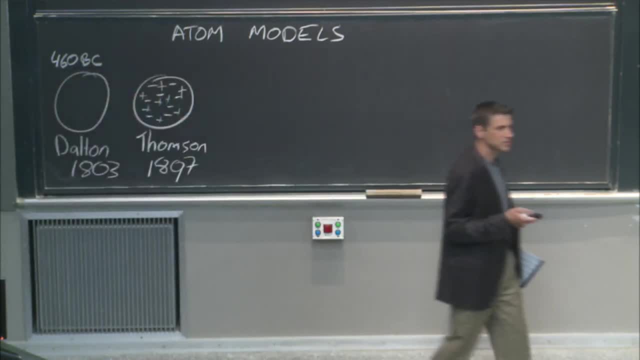 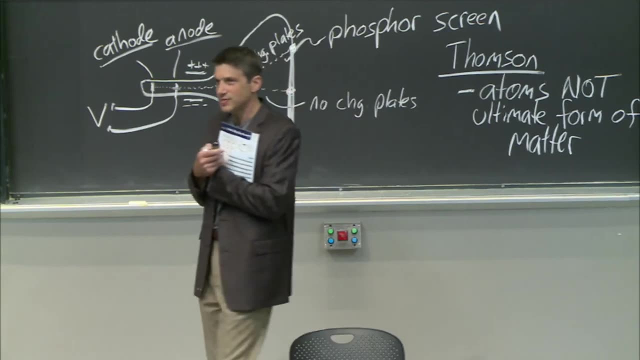 Is Thomson really right- And that was the next part of our detective story- Was to really understand what these charges are doing inside the atom. I'm carrying this around like my security blanket, Which is making me feel very secure right now, And you should all carry it too. 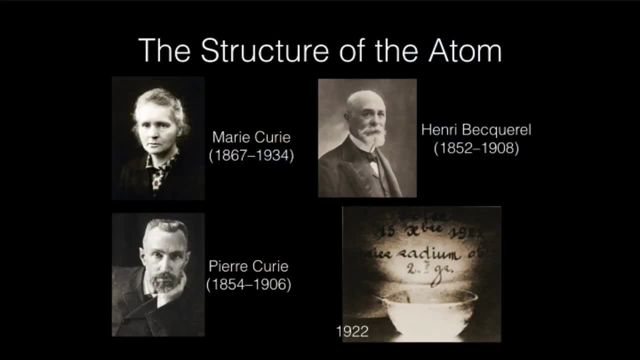 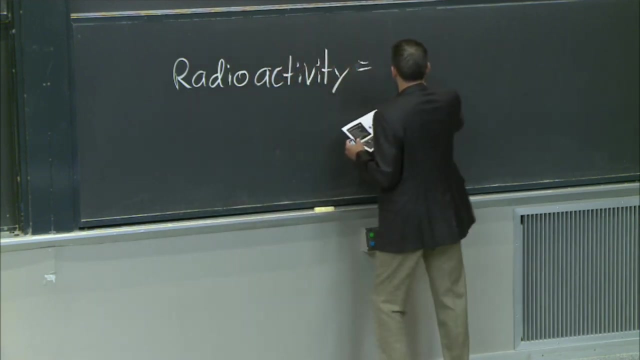 This part of the story relies on another type of energy that was being discovered at the time, And you all may remember, And you all may recognize this as radiation. Now radioactivity. Radioactivity is nothing more than ray activity. This is what they named it after. 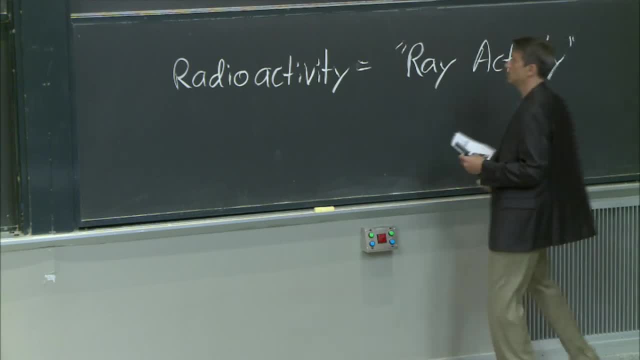 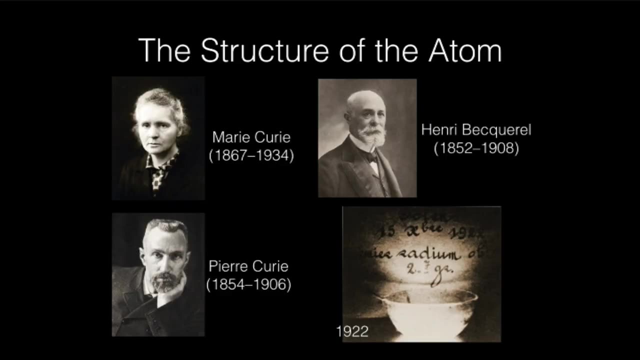 Ray activity, That's radioactivity, And it was these three people who really pioneered the understanding of radioactivity And, in particular, the fact that some elements seem to just be radioactive. What did that mean? Well, it means they gave off these rays of energy. 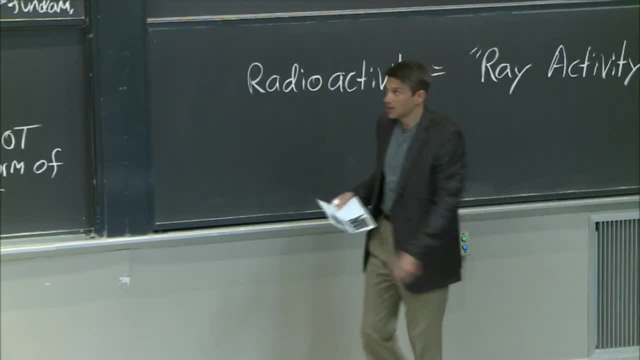 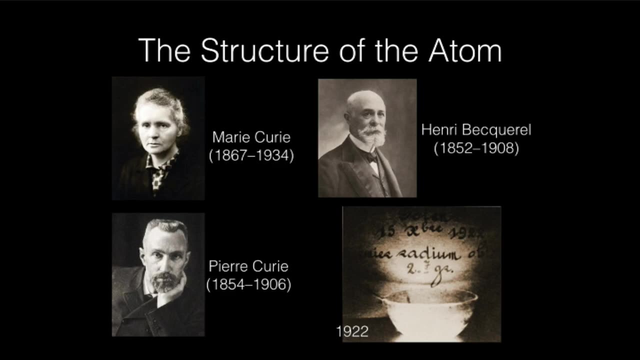 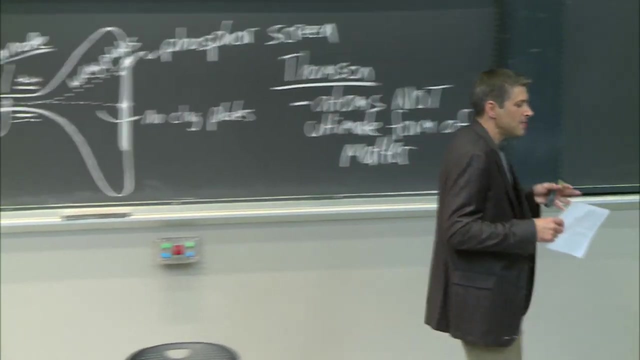 It means they gave off these rays of energy. You had Henry Becquerel, You had Marie Curie and Pierre Curie. Notice, I didn't even try Where's Jerome? I didn't even try with the French, But anyway, They took these materials like uranium ore. 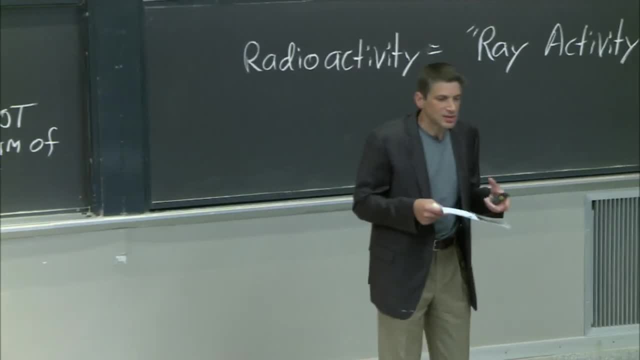 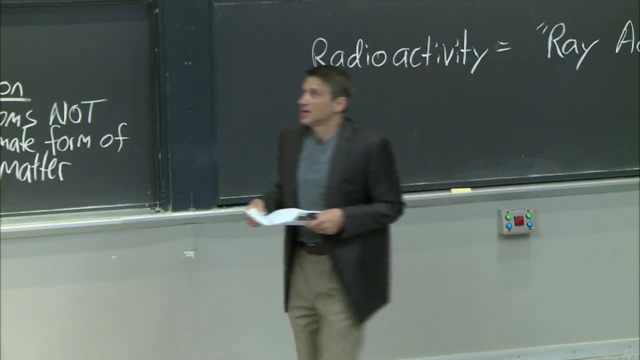 Right: Minerals made out of uranium. And they said: this stuff looks like it's got something coming off of it. Let's see if we can find what elements are causing that. Right. And Marie Curie won. She found polonium and radium this way. 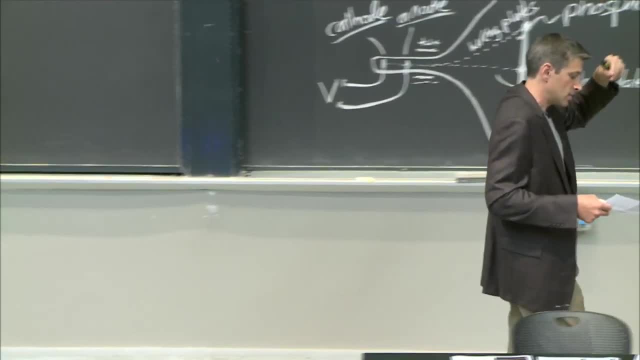 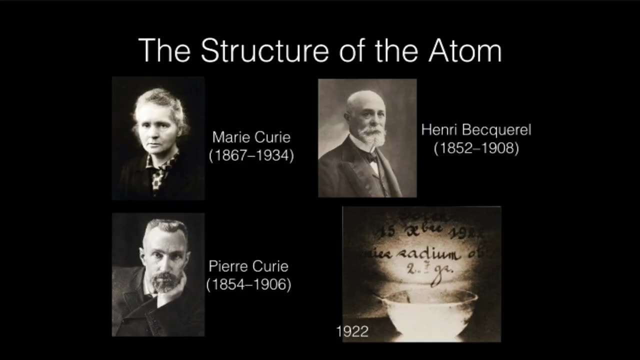 Those two elements- Polonium- named after her home country, Her native country of Poland, And this stuff was so, And this stuff was so, It gave off all this energy And it was so energetic They could literally put it in a cup. 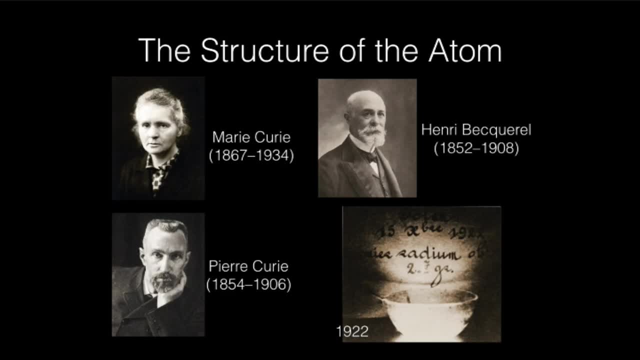 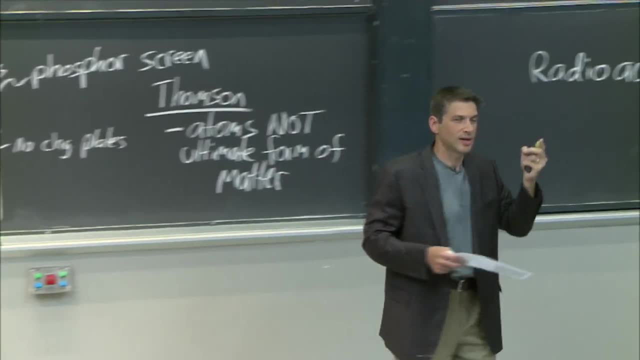 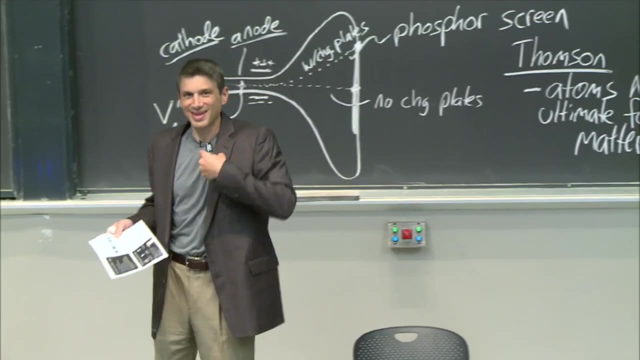 And have some writing there And put it in a super dark room And it would illuminate the picture. Right, It would illuminate the picture, But this is not a recommended way to light your pictures. So Pierre carried a vial of radium. 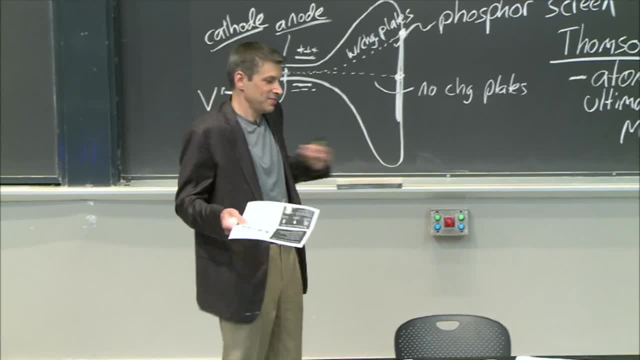 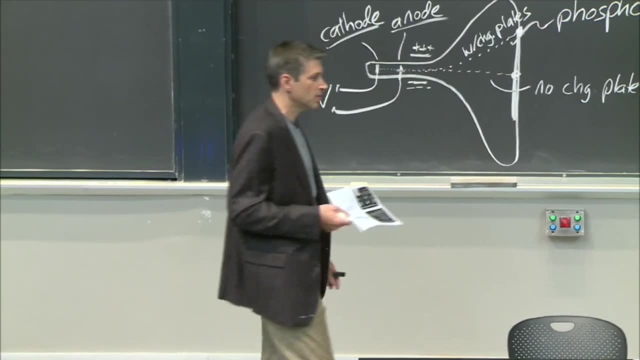 Because it was so cool and it glowed. He was like: look at this stuff, Right. And he actually did have bouts of radiation poisoning, Although he died tragically when he was struck by a horse-drawn carriage in 1906.. 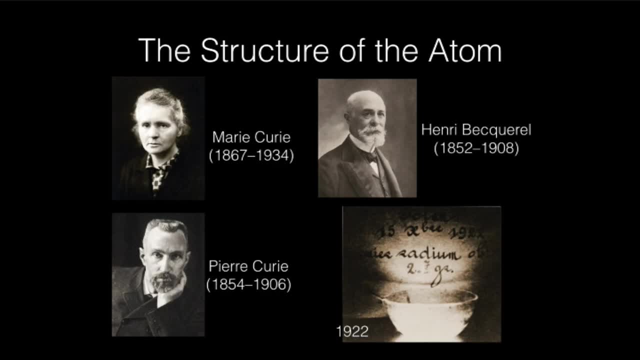 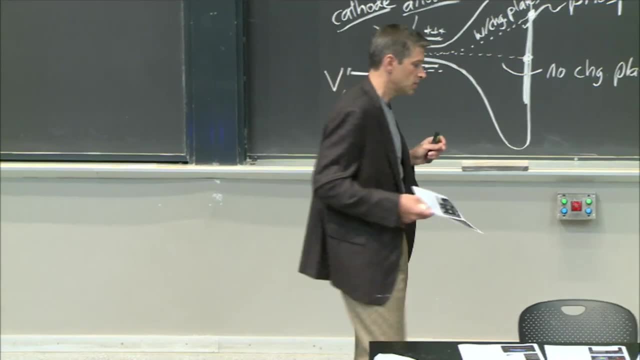 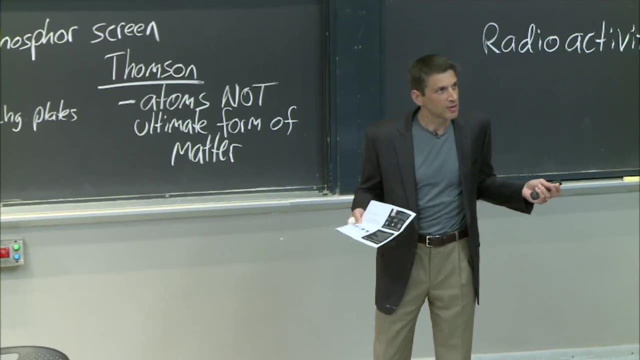 Marie lived much longer And won two bouts But also died because of radiation poisoning. But she won two Nobel prizes: First woman to win a Nobel prize, Only woman to win two And for only person ever to win two And won in two different disciplines. 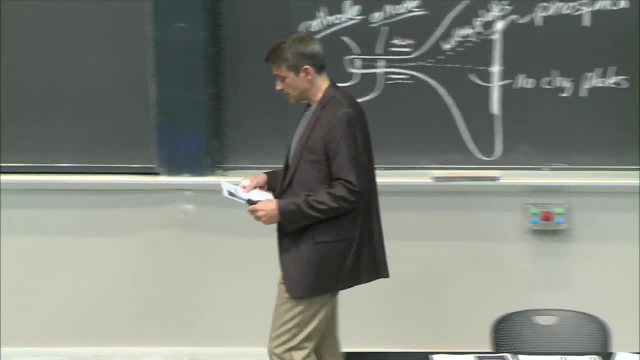 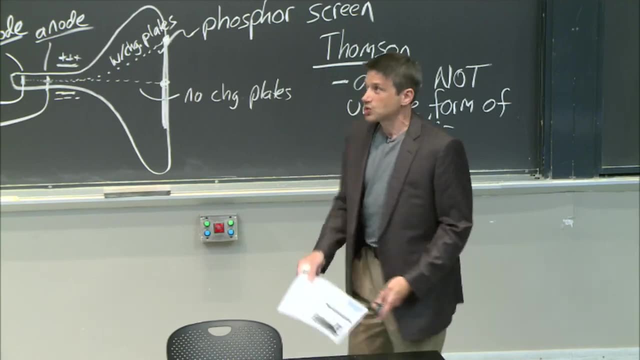 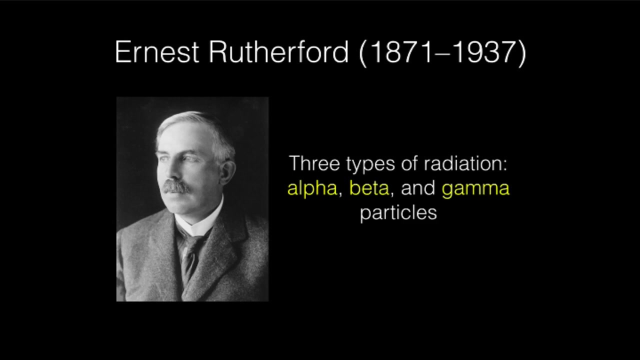 Physics and chemistry. She was quite a brilliant scientist. And they gave us this radiation. Now, OK, But see, OK, They were really into radiation. But it was Rutherford who said: well, wait a second, Maybe I can use this stuff to keep going along this story. 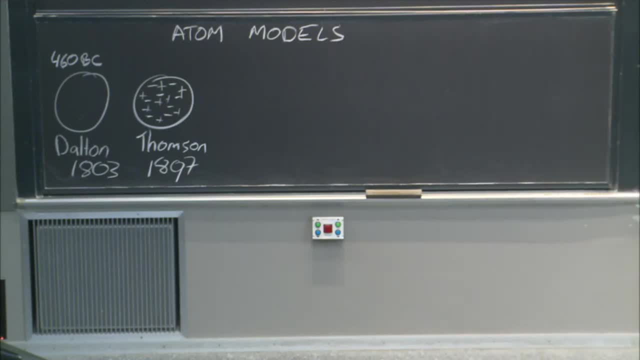 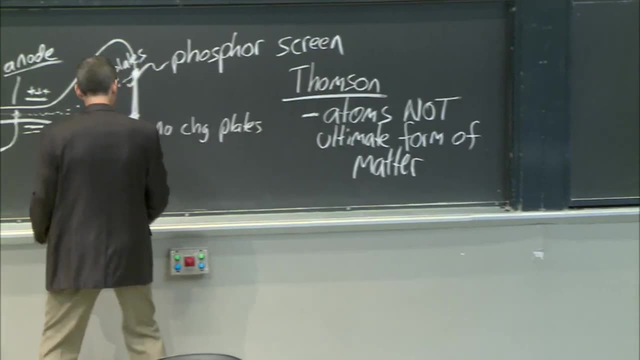 Right. Rutherford was like: well, maybe there's something we could do with this radiation. And so what happened? He was like: there it is, And so I'm going to put it right above it so you can see. So he said: well, OK. 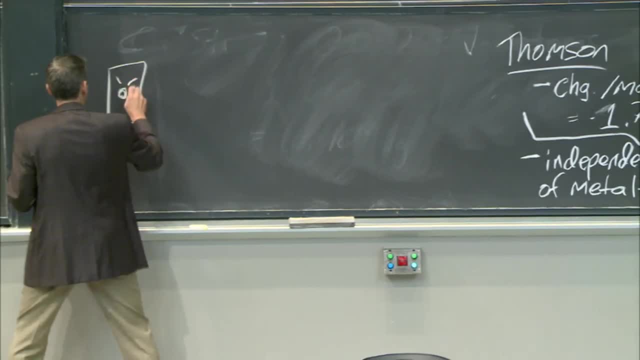 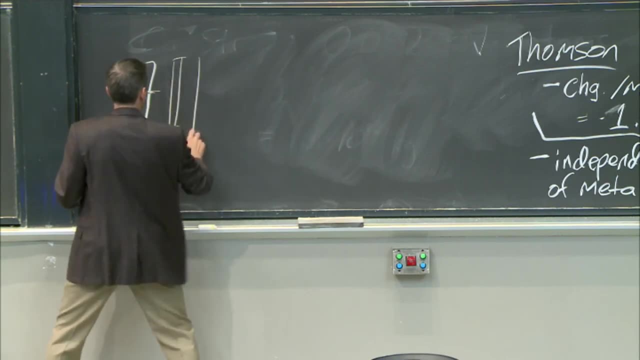 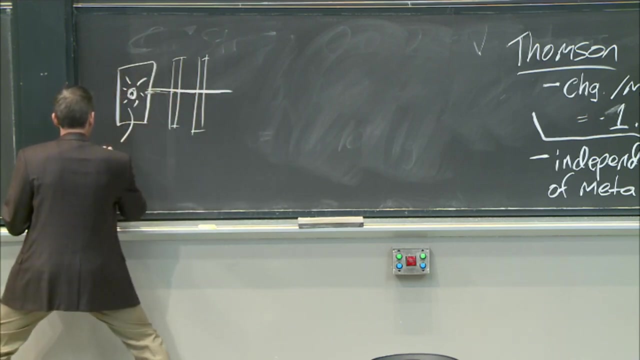 If I take something that glows, maybe some radium, And I carve out a little thing here And maybe I put some plates to kind of protect scatter, I can make a beam of this stuff OK. So this would be like maybe radium, let's say. 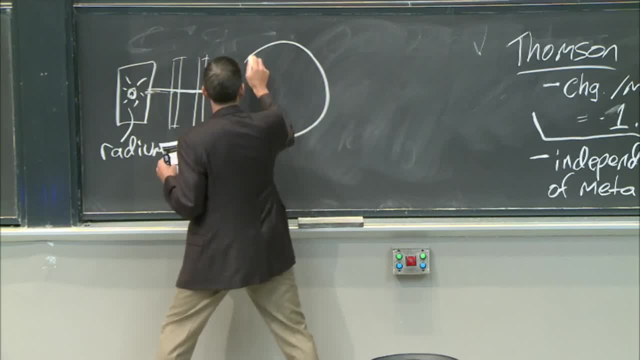 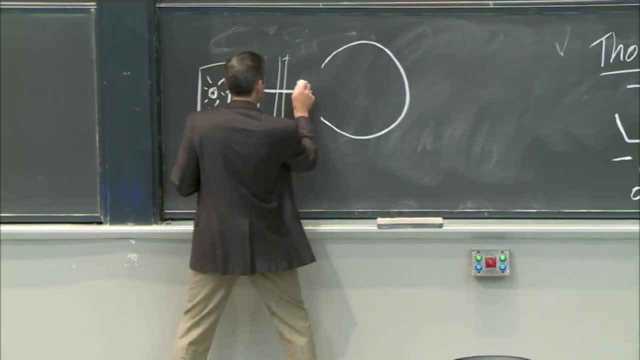 And then what he did is he took this photographic plate And he curved it Just so you could really collect as much as you could, So you can really collect really high angles. And he did the same thing: He put charged plates on either side. 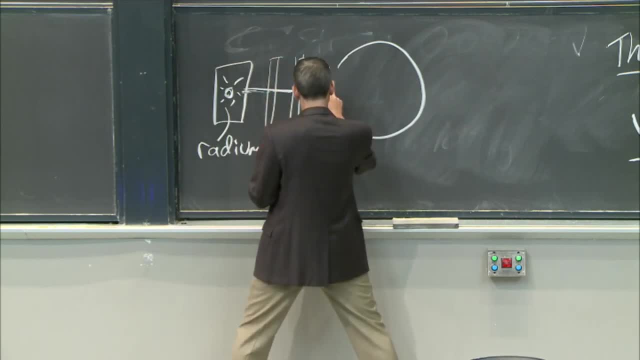 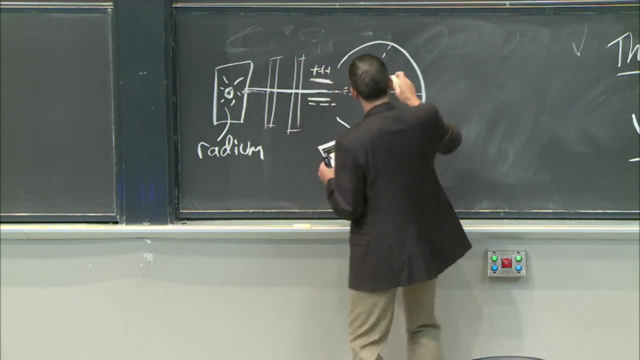 And he found that you had three different types of beams. You had one that went like this, one that went like this and one that went like this. And we now know that this is beta, this is gamma and that's alpha. 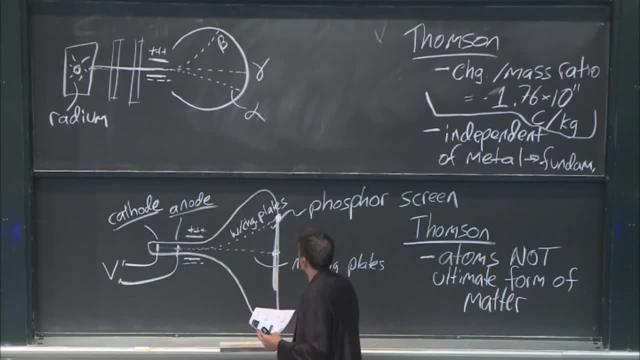 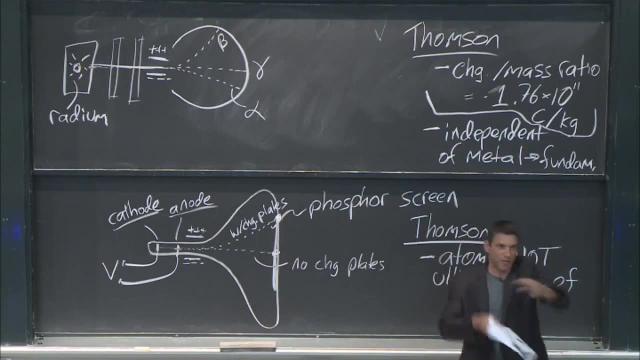 Let's put this right above: This is so cool to watch this. So what Rutherford did is kind of like this: He had stuff And he made a beam of it And then he put stuff around it. But if you've got a beam of something, that might be charged. 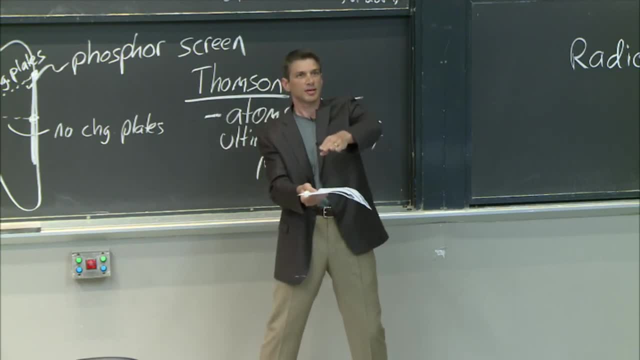 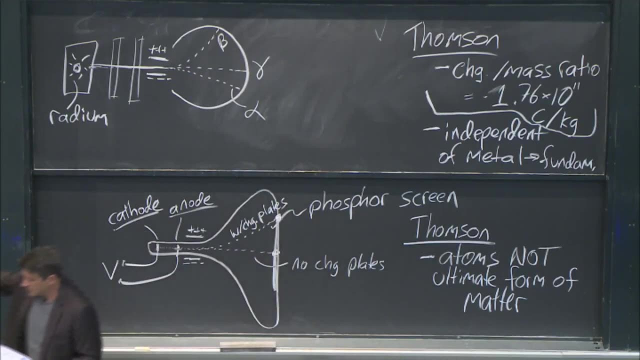 you're not going to smash it or burn it, You're going to put some plates around it or a magnetic field or electric field. And that's what he did And notice alpha bends down towards the negative charge. So alpha must be positively charged. 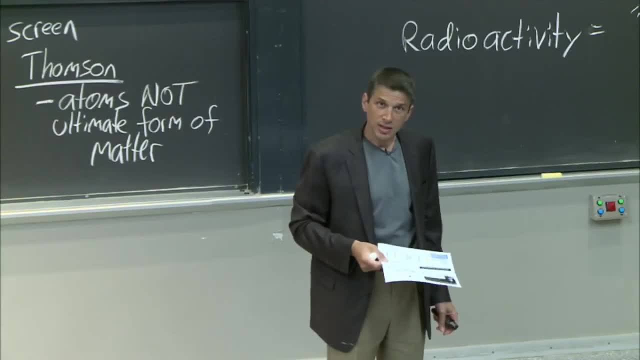 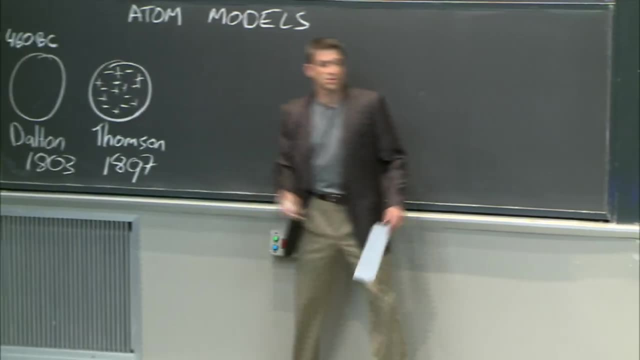 I said: OK, that sounds cool, Maybe I can use this, Maybe I can use this on this, on this question of how these things are spatially distributed. So then he said: OK, let's just screen out those alpha particles. 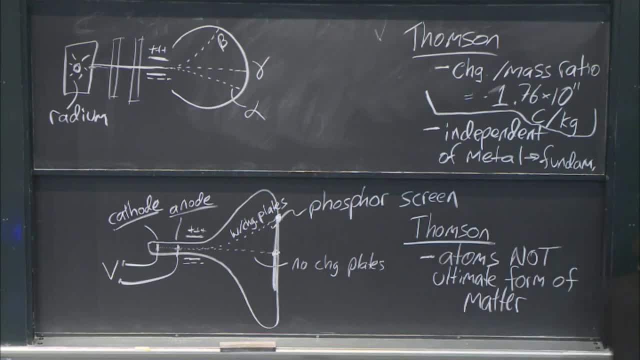 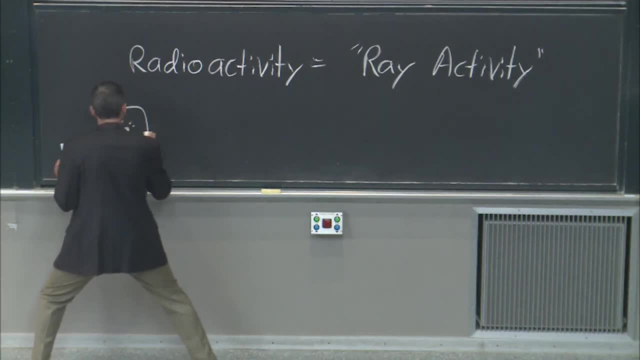 And let's just take these alpha particles And let's shoot them. So now comes the famous experiment. So you had stuff in here, radium making a beam, And you collect it And you make it just alpha particles. So now he's just got all alpha particles. 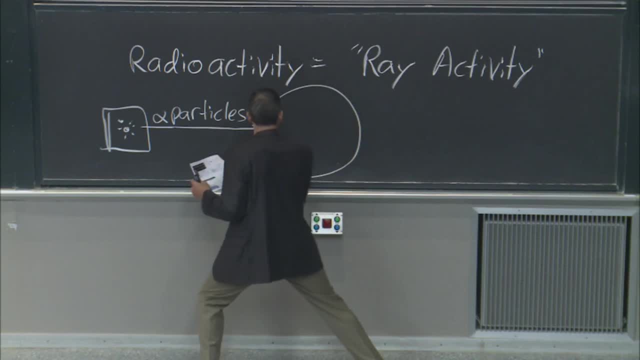 And what he did is he also had a photographic plate, Or this could also be a phosphor screen And you could watch where, If it's a photographic plate, you record things, events, And you can see it like a picture, a film. 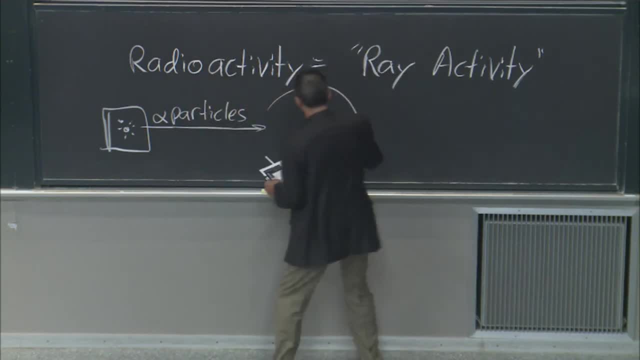 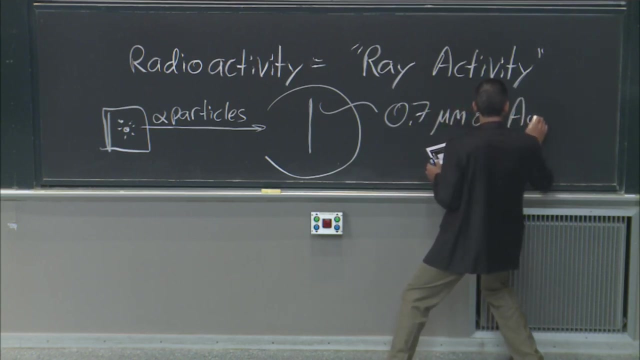 And if it's a screen then you watch it. Either one was used. But what he did is he put a very thin strip of gold in there, 0.7 microns of gold. So that's a 0.7 thickness is 0.7 microns. 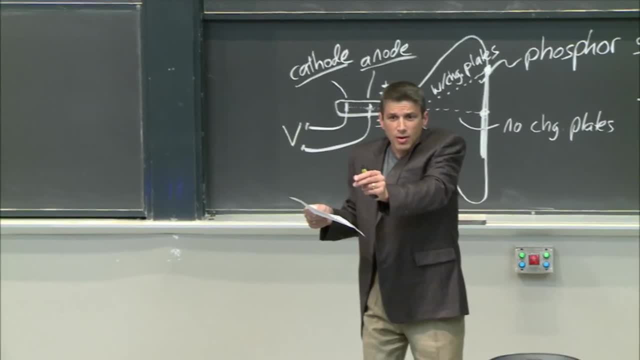 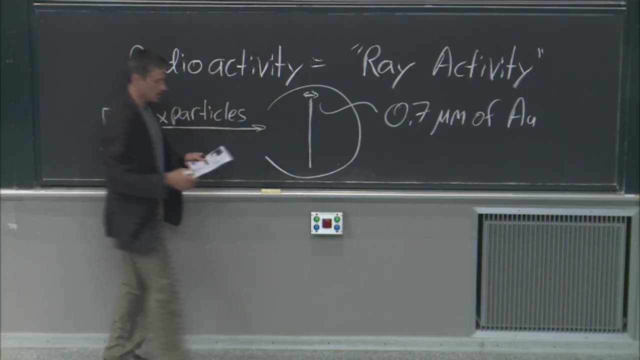 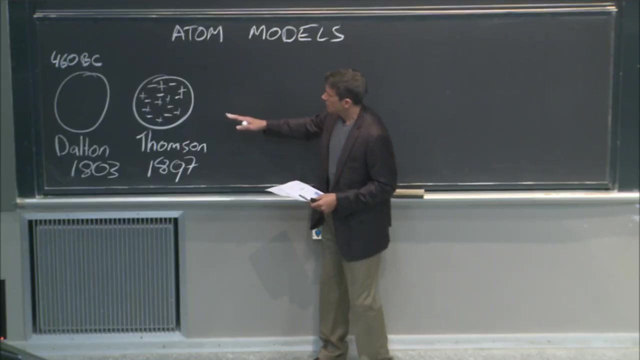 Really really thin, like a tissue paper of gold, And he shot these alpha particles at it. Now, why is this important? Because Gesundheit, because if this model of the atom was correct, then he'd isolated these positive particles. 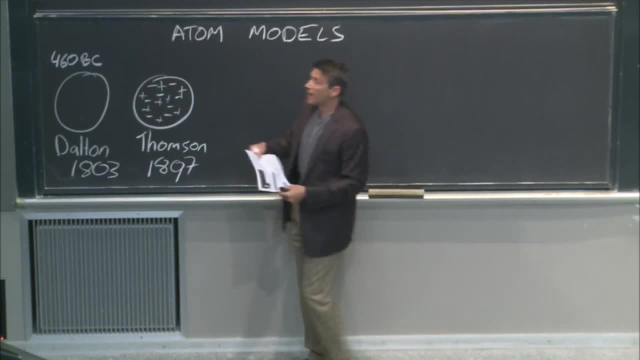 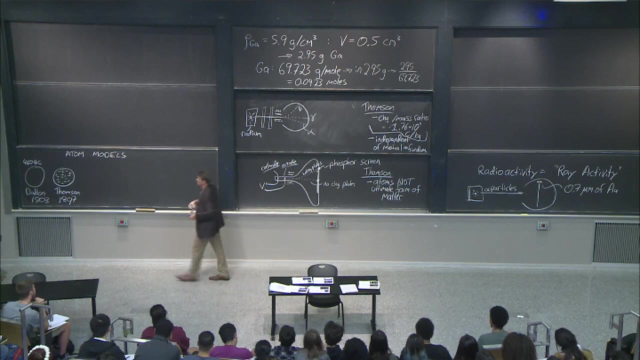 that he's shooting at these atoms, And if that model of the atom is correct, then this is kind of distributed all over And so it's kind of neutral. almost anywhere you look It's kind of neutral, And so you would expect that a positive charge would maybe. 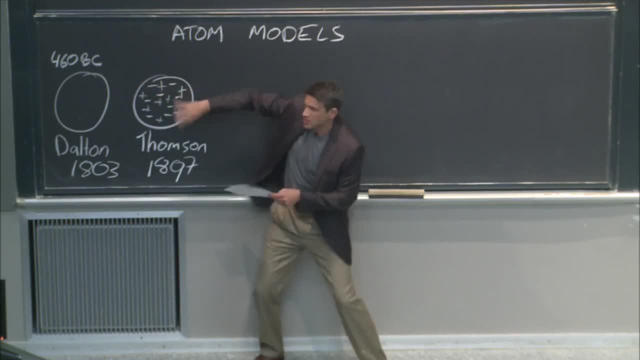 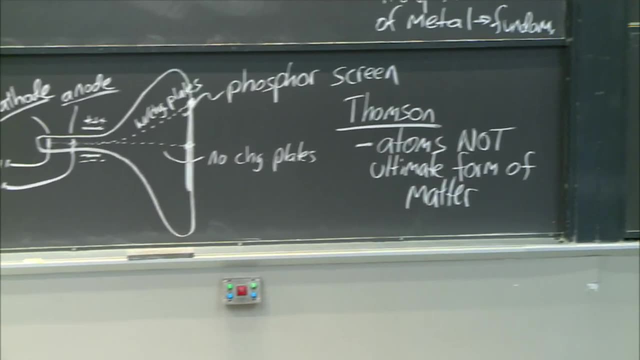 feel a little bit, But it kind of feels mostly neutral because it's evenly distributed And so it would just kind of come out. But that's not what he saw. That's not what he saw. What he saw is that sometimes that would happen. 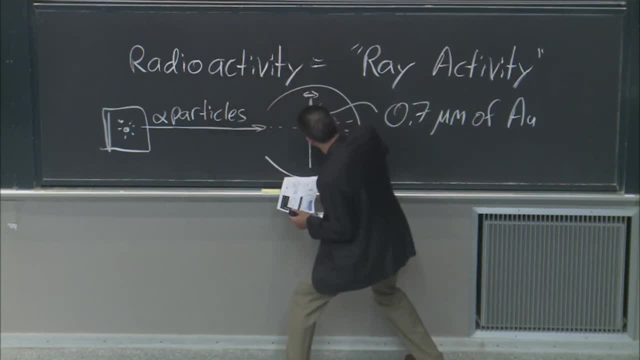 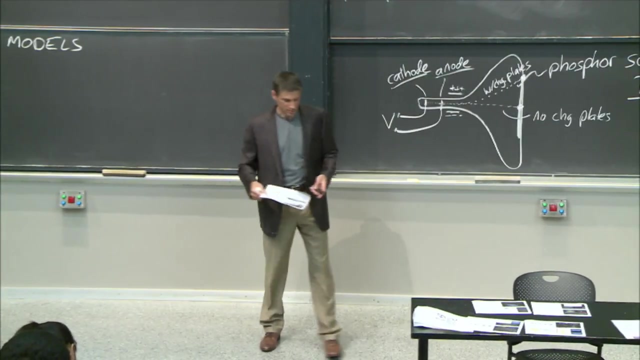 You get a little bit of deflection, And other times you'd get a signal out here or there or even right back at the radium. How is that possible? This did not work. That model of the atom did not work. 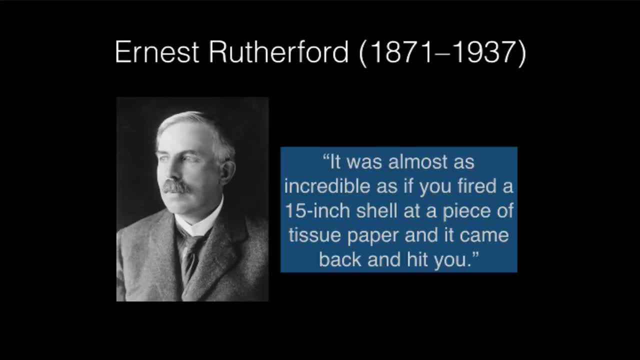 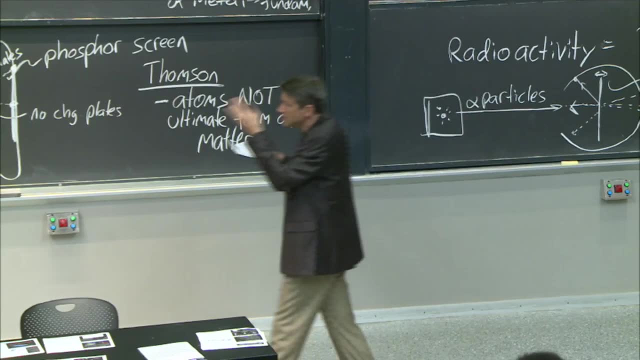 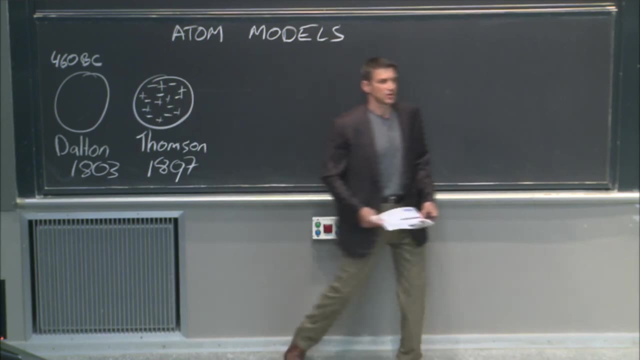 And Rutherford himself said it was almost as incredible as if you fired a 15-inch shell at a piece of tissue paper and it came back and hit you, Because they just didn't expect that a positive particle could bounce backwards off of an even distribution of charge. 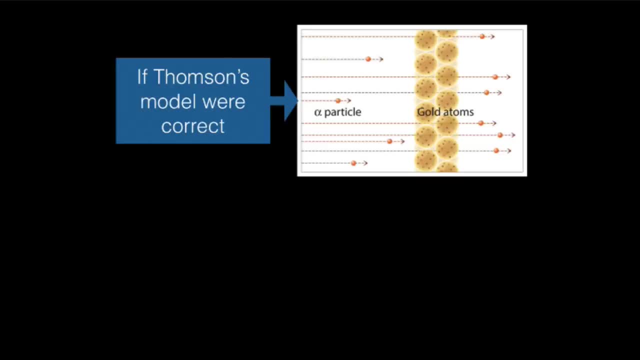 And so this is a picture from your textbook, April, that I know you are actively reading on a daily basis. So there's the alpha particles. That's what I drew, that they would expect, Or what I mentioned. they would expect it to just kind of pass through. 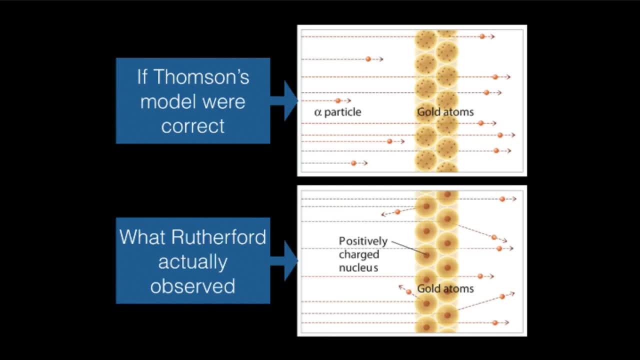 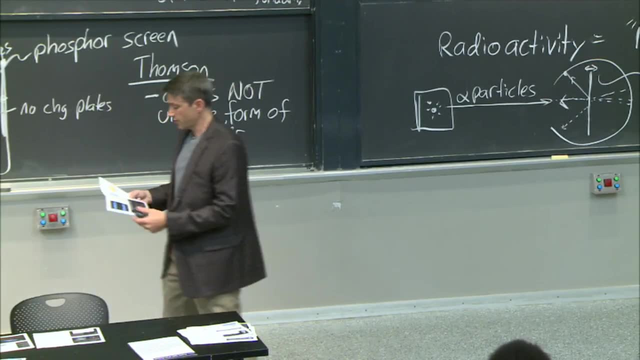 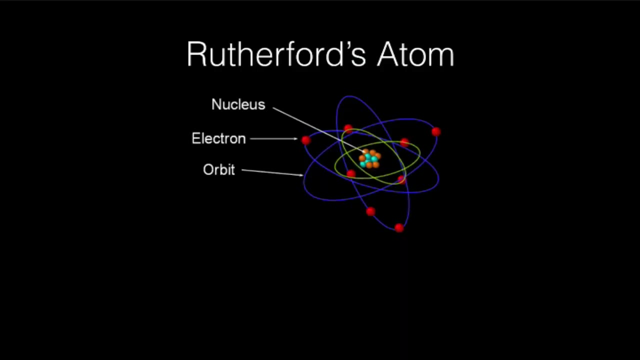 This is what was found, where they kind of come back at very sharp angles. That's what he actually observed And it led to the Rutherford atom. And the Rutherford atom was that? look, the only way that this can happen, that you get these events where? 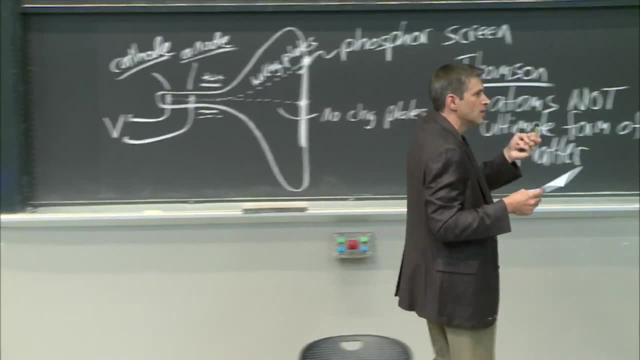 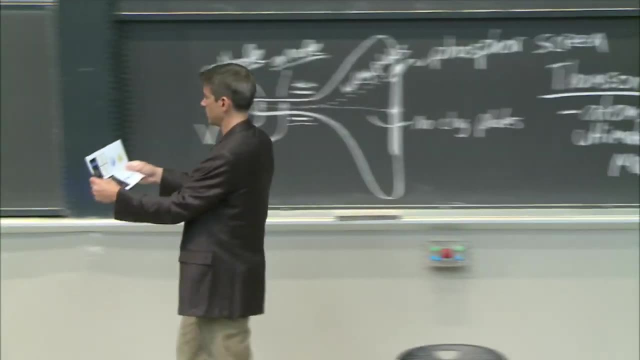 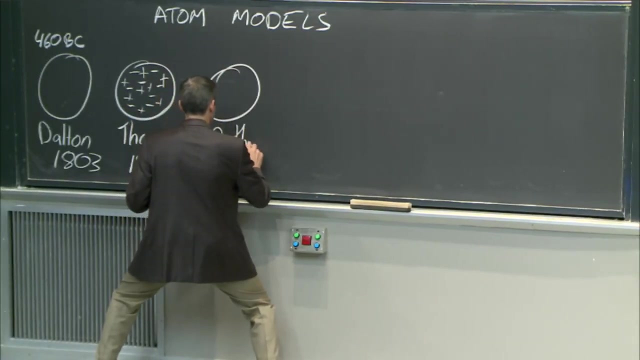 a positive charge comes back like, that is, if there's a very, very strong concentration of the positive charge in one small place. And so he said, let me see if I can read my date correctly, 1912.. And so, Rutherford, he said that the positive charge has. 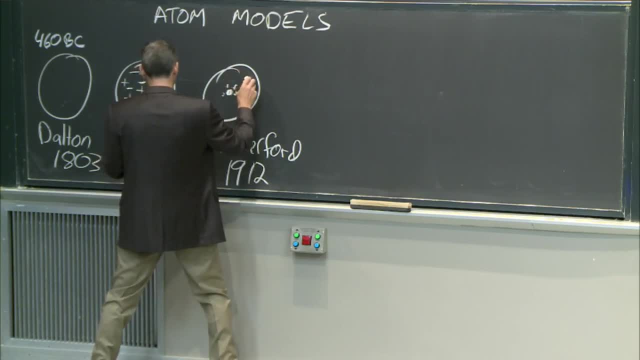 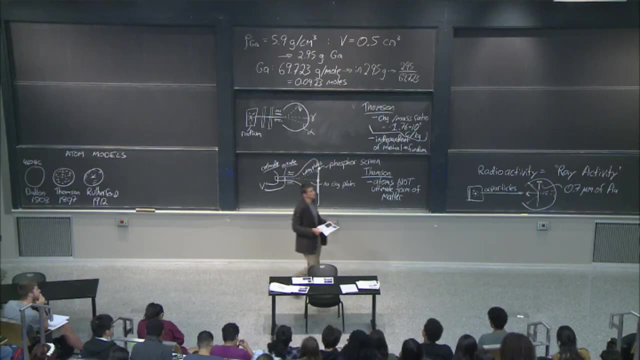 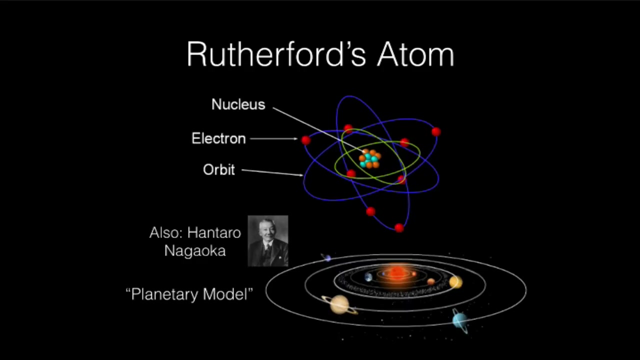 to be in the middle, and then the electrons must be far away, And that is also sometimes it was called the planetary model, And in fact it was. In fact, there was another scientist from Japan, Nagaioka, who five years earlier had predicted: 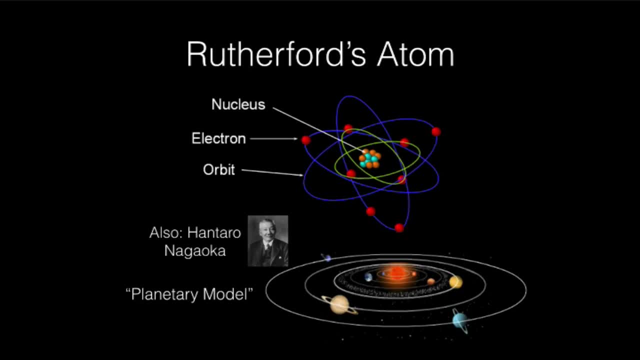 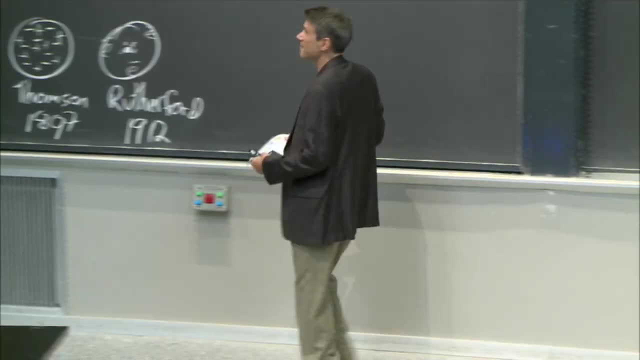 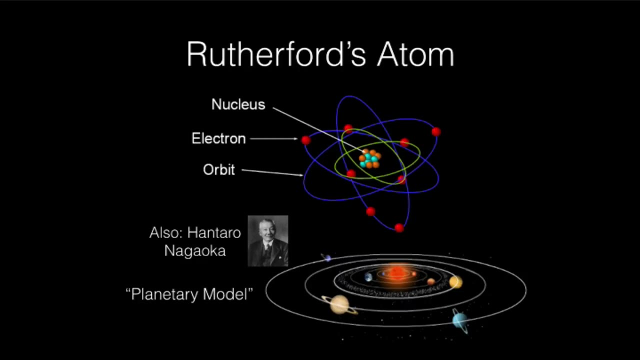 although he sort of predicted this because he loved Saturn, He really did So. he said: you know, it seems that maybe we have a Saturn situation And he called it the Saturnian model. But I want to mention it because it was part of the way there. 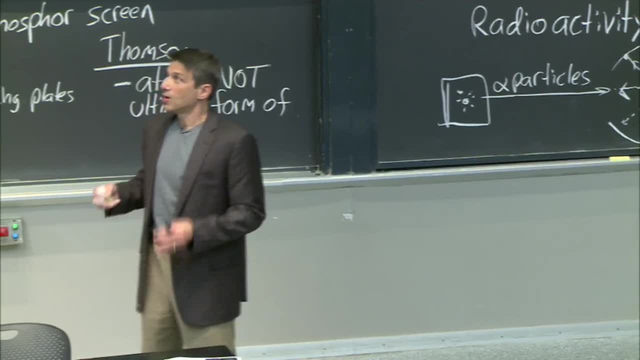 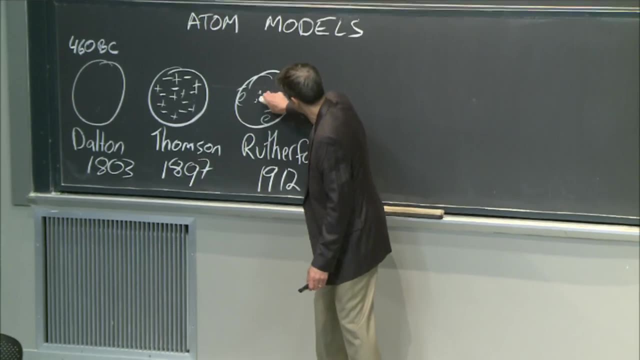 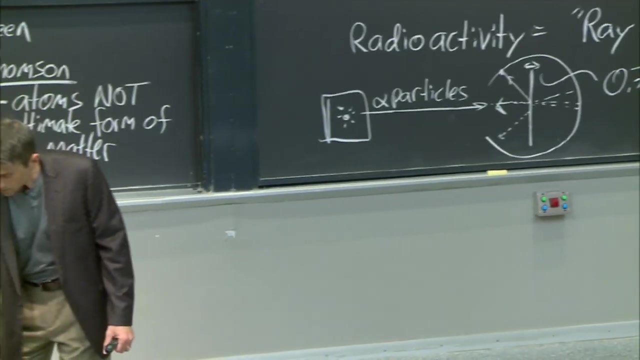 But in this planetary model which came from Rutherford's experiments, you had a very different picture now of the atom. You had a very different picture. You had all the positive charge really concentrated in the middle. Now the thing is also that the atom 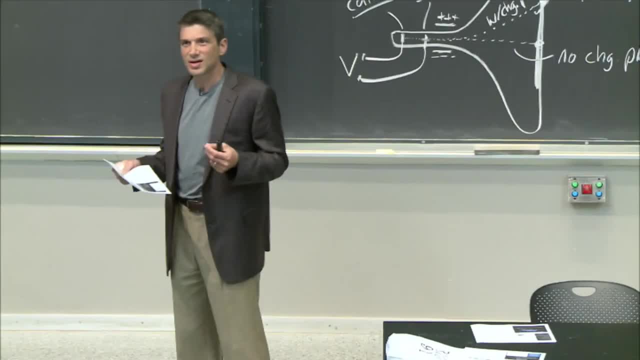 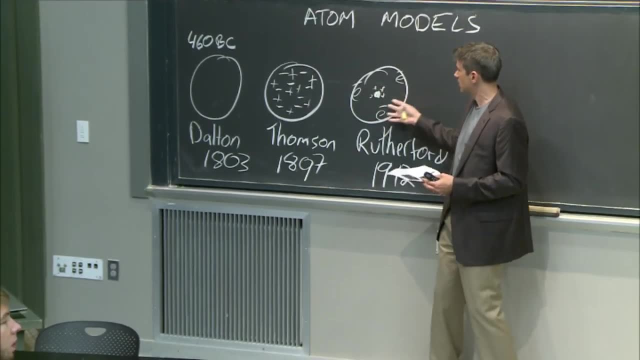 what they were starting to understand is that the atom isn't just like. there, isn't just all this space here. right, They knew the electrons weren't distributed evenly in here. They knew they were sort of far away. There's a lot of space. 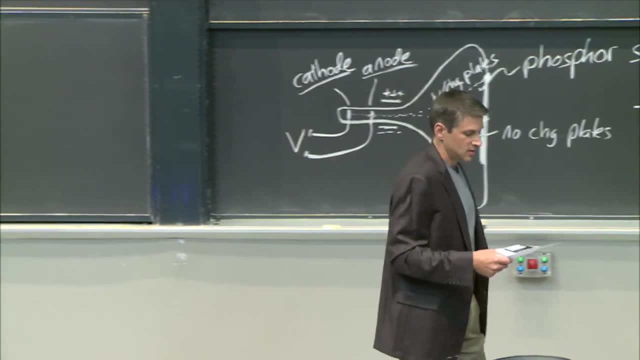 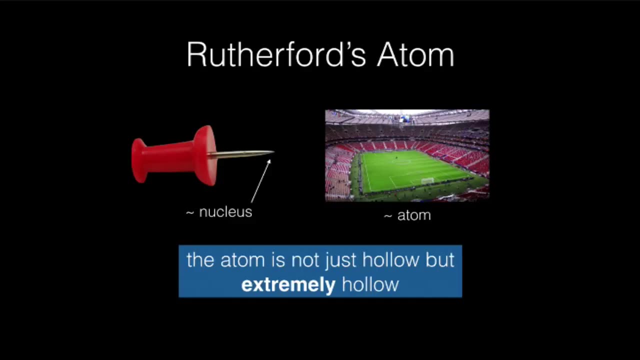 There's a lot of space. The radius of the atom is 100,000 times bigger than the radius of the nucleus, right? So just to put that in perspective, right? So here's a picture. There would be, like the nucleus, the head of a pin. 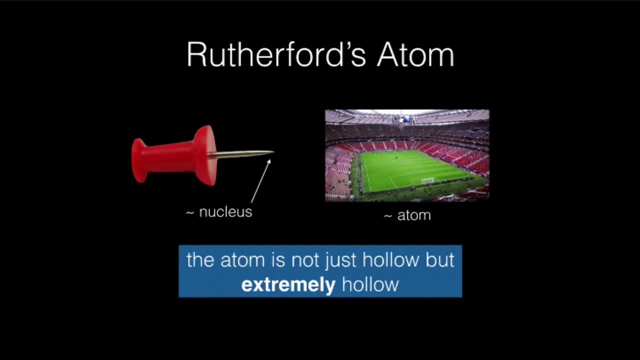 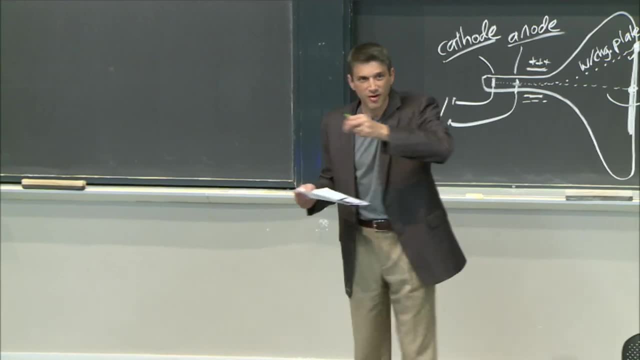 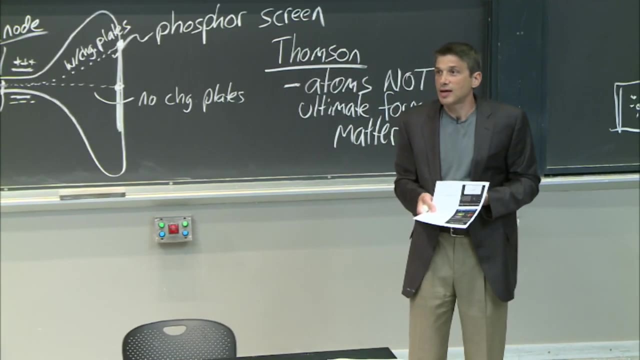 And this would be the atom, a stadium. OK, If you took all the stuff, all the stuff in a human body, that means the protons, right, All the stuff in the nuclei, the neutrons. Oh, I'm getting there. 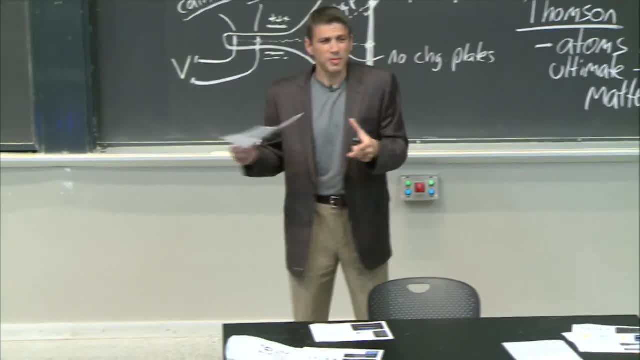 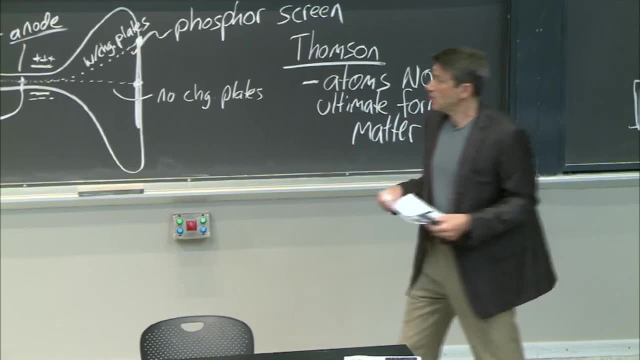 And the electrons, And you take all. you take 7 billion people and you put that all into one volume, it is the volume of a sugar cube, So you know. so things are pretty empty out there. Things are pretty empty out there. 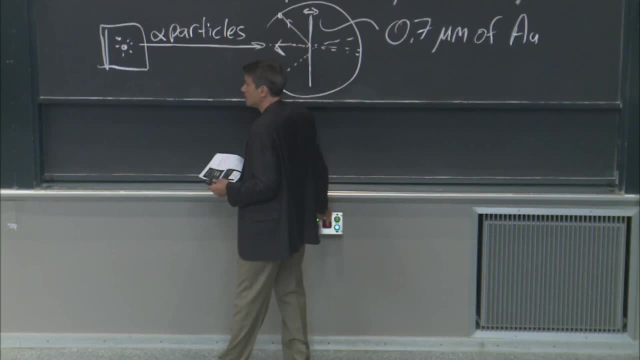 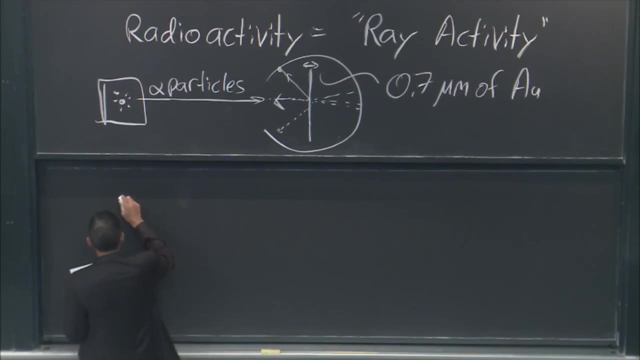 How empty are they? But this is where you find true meaning. This is deep. How empty is stuff. Look, if I weigh the universe, you know the universe itself. we're going from the atom and the electron all the way up to the universe. 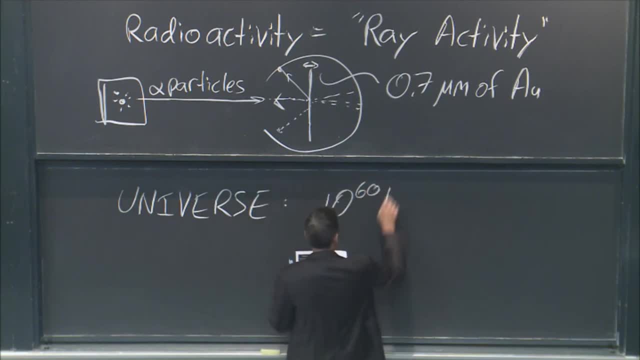 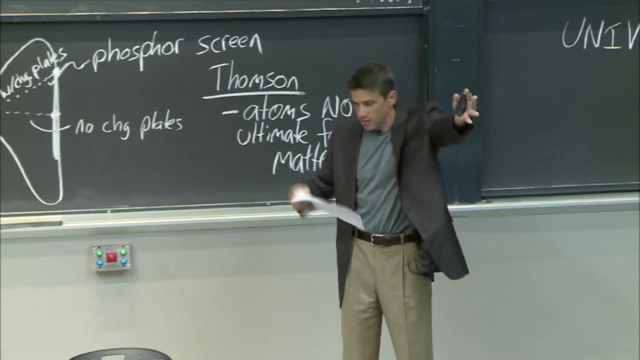 The universe weighs something like oh 10 to the 60-ish kilograms, That's over roughly 30 billion light years. OK, So if you just do the math right, so you weigh the universe, you know how big it is. 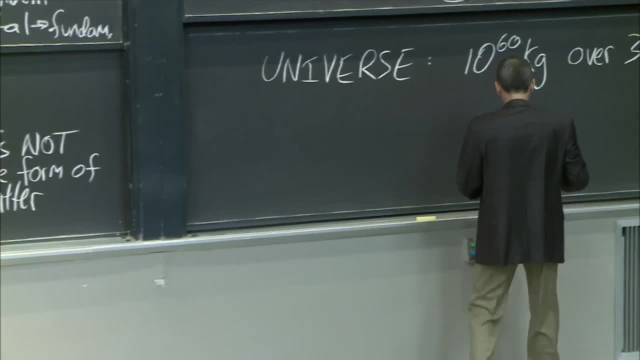 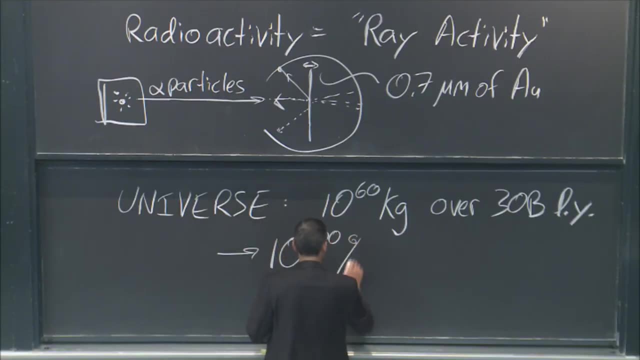 roughly plus, or you know, give or minus. plus or minus, then that means that 10 to the minus, 20% of the whole universe is stuff And the rest is empty. That's deep, Because we find meaning in all of it, don't we? 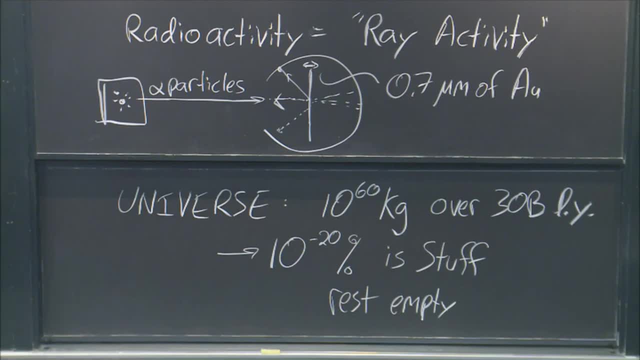 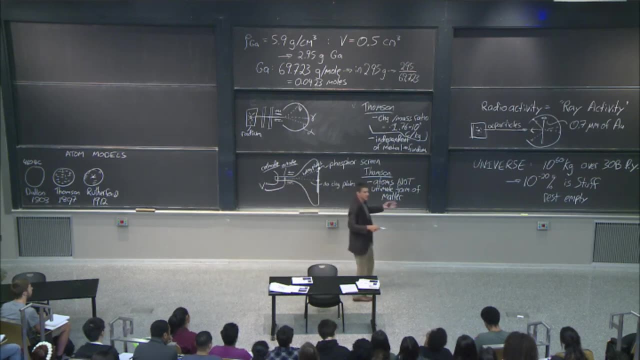 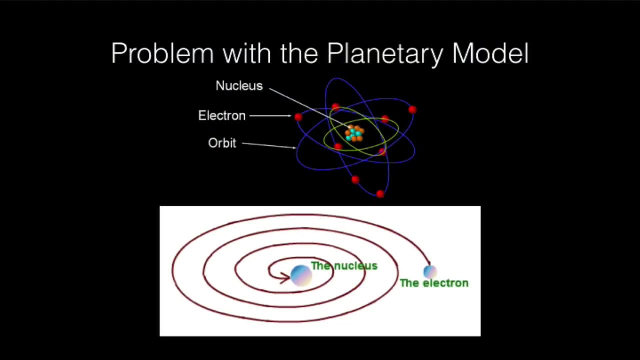 That's deep. Think about that. That's not just the universe but the atom. It's the same. You know so much of everything is nothing, OK, Planetary, But there was a problem with the planetary model. There was a big problem with the planetary model. 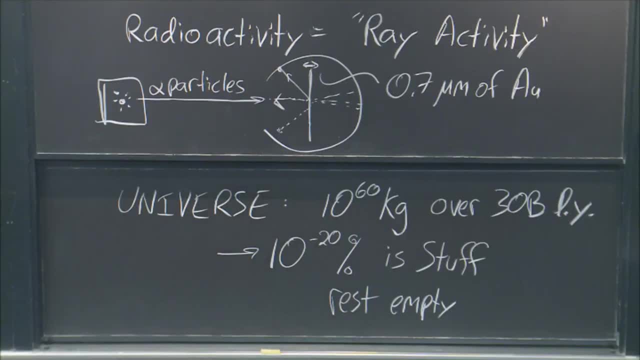 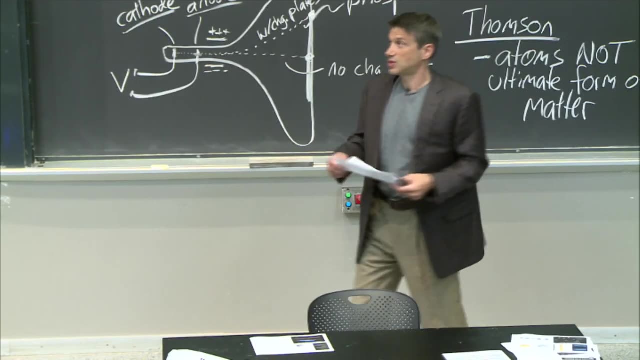 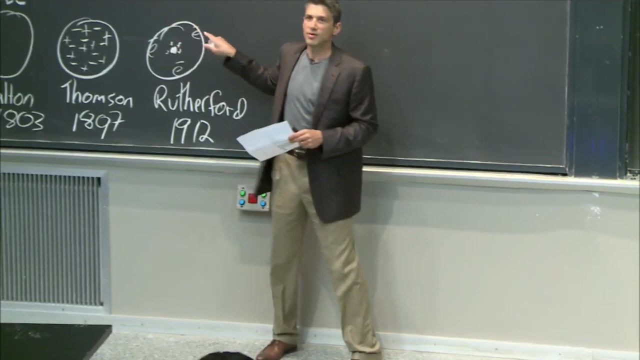 Because classical E&M told us that if a charge is accelerating, which it is because we think it's going around. We think they're going around here. They're not- Friday will know more about that, But we thought they were. 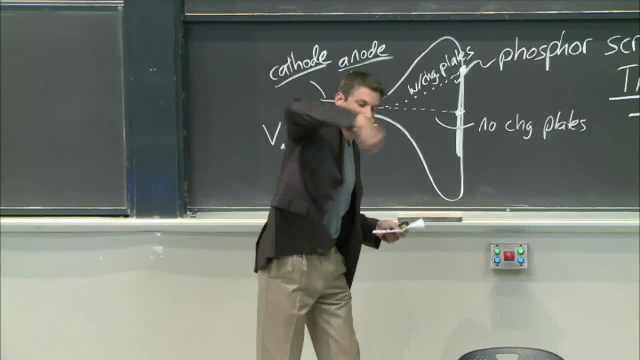 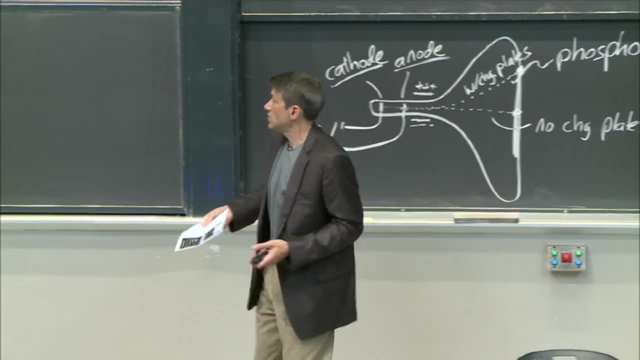 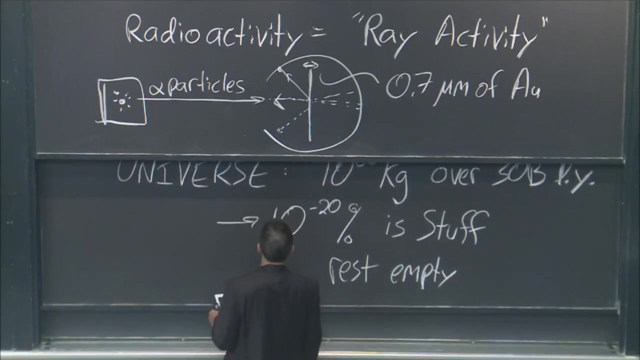 But if it's accelerating to keep the circle, then it's got to be radiating energy. That's what classical E&M tells us. An accelerating charge loses energy And if you go with that, then the electron. let's see the stability analysis that we. 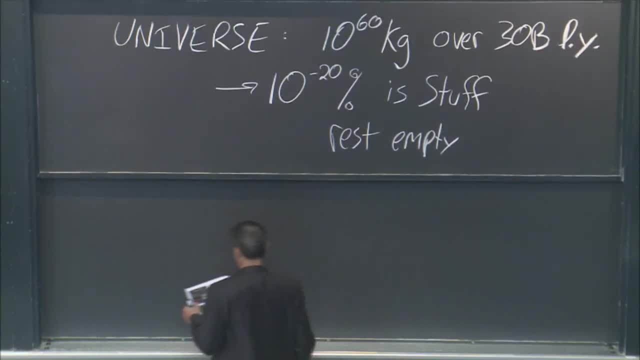 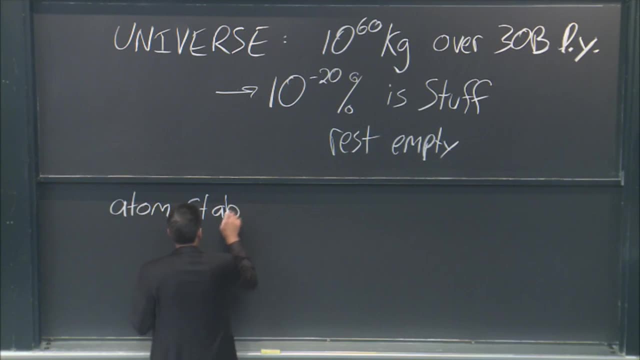 get out of something like that. hang on is that the atom would be stable for ish 10 to the minus 11 seconds. Eh, five times Roughly. That's not giving us a lot of time, Right, And so we were getting so far. 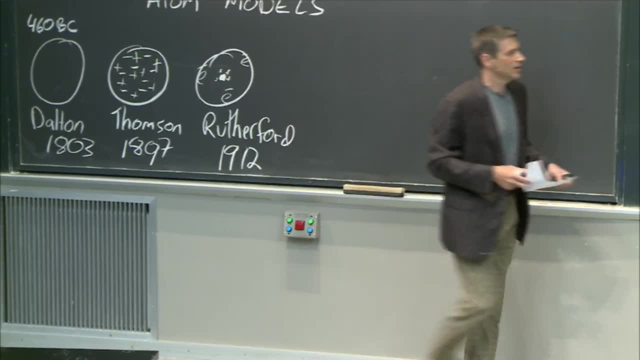 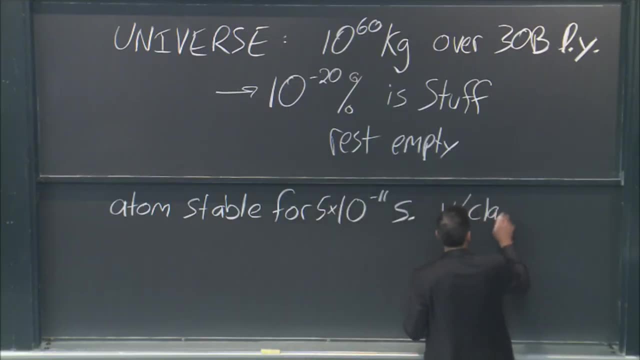 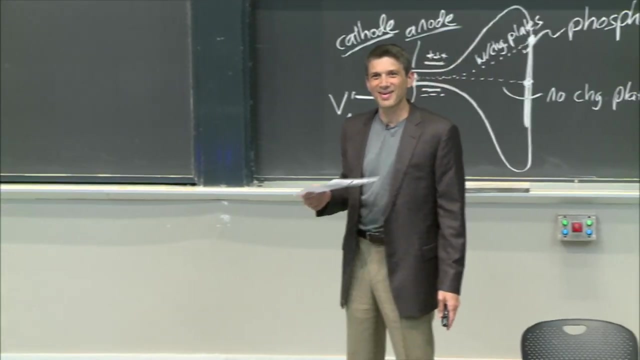 We had this great model, But it didn't go with classical E&M. So atom stable for that with classical E&M? Oh, because you know what's coming will go in quantum. Not now, I'm just preparing you. Did I hear an? oh? 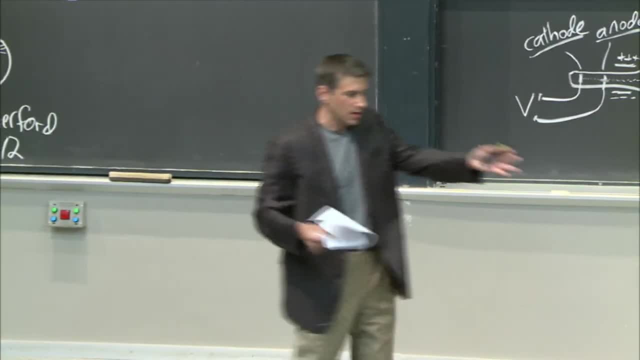 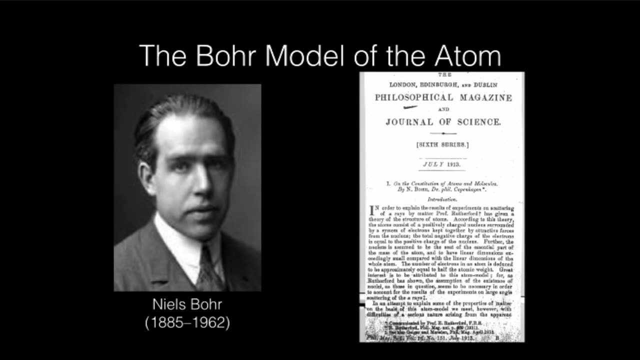 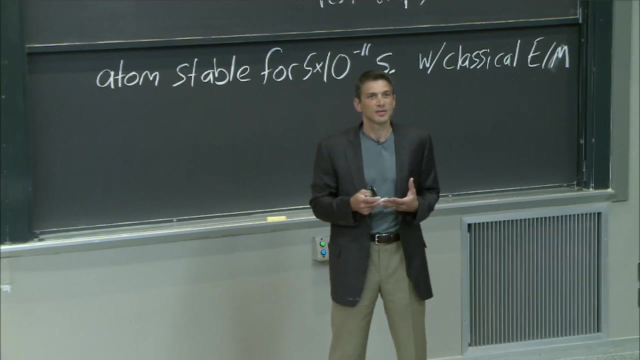 Thank you Friday: OK, So Bohr comes along, And on Wednesday we're really going to go into Bohr And we're going to talk about how Bohr's model of the atom allowed us to understand how light and matter interacts. 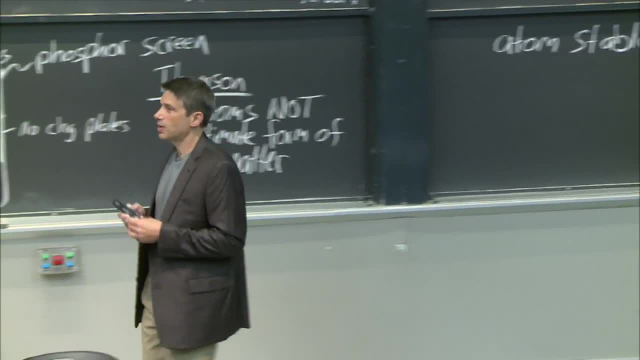 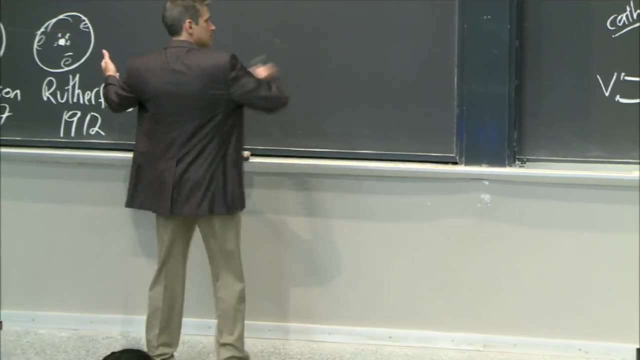 That's a big deal, Right, But we'll go into that on Wednesday. For now, I just want to tell you what he did, which is he thought about this problem a lot And he's like: this can't be. We need some way out of this. 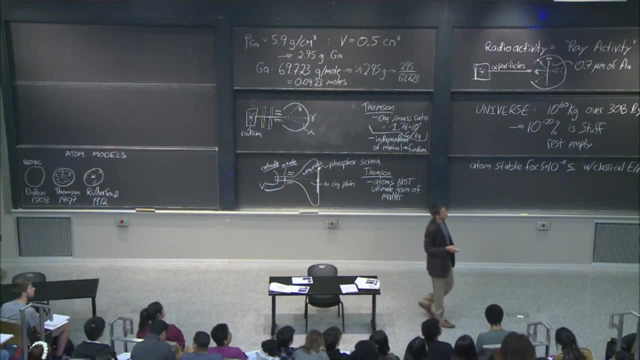 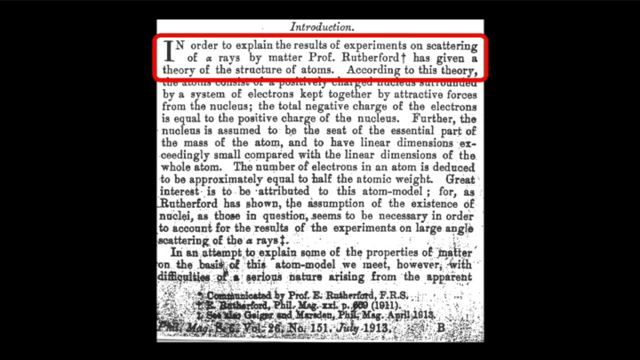 And he wrote this paper where he said the following: Oh, he said, let's go over here. He said, OK, in order to explain the results of experiments on scattering of alpha rays. we just did that: scattering of alpha rays by matter. 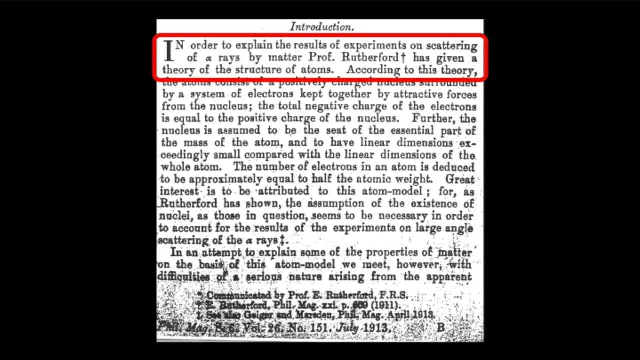 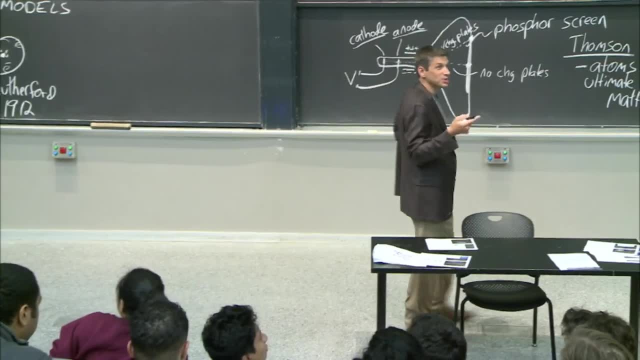 Professor Rutherford has given a theory of the structure of atoms, And then Bohr goes on And he says great interest is to be attributed to this atom model. Now that is a serious diss. Great interest- If somebody calls your model of great interest. 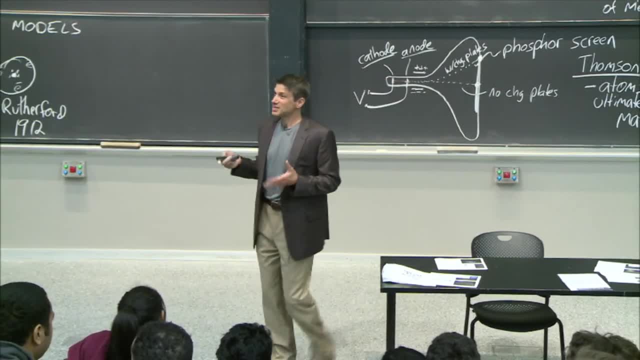 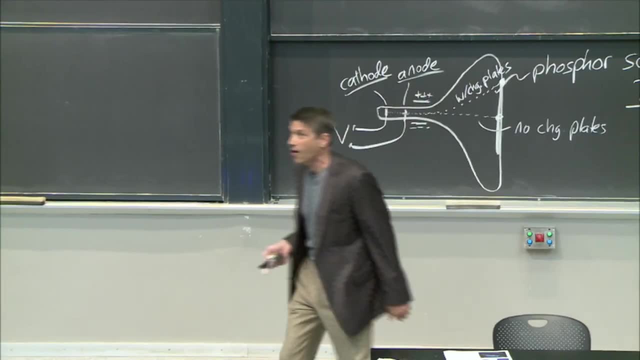 you know you're in trouble. That's basically he might as well have said back then: you know, this model is of great interest because it's totally wrong, And if you want to know what's up, come over to me and I'll tell you. 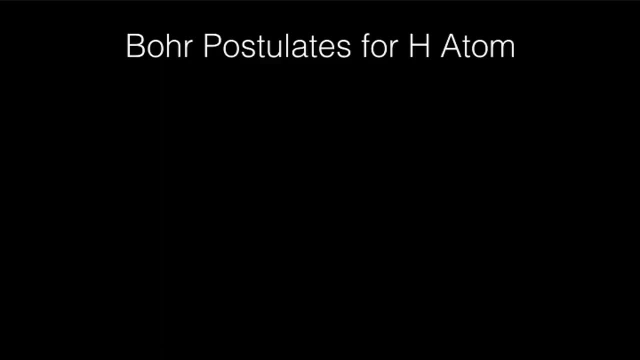 And that's what Bohr helped with in his work. And what he did is he wrote down some postulates. He said: look, the Rutherford atom is correct, But the problem here is classical E&M theory. You cannot apply classical E&M theory. 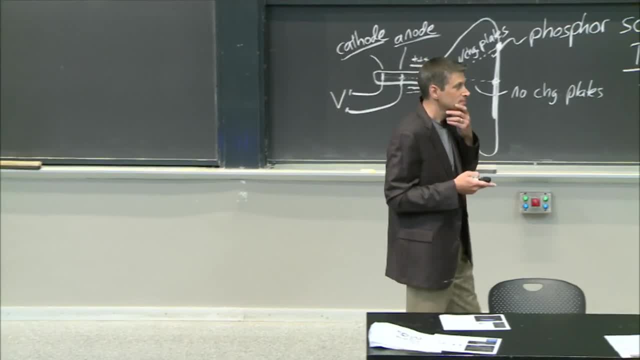 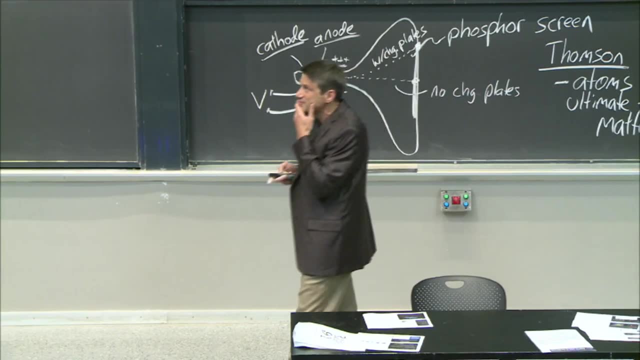 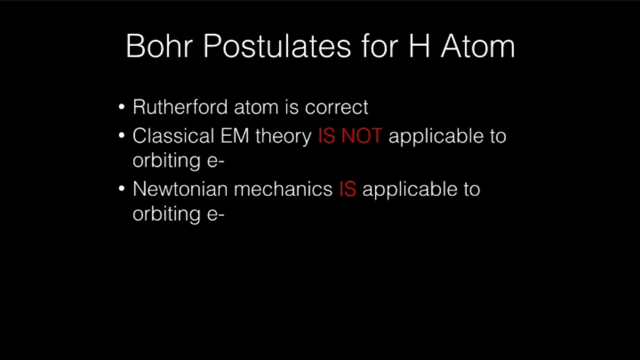 to the orbiting electron? You can't, because that's what happens. So something's wrong with literally nothing less than classical physics. Right, He said Newtonian mechanics still works. Right, Newtonian mechanics works, but not E&M. So he said we can go classical on how things are moving. 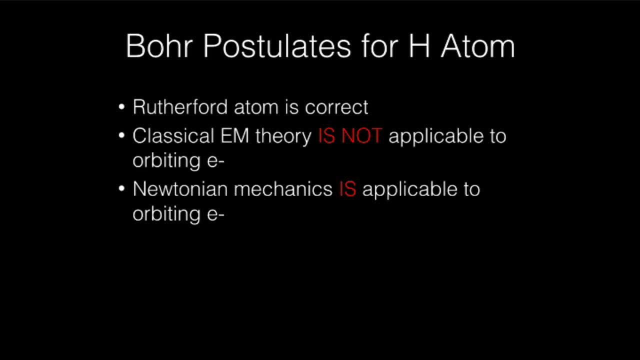 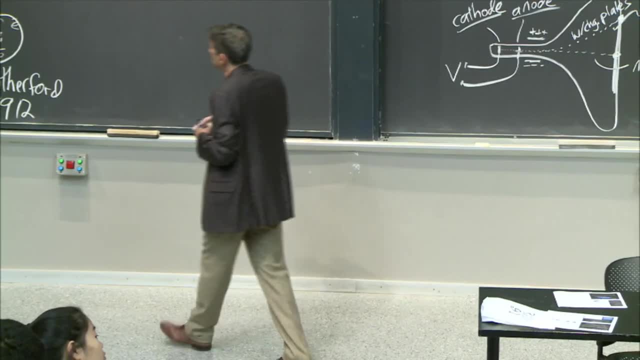 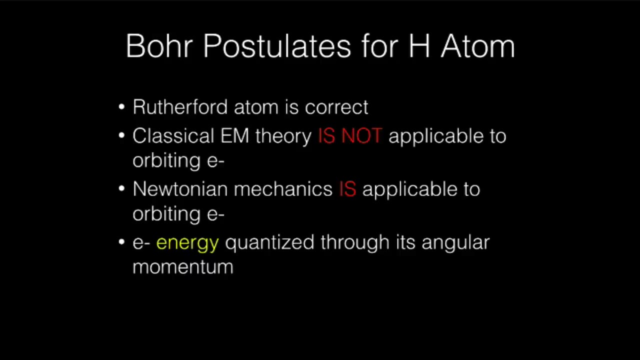 around F equals ma stuff, but not E&M. He also postulated that the energy of these electrons, the energy that these electrons sit at or have- we'll get into this a lot- he hypothesized that that's quantized, Quantized. 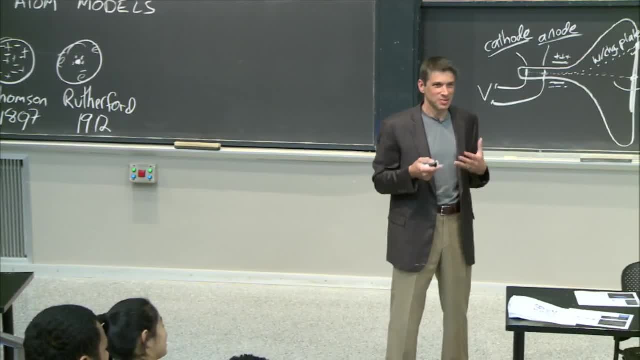 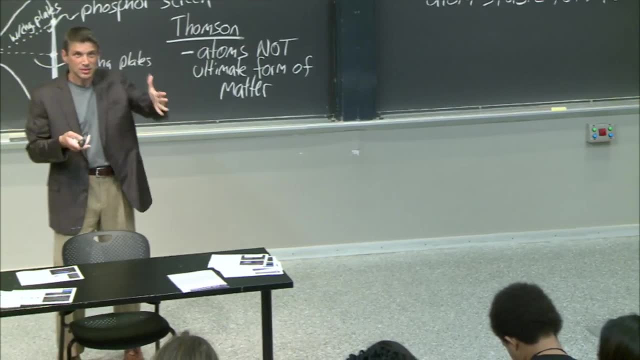 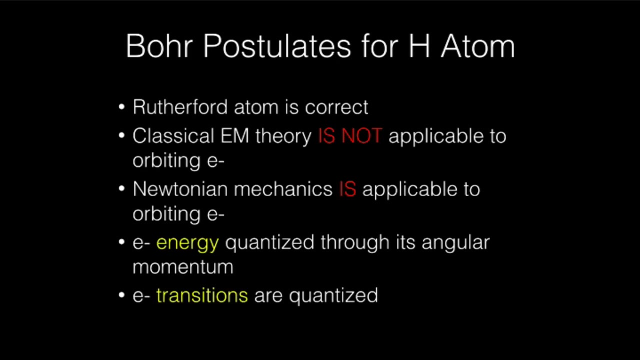 Quantized. We're saying that word. It's a beautiful moment. Quantized. Quantized means that it could only have certain values, Certain values, Which means that if this electron were to be in one value and then change into another, that the transitions 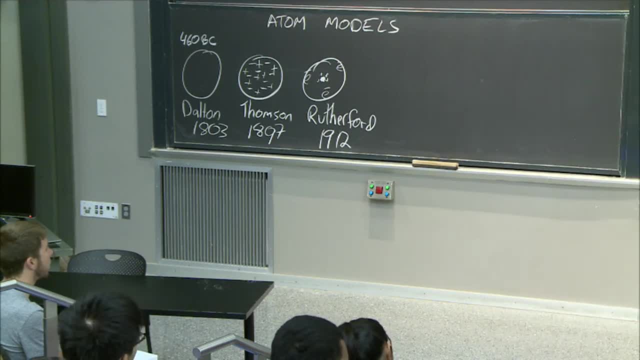 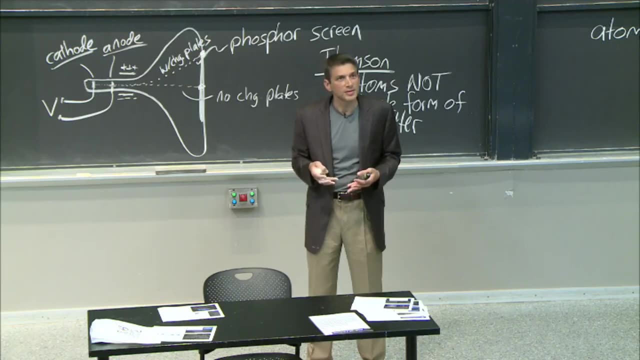 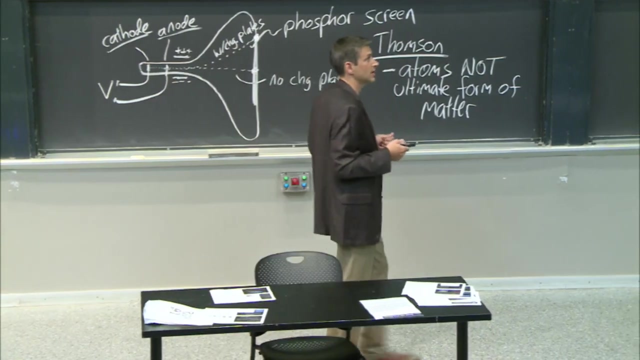 are quantized. The transitions of an electron from one energy level of the atom to another, To another, can only have certain values, And that is what we get from the Bohr model, And boy did it explain things. That's going to be the subject of Wednesday, as I mentioned. 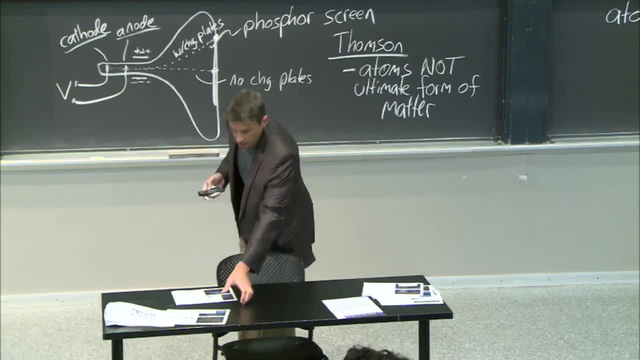 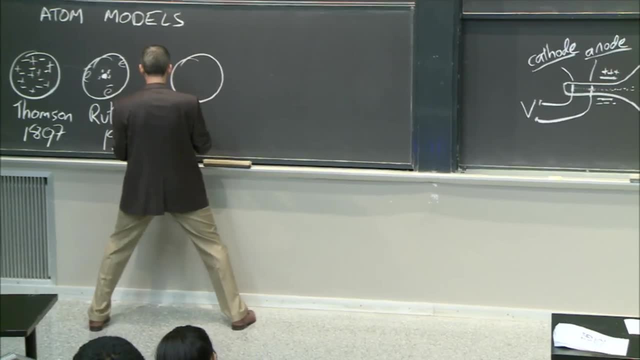 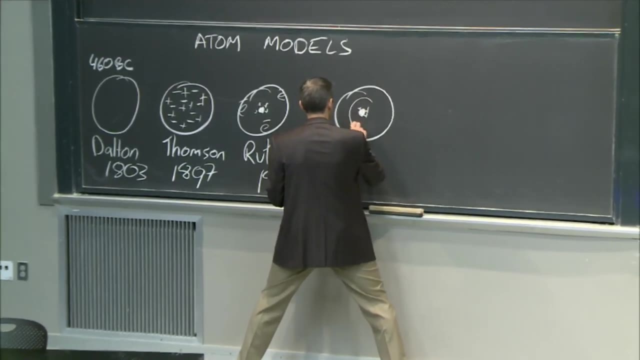 Right. But this gets us to the Bohr model. And here's Bohr, where now- oh, I got to draw this- We got all the positive charge in the middle. These electrons can only have certain radii, certain energies. 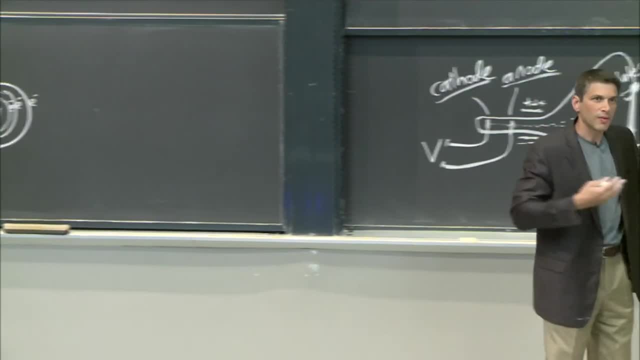 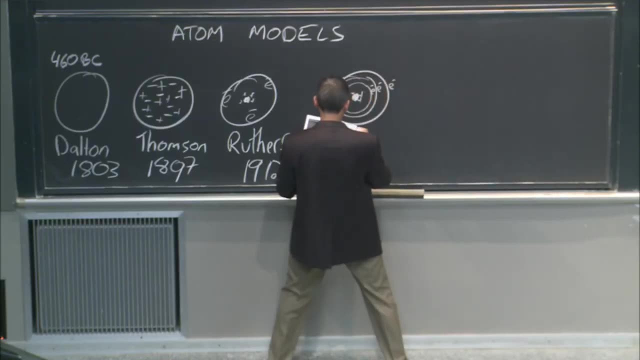 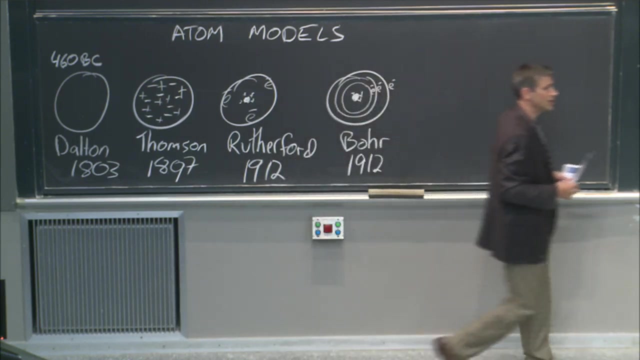 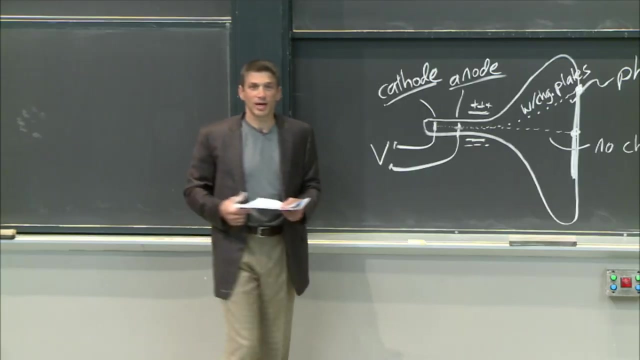 They cannot continuously roam around. They can't. They're quantized. That's the Bohr model And this is 1912.. This is closing in on the last and final model which we'll get to this week, which is where quantum mechanics comes in. 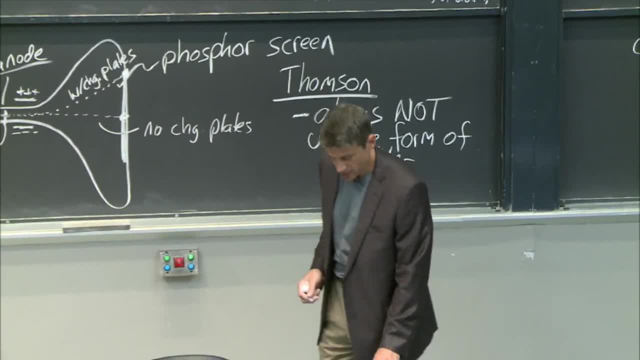 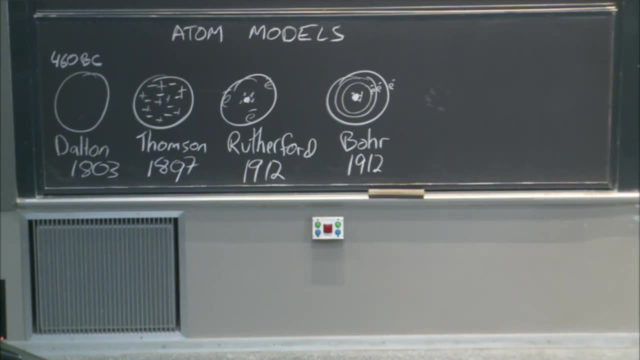 OK, Now we got one more thing to talk about. So this is where we're going. We're building up the full understanding of the atom. But there's one more thing that I got to come back to, And that is that. look, we just said: 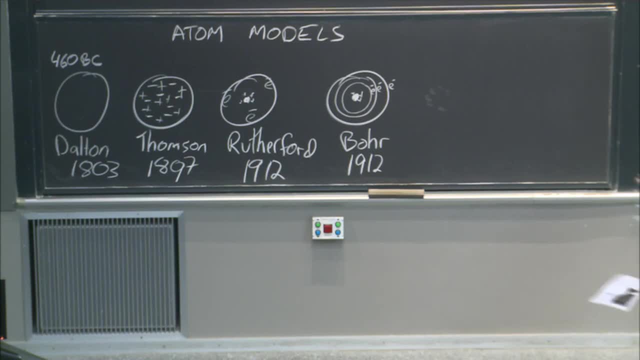 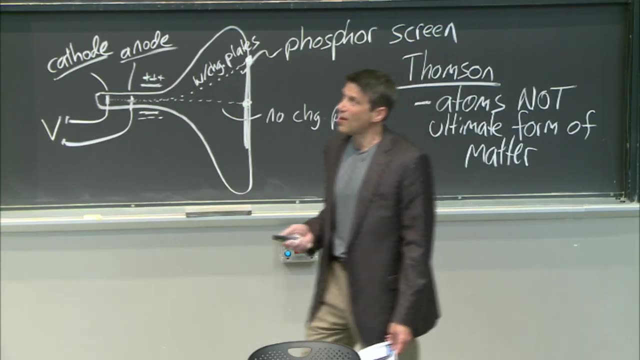 there are these positive charges in there and these negative charges out there, But it turns out that atoms can have different masses and stay neutral, All right. So we're now in a position to talk about this thing that we've been calling the nucleus, and the fact. 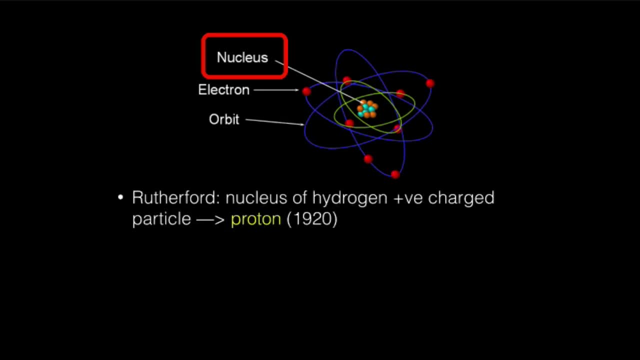 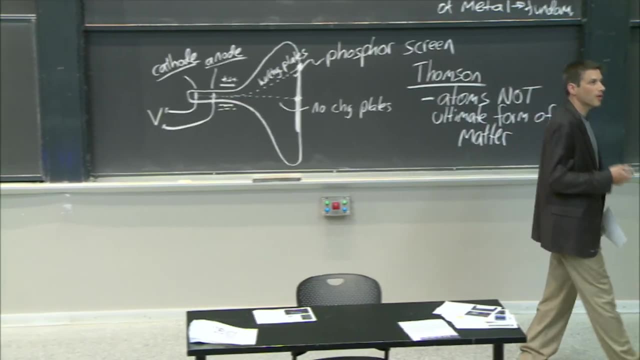 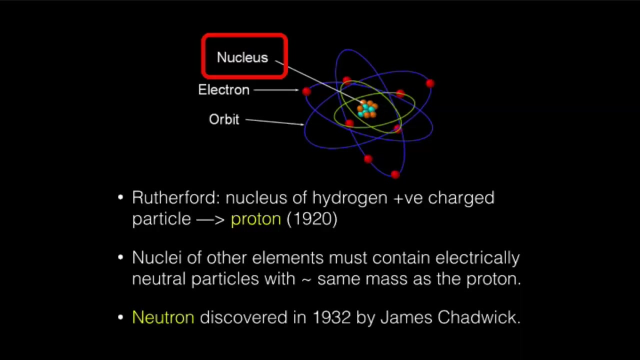 that it's not just protons. We're in a position to talk about that, And so Rutherford gave us this idea of the proton, the particle, the proton, And it wasn't until 12 years later that Chadwick found the neutron. 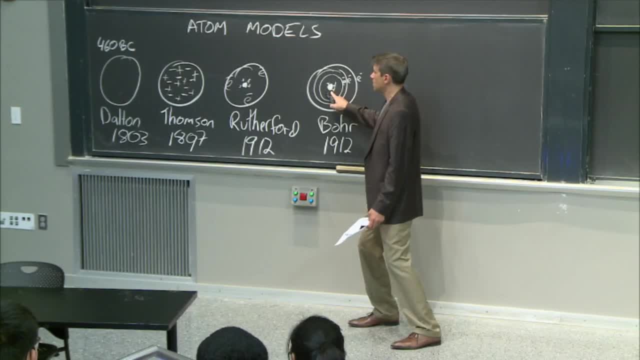 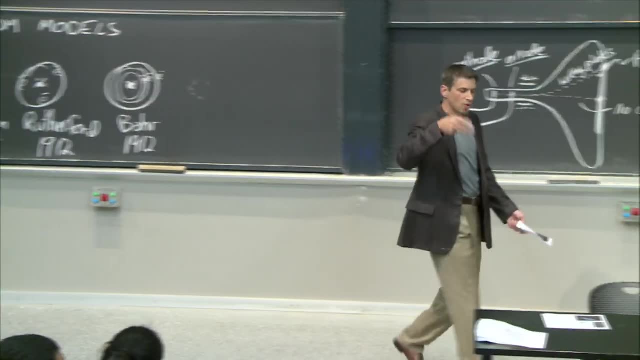 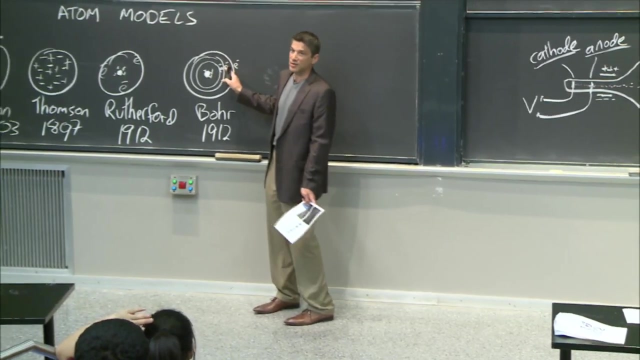 What the neutron does is: it adds mass to the atom. See, the mass didn't work. So again, if you know what the mass of the proton is, then you can add it up And you got the mass of the electron, although it's like 1,000th as much. 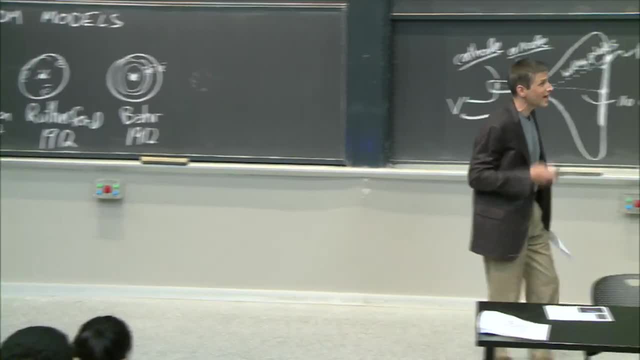 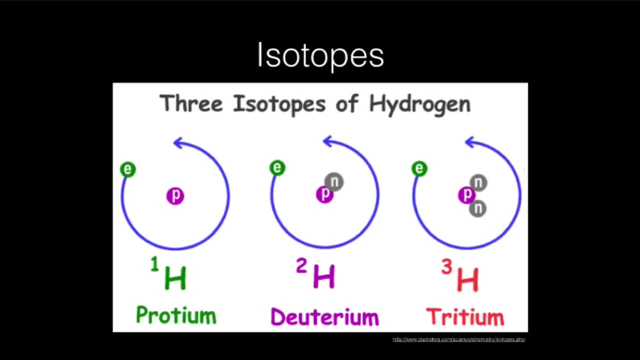 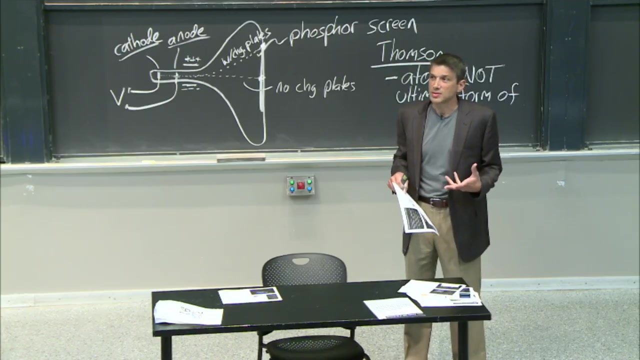 But it doesn't work. There's something else in there that's adding mass, But it's not adding charge, because these things are electrically neutral. So those other particles are called neutrons And what it does is it gives us ranges of masses for the atoms. 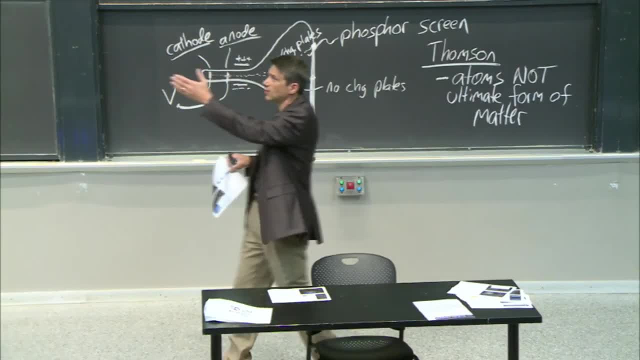 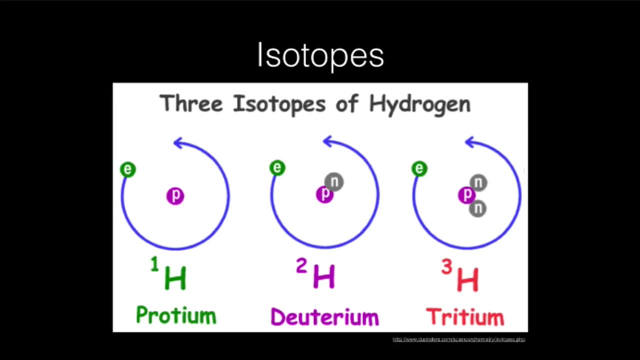 It gives us ranges Because hydrogen- now we might think about it. 99.99% of all hydrogen is just that thing on the left, a proton and an electron, But sometimes it has a neutron, So it weighs more. It's still got neutral charge. 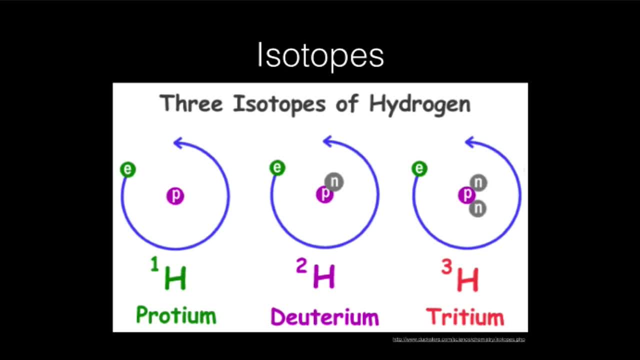 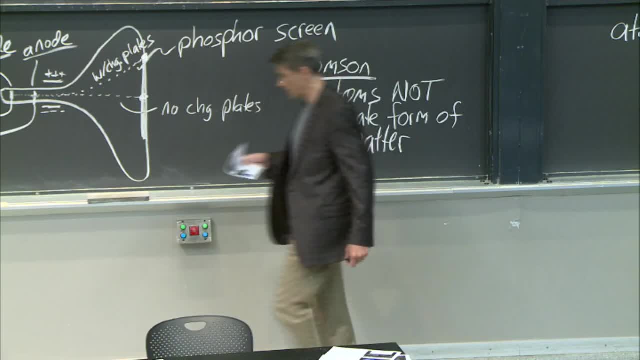 It's called deuterium. And then you've got tritium, which isn't stable. You can make it And these are called isotopes. As many of you, I'm sure, already know, these are called isotopes. 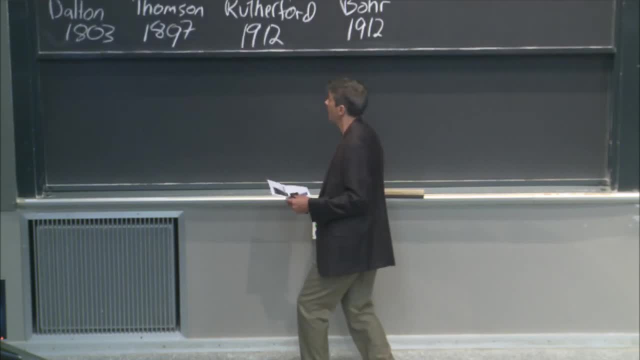 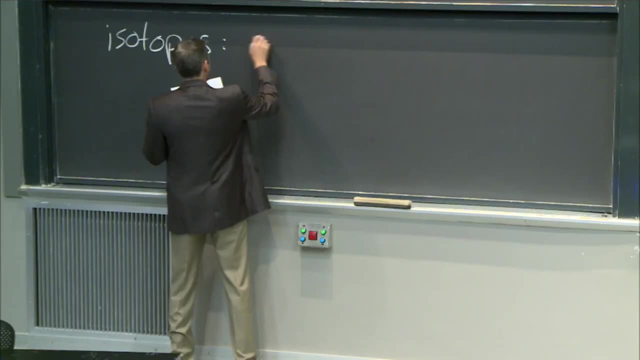 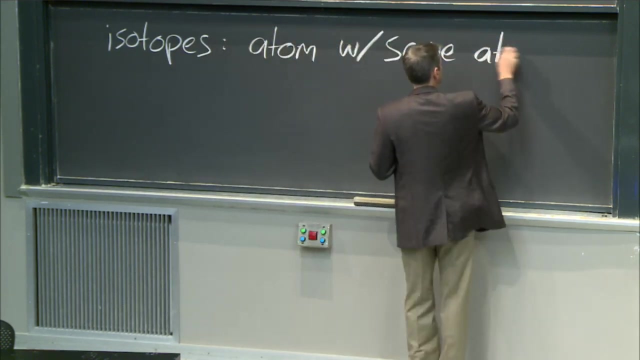 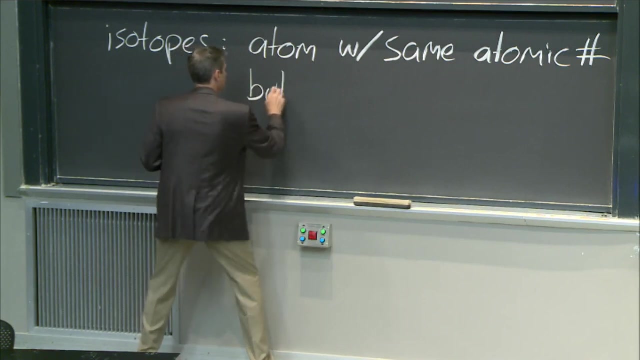 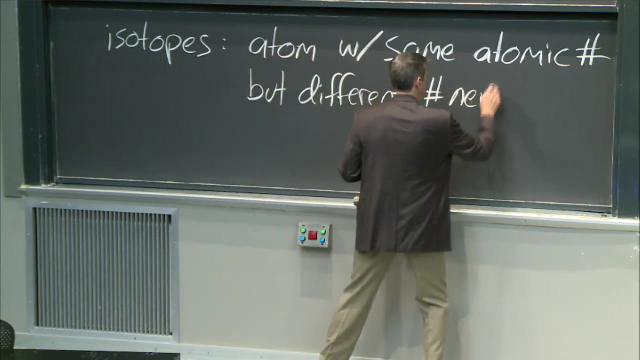 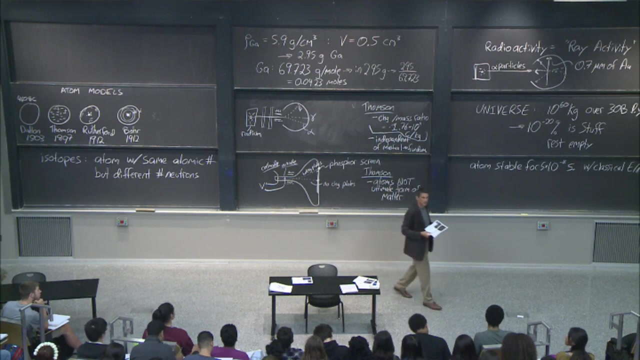 And so the isotopes of an atom. the isotopes have atom with the same atomic number, different number of neutrons, different number of neutrons. So atoms have these three things in them. They've got the neutrons, the protons and the electrons. 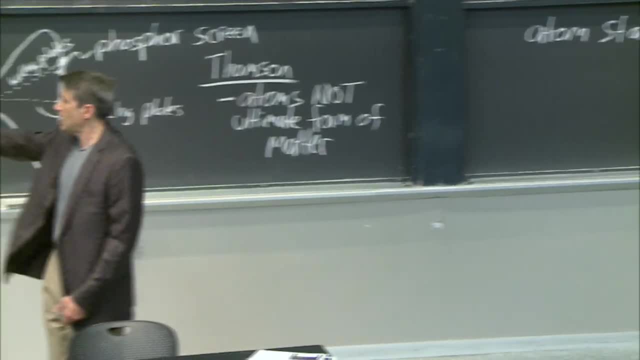 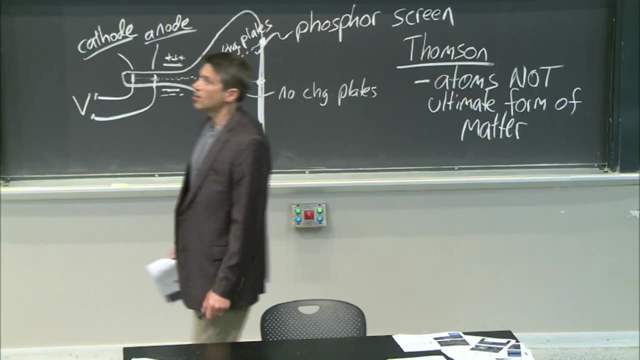 We've been talking today about the protons and the electrons, But they've got to have these other things in them where the mass doesn't work, And so if you look at something like carbon, you see the same thing. And now I want to get into how these things are written. 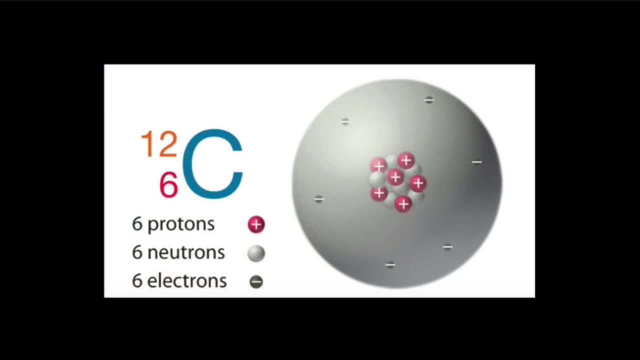 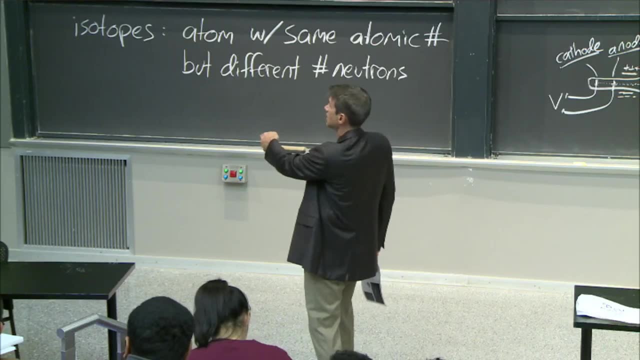 Right, So here's carbon And there are those electrons. They're now put out there. OK, we didn't draw a circle, So maybe this is around Rutherford's time when Averill made this picture. And there's the pluses. 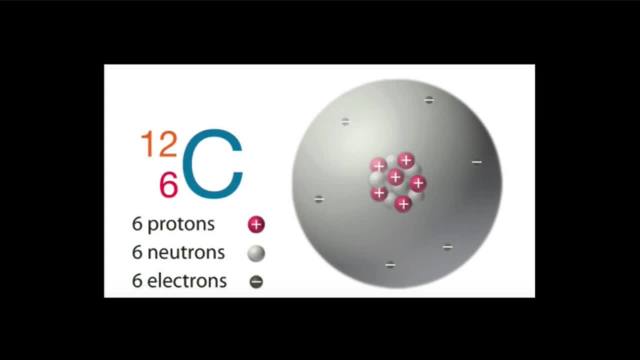 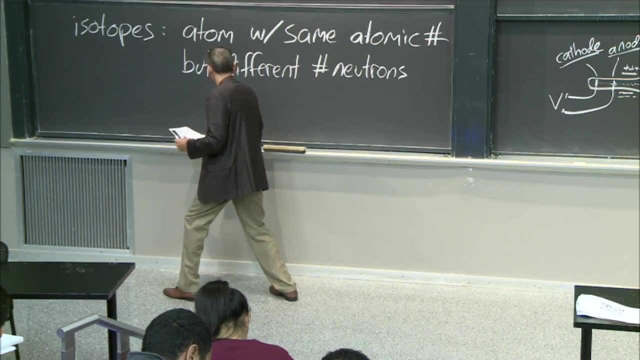 And there's other things in there, And those are the neutrons, And so what we do is we have a nomenclature for this, which is the standard, And that is that if we write an element like this, this would be the element. 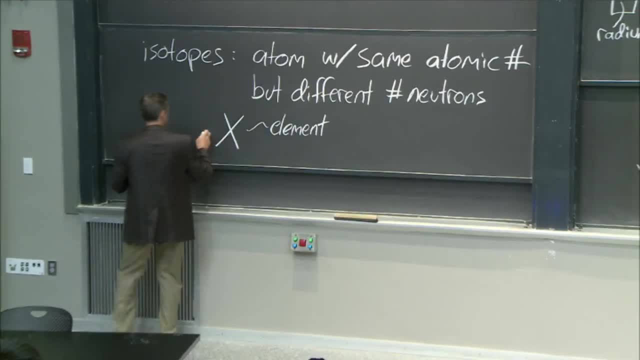 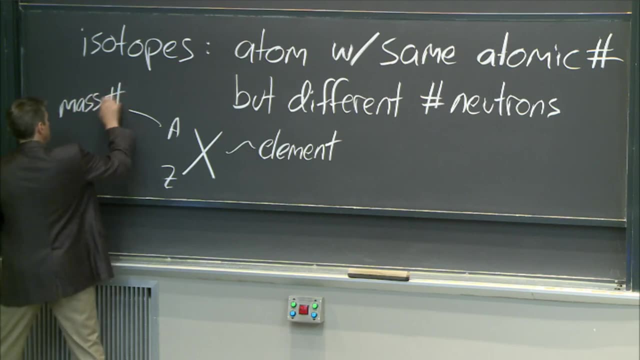 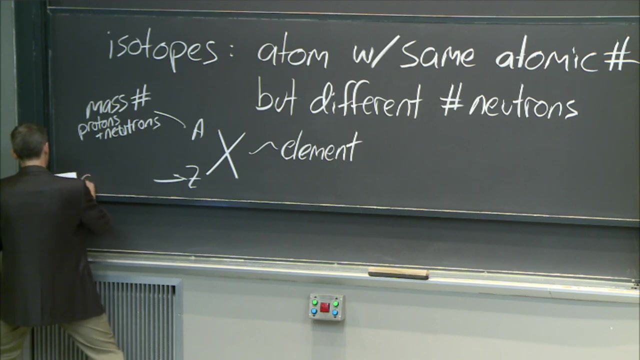 And we put something here and something here. This is the mass number. OK, So that's protons plus neutrons, Ah, Neutrons, And this is called the atomic number. Now, the atomic number, I've been referencing this thing, this atomic number. 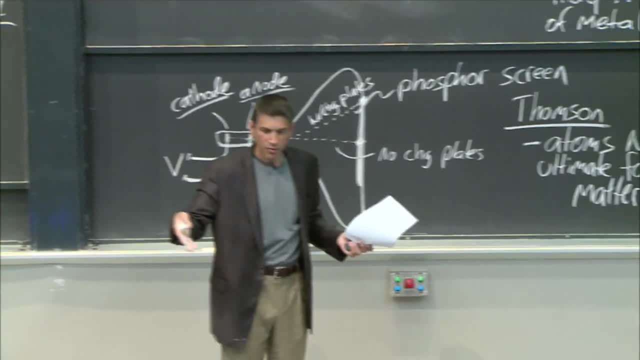 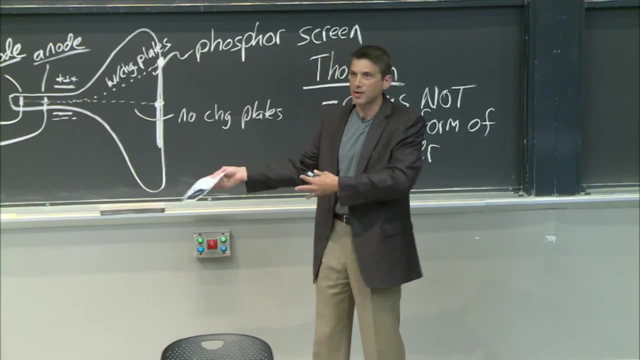 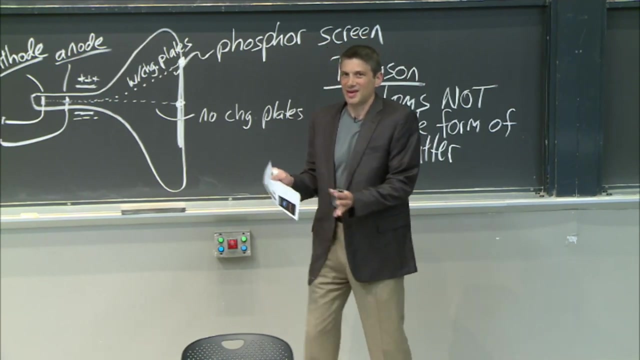 I said Mendeleev and many others. they put things in order of atomic number, maybe mass. sometimes Mendeleev did the thing where he did those things in properties Right, The atomic number was just a number until later And once we discover another type of ray, x-rays. 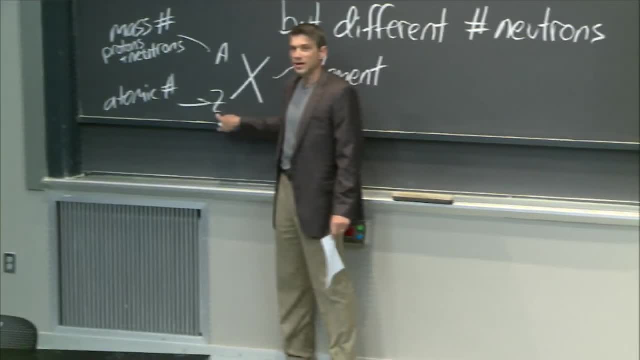 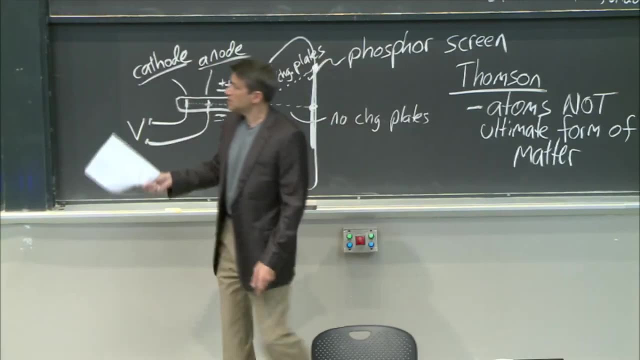 then this has real physical meaning, Right, But right now it's still just a number. It's just a number of the element in the periodic table, Right, But that mass number tells me how many neutrons I have and what the isotope is. 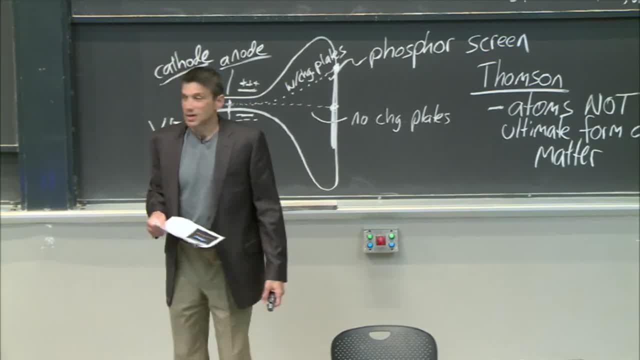 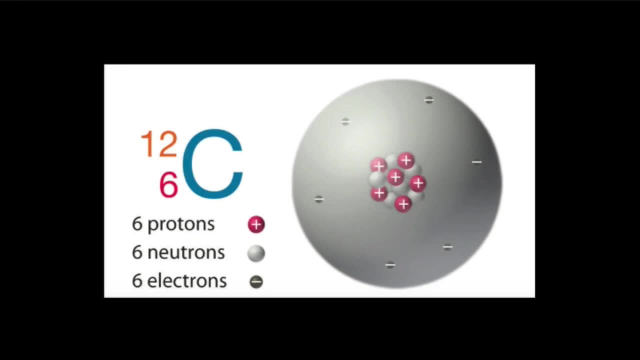 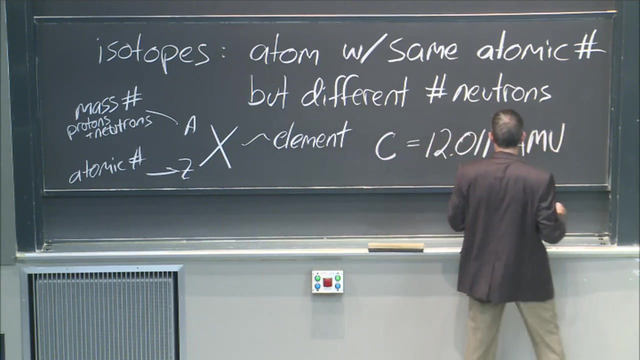 So now I go back, I can go back and I can look at carbon. Oh, by the way, carbon. I wanted to write this down before I say that: Carbon. when you look it up in the table, you have 12.011 amu, or grams per mole. 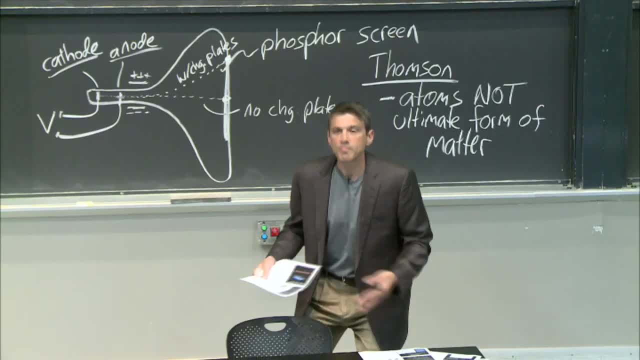 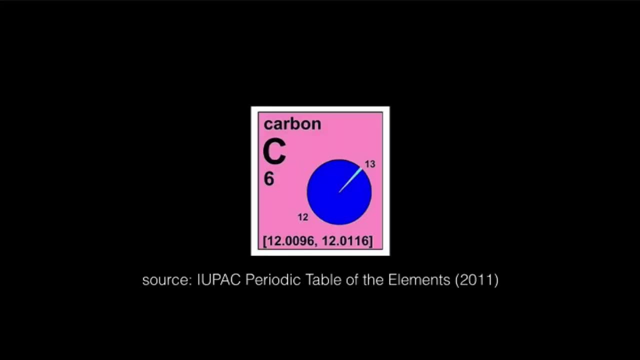 That's what's in the table. But now you know why? because it's just an average And in fact the IUPAC, which is a rocking body of the International Union of Pure and Applied Chemistry- I'm sure you've seen them on the feeds- 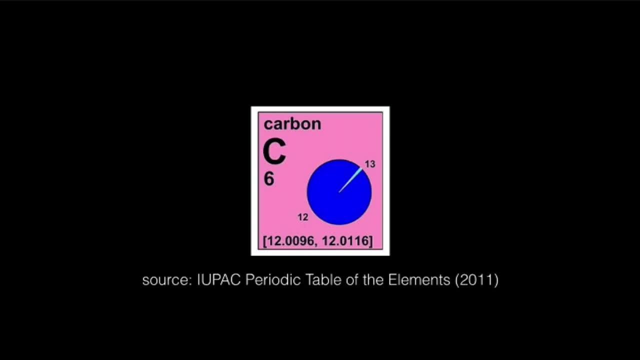 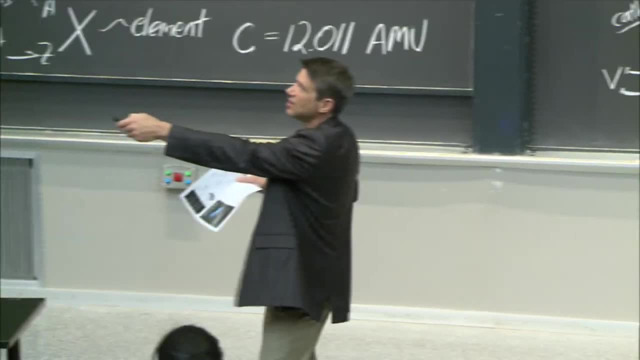 they hold meetings And, in Vienna, a nonstop night of intense meeting and partying, And they said, hey, maybe in 2011,. maybe we should actually do this with the periodic table, just to show that actually there really is a range. 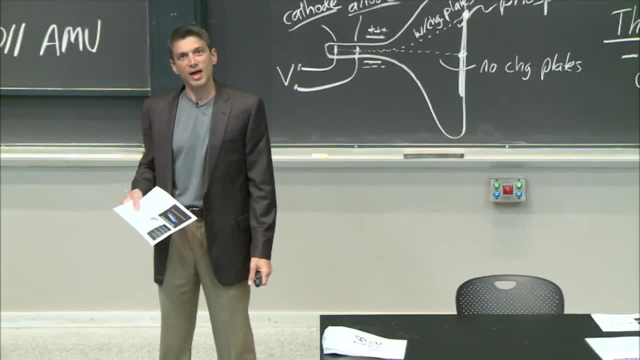 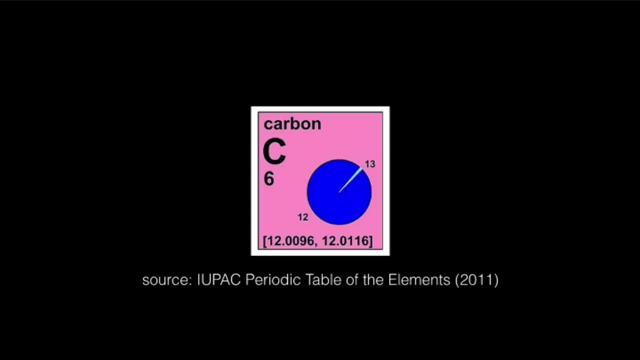 If I did carbon out of the ground here or carbon out of the ground there, maybe they have different amus Right. These are averages And there are ranges, So they're actually talking about different ways of even putting this into periodic tables. 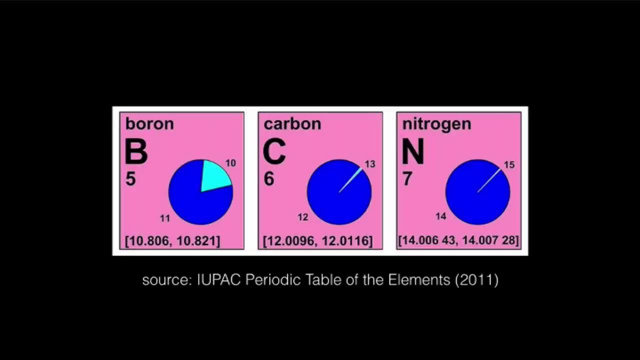 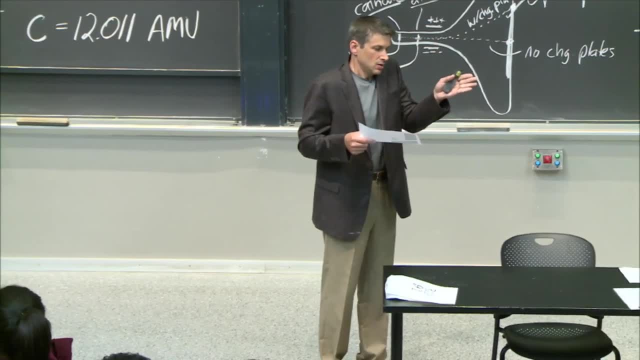 And this gets us to: oh, there's boron and nitrogen ranges, Right, But what we do, now at least, is we just look at the one number, because that's sort of averaged over basically anywhere you can dig this stuff up. 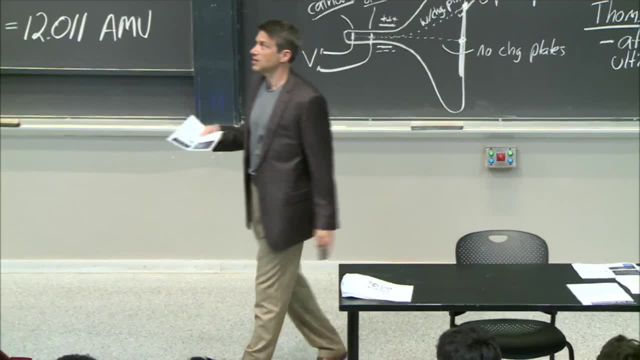 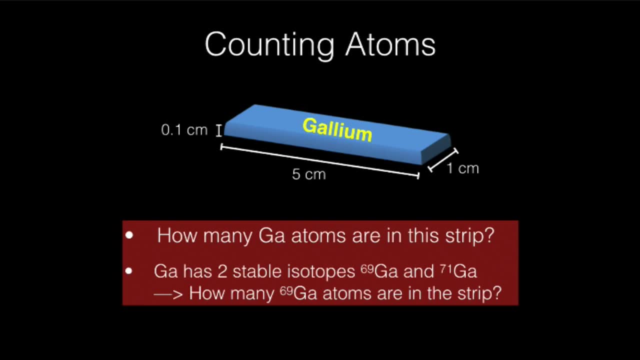 and the stable isotopes, Stable isotopes. And it gets me to my last slide, which just comes back to the beginning, as I promised, Because now I can say not only how many gallium atoms are in this strip, but I can tell you. 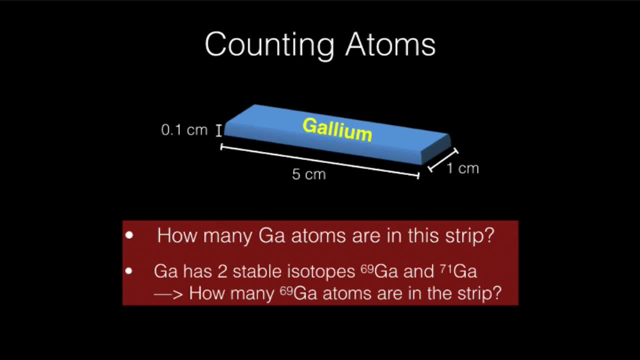 gallium has two stable isotopes. By the way, it's got a bunch of unstable ones, but it's got two stable ones: gallium 69 and gallium 71. And I can now ask you how many gallium 69? 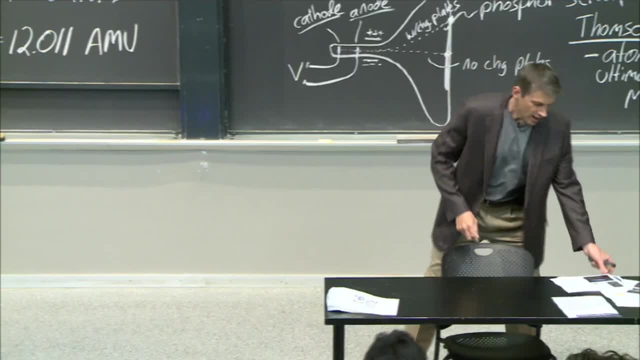 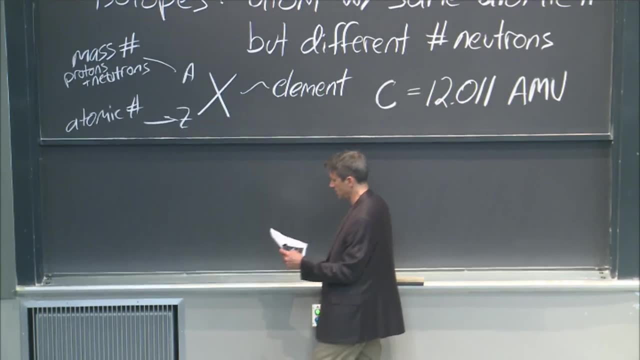 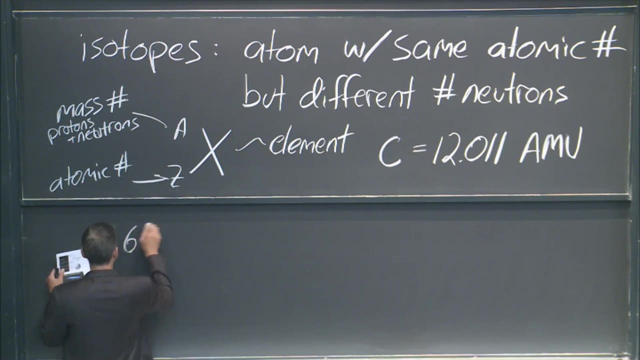 atoms are in this strip. How? Because I can again look up in the periodic table and find that in a gallium strip I know how many atoms I have. But if I say, well, 69 times x plus 71 times 1 minus x, 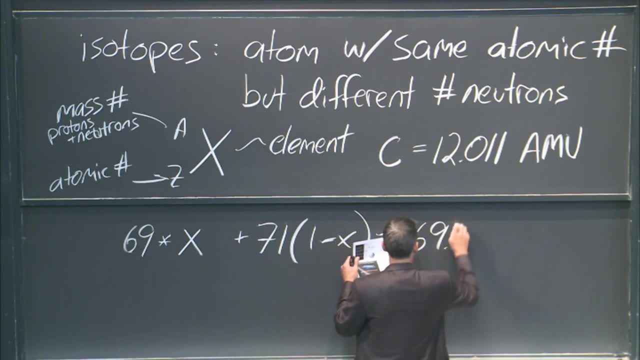 that's going to equal 69.723 amu. That's what's in the periodic table, But I now know that that's simply an average over all the right. So this would be like the fraction of 69 Ga, right.